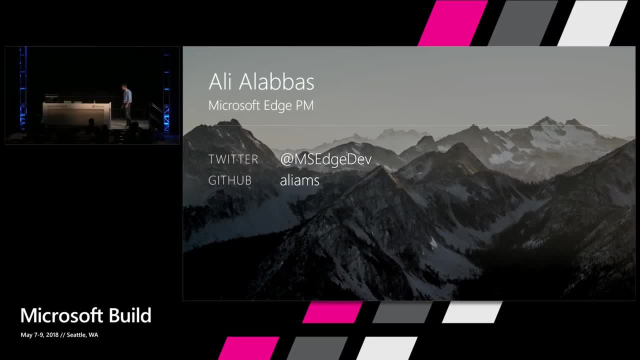 I mean, i'm still trying to recover from the last Experience. I will say, though, that i Remembered at that point that uber had a pwa at mUberCom That i was able to use, And so i immediately went over. 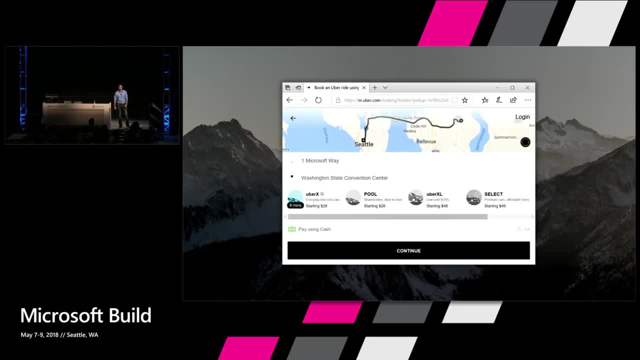 There and booked my trip over here. And in that moment, on that uber ride over here, i realized that This problem of not being able to get to the microsoft edge, Of network connectivity issues is not unique to me. Every day, hundreds of millions of people all around the world. 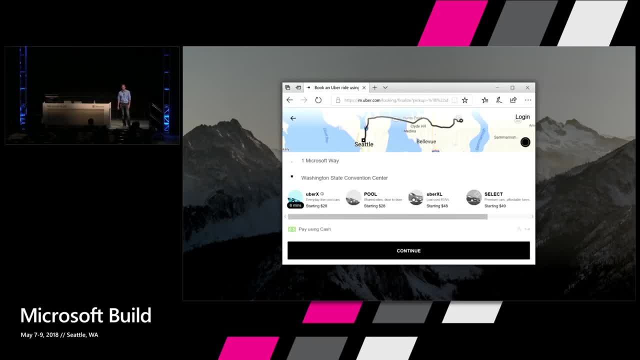 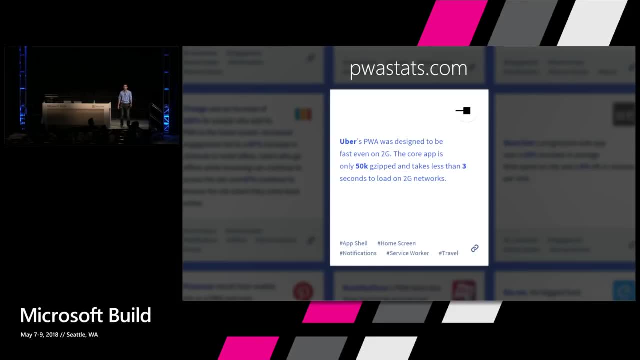 Are running into network connectivity issues in some Form or another. If you head on over to PwastatsCom, a community-driven list of statistics for pwas, You will see that there are many, many companies working Hard and investing in pwas so that they can not only improve. 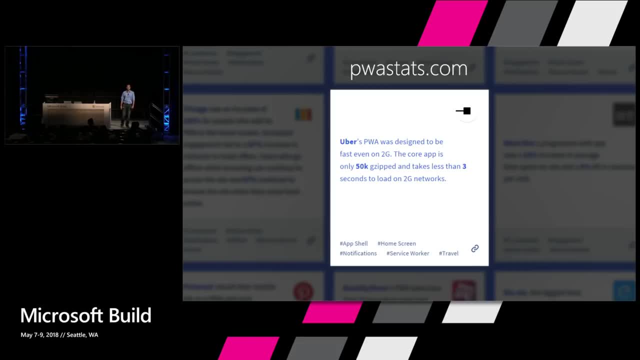 Their customers' experience, but also expand their network Opportunities on the web. Perhaps uber wouldn't have made Their cut from my ride on over here if i wasn't able to use MUberCom, But, more importantly, i had a way Of actually fulfilling that use case because they had that pwa. 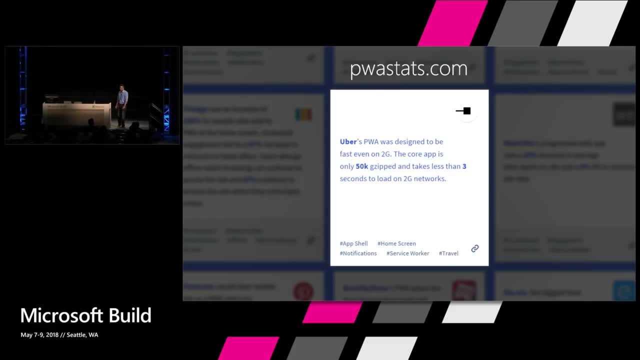 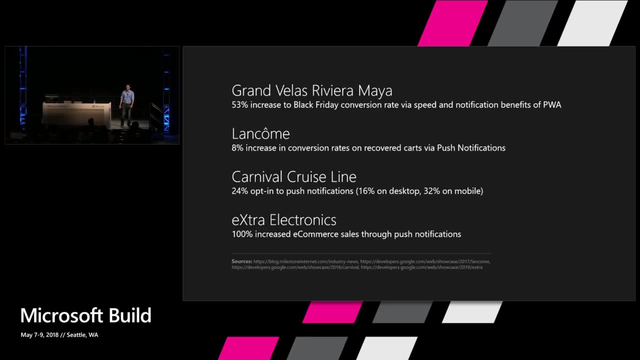 That they optimized for 2g connections. And of course there are other examples of this. For instance, grand vales, revier amaya, back in black Friday increased their conversion to pwasCom, Increased their conversion rates more than 50%. 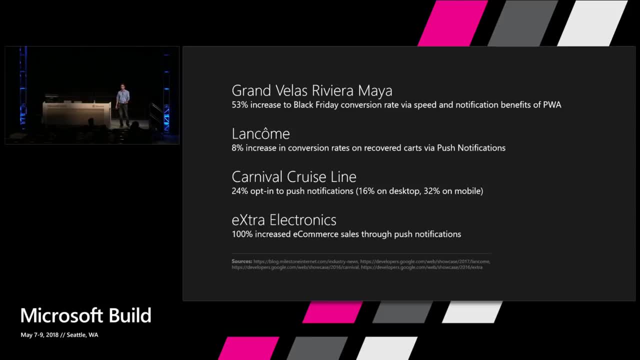 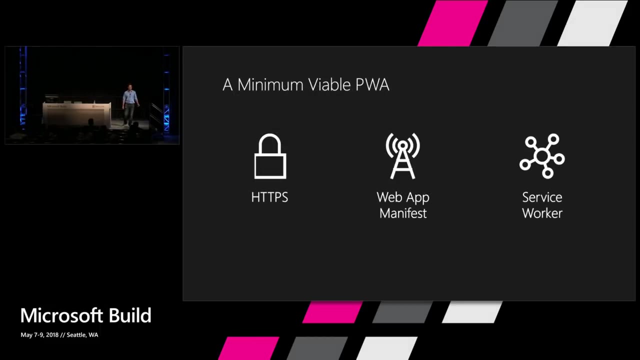 More than 50% due to the benefits of pwas and their Features, Specifically push notifications, And the reliability and poor network conditions improvements That they got from there. Now you may have seen jeff Burtoff's talk or maybe even aaron kustafson's talk. 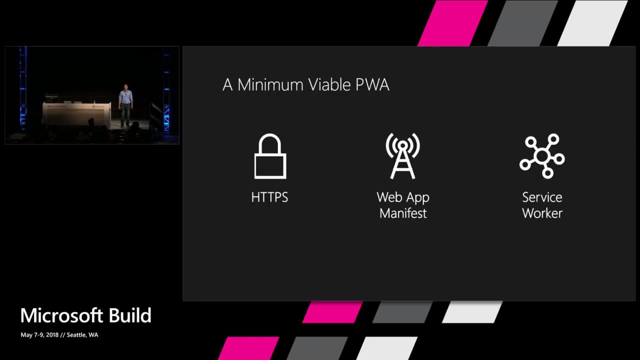 They had covered a little bit about pwas. Maybe you've seen this. Basically, a minimum viable pwas Requires that you use https, you have a web app manifest to Find and you have a service worker. And, as you know, there's more to it than that. 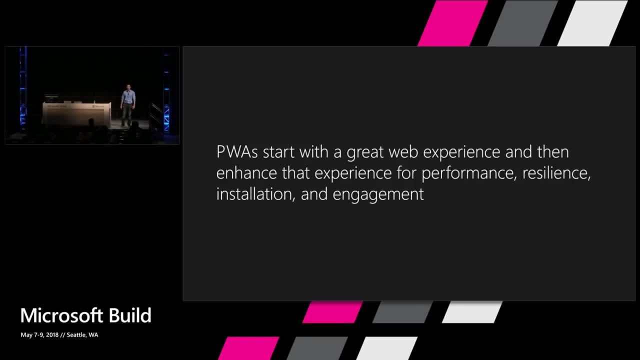 Pwas are about expanding the already great sites that you Guys are building, and applications, and enhancing their Performance, their resilience and the engagement of those applications. Today, that's what we're going to be talking about: How to build a pwas. that's going to be a little bit more. 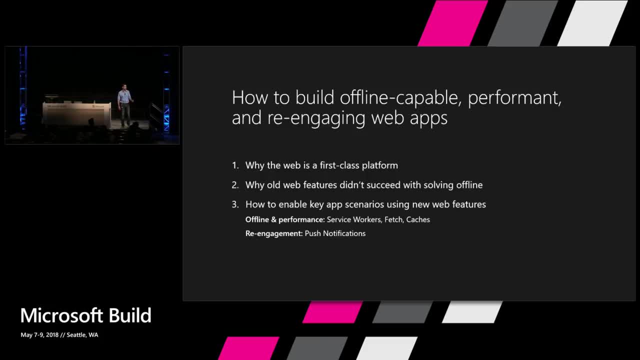 Simple How to build those offline Capable, performant and reengaging web applications. We'll first talk about why the web is a first-class platform And why some old web features that were there before were Supplanted by new ones that enabled some new scenarios. 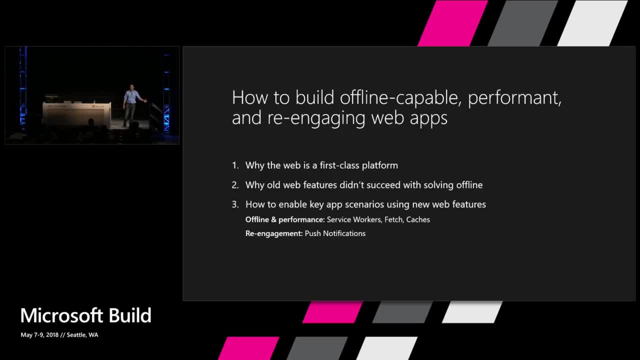 Specifically what you're probably here for Service workers and, of course, the other technologies that are Involved there, like fetch and caches and also push Notifications for reengaging those users. So you may have seen a list of pwa principles, as you might have. 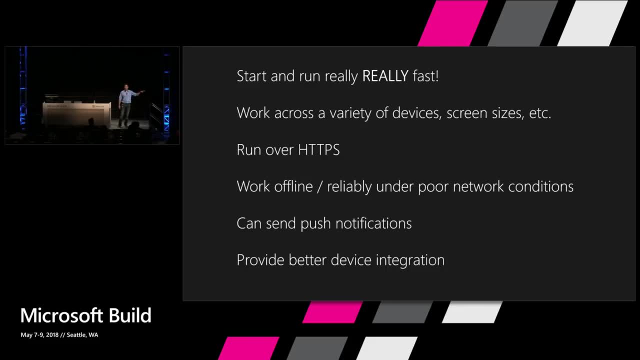 Called them. They may have seemed like this Or in another form, But basically we're going to Focus on two of those principles: Working offline and reliably Under poor network conditions and being able to send those push Notifications. For the first one today, if you. 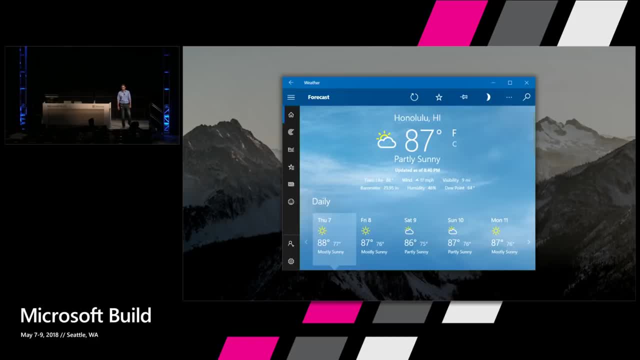 Take the weather app, for instance, in windows, you'll Notice that the app can work offline. It will give you an experience even if you're not connected. In fact, if you look closely underneath the temperature, It's going to tell you that it was last updated at some point. 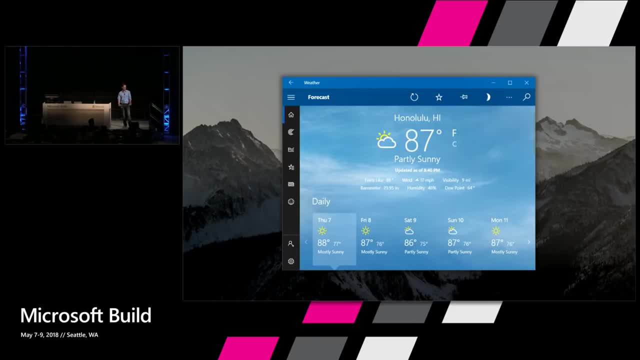 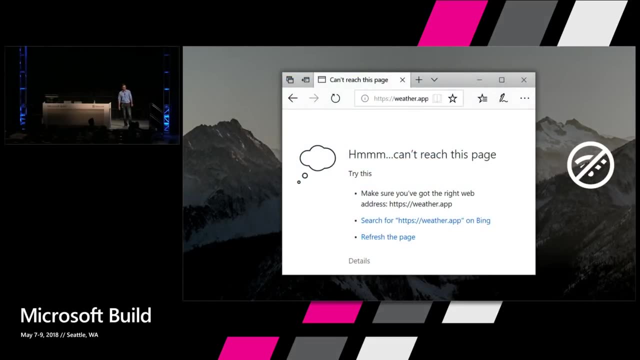 In time, And this is what native apps have Been doing for a very long time- They will launch to some Experience, even if you're not connected. And if you try this on the web, in a browser, for instance, You're going to get this A very frustrating you're. 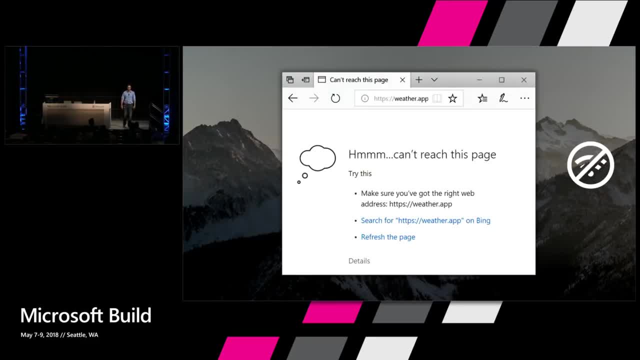 Offline page. That icon on the right indicates That you're offline. You don't have wi-fi And this you're going to get this. The problem is not unique to edge, or you know. obviously Other browsers as well have this problem. 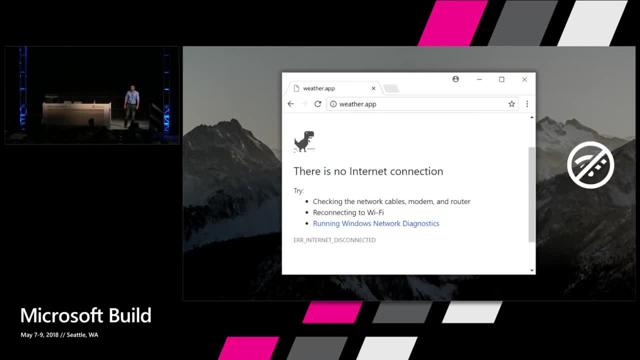 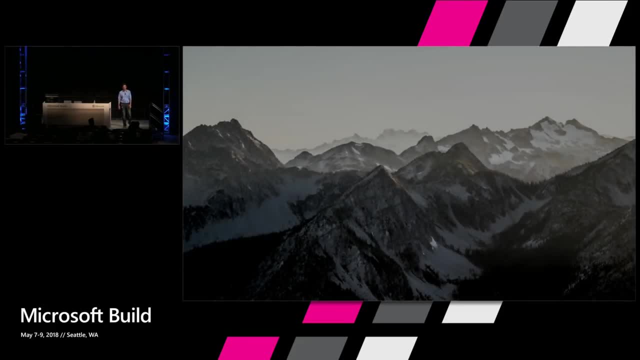 If you're not connected to the internet, you're not going to Get your experience. And then there's the other Aspect of sending notifications as well. Today, a native application is able to pop a toast that you Can then click and go back to the application, so you can. 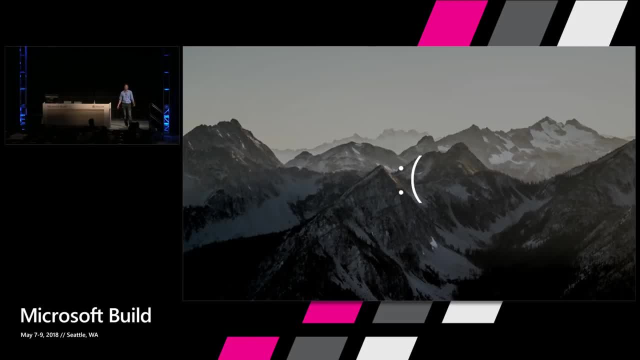 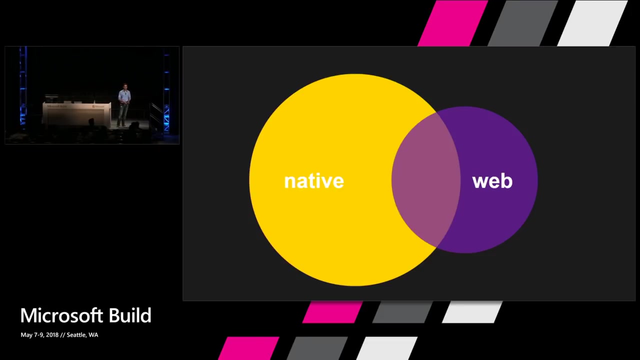 Reengage with it. With the web, however, you're Left stranded. There is no way to send a Notification if the browser is not open or if your web Application is not open. So, to start, it's important to Understand that there are a lot of gaps in the web. 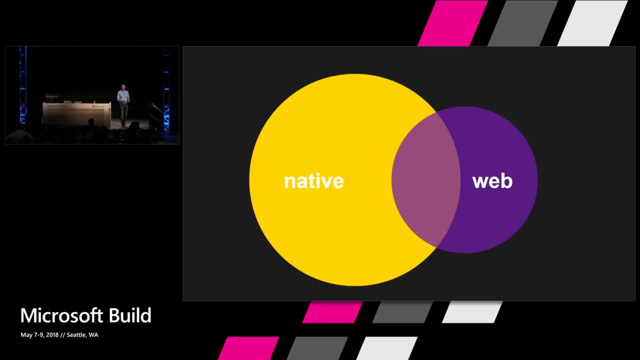 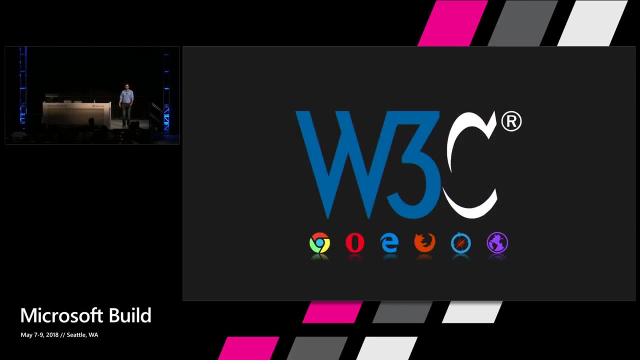 And when you compared it to what native apps were capable of Doing, it kind of looked like this. So a bunch of contributors and browser vendors took to the w3c, The worldwide web consortium, where we standardized web-based Technologies and capabilities and we came up with a way to 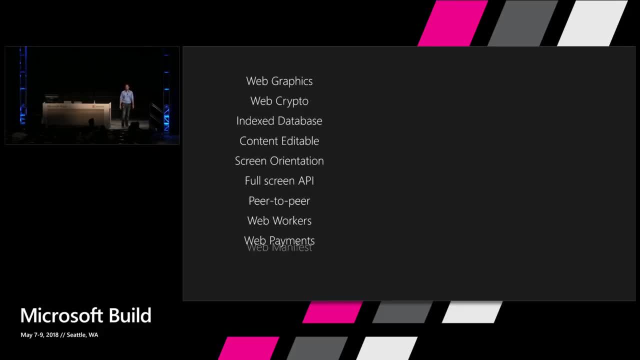 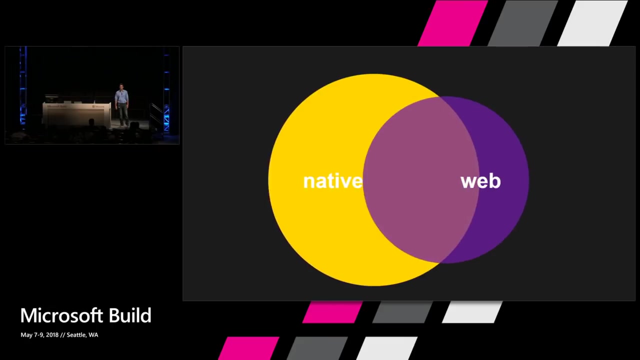 Fill some of these gaps And, as you know, history played Its way out, and we created a bunch of different apis that are Web-standard, along with the different vendors. This was a joint effort, And so we went from something That looked like this to something that looks a little. 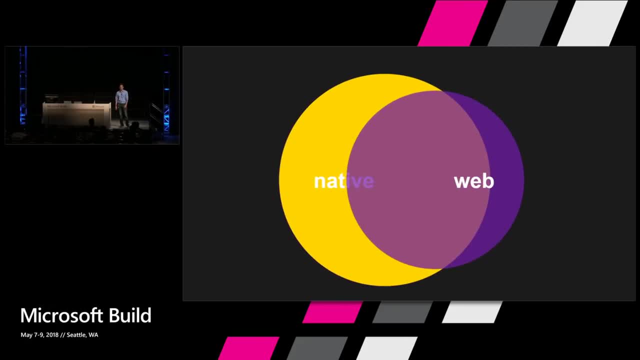 More like this. We're a lot more capable as the Web. now We can do a lot more, And to really understand where we are now, we're going to need To take you back in time so you can see what it kind of looked. 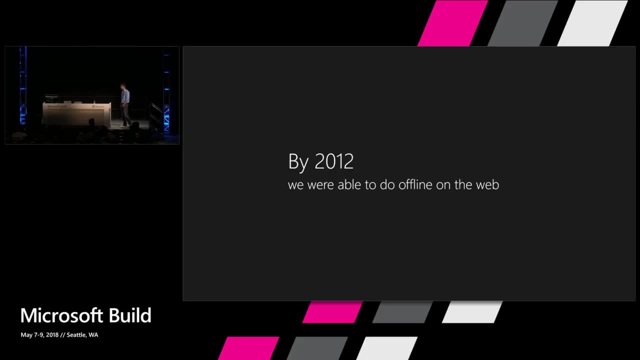 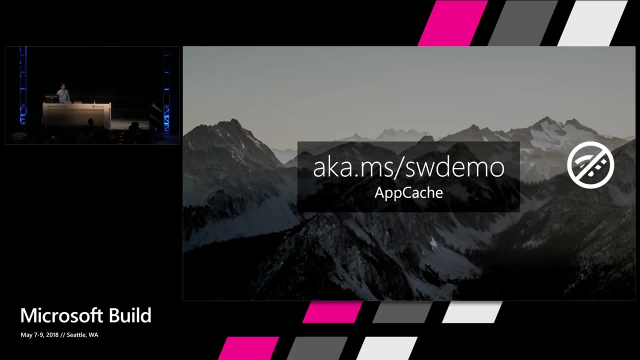 Like in 2012.. So we're going to go back to 2012 And take a look at something called application cache, And i have these demos. You can access them on akaMs Slash sw demo And we're going to do the first. 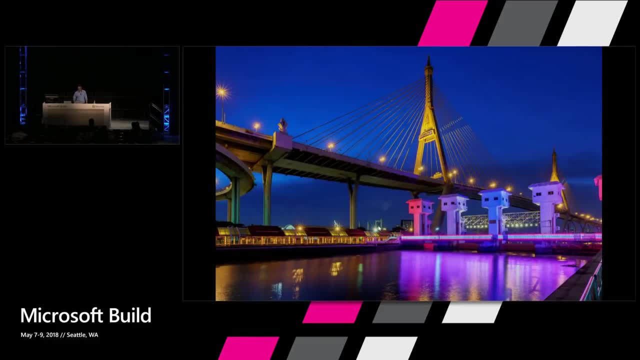 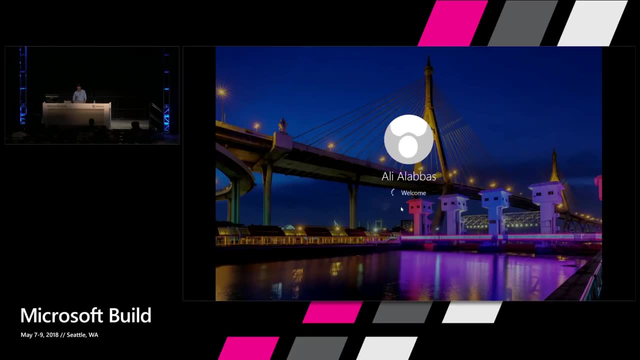 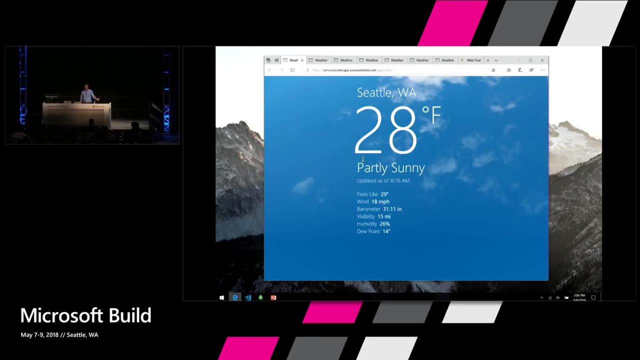 One on app cache. My computer fell asleep. Give it a sec, Okay. So here's a very awesome web Application that i built. It's basically a weather app. I rebuilt some parts of that weather application we saw before. Of course, it's telling me the weather. 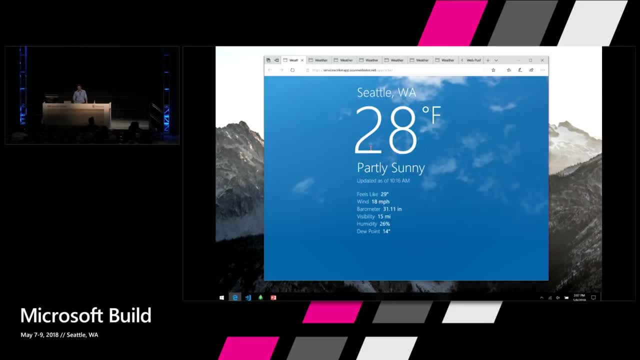 This is not accurate. As you know, it's pretty warm Outside right now. For those of you that only know Celsius, this is below freezing. Yeah, Okay. So if i refresh this page, you Know i'm getting that experience there. 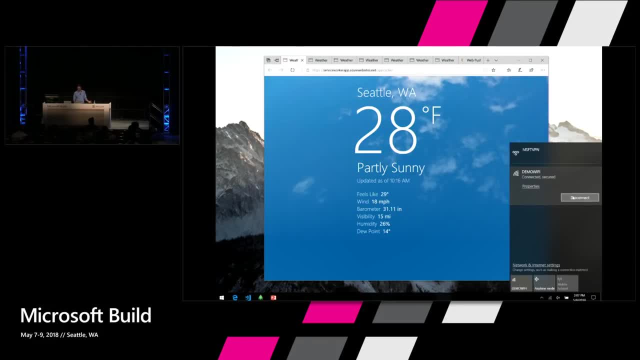 And if i disconnect from wi-fi- which is what i'm going to do Right now- and i refresh this page, you'll notice i still get An experience. So i'm still getting something. But you may have noticed, when i was connected i didn't get the 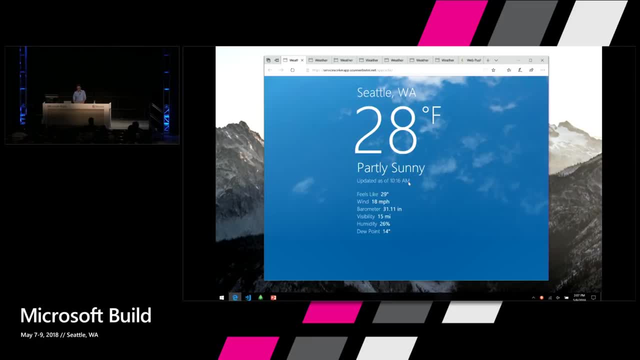 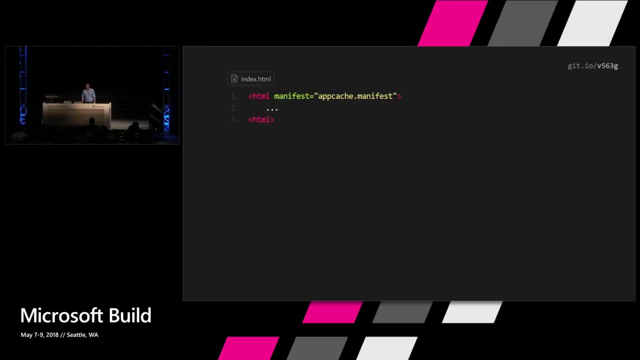 Updated weather information. In fact, it's telling me that it's Still updated as of 1016 aM This morning. So there i am, connected again And it kind of looks like it's Busted. So this is how you would have. 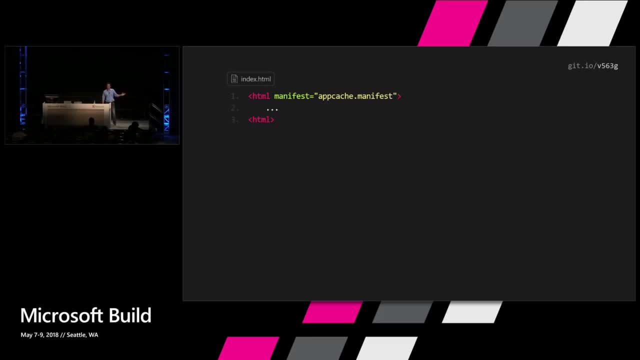 Used application cache. You basically had your html page That you would then identify your manifest, your manifest File, that's going to tell you what things to cache, And you're going to do that by saying manifest equals app cache, And then you're going to specify the actual manifest itself. 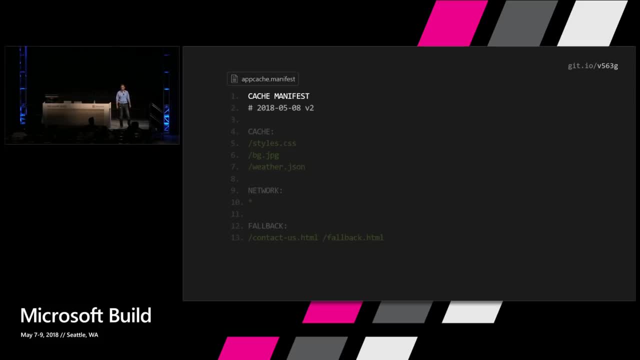 The first thing you're going to do is you're going to say cache Manifest and here i have a comment saying when it was last Updated, and then i'm going to, under the cache heading, say Which resources i want cached. I'm telling: app cache these are. 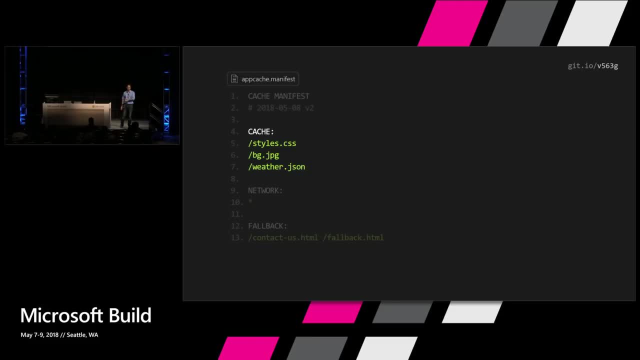 The resources that if you make a request, pull them out of the App cache, Don't go to the network And, of course, if we are connected to the internet, for Any other request that is not defined in those previous Rules, go to the network for those requests. 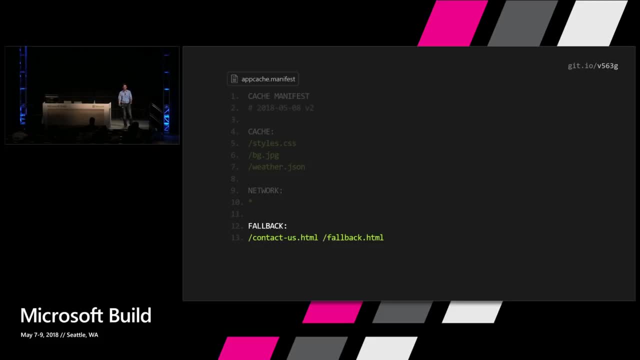 That's what this star wild card is, And then i can also specify a Fallback. For example, if you have an Experience that actually requires an ever connection, Like maybe a contact us page, i can have a fallback experience For that. So it wasn't really quite the. 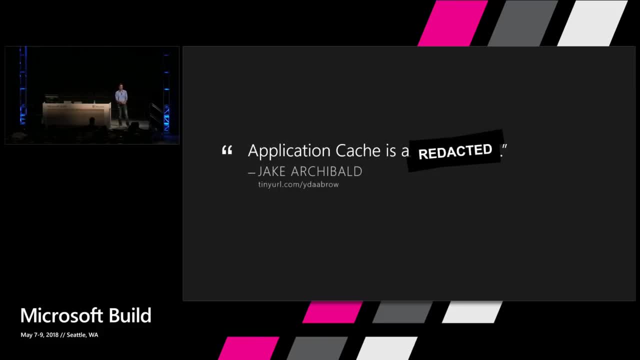 Silver bullet we were looking for. Jake archibald, a tech evangelist, had some choice words About application cache. If you're interested in knowing What those words were, feel free to follow that link And then you're going to go to the network. 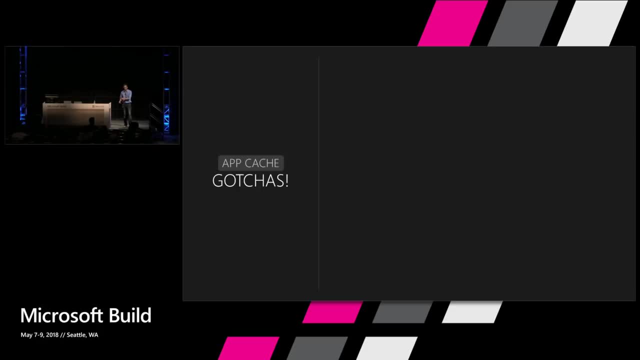 And to kind of give you an idea of what those were. you kind of Saw it right there, but you basically had to update the Manifest file if you wanted to change anything. That's very important. So you notice that comment i had Inside of the manifest. I would need to update it maybe. 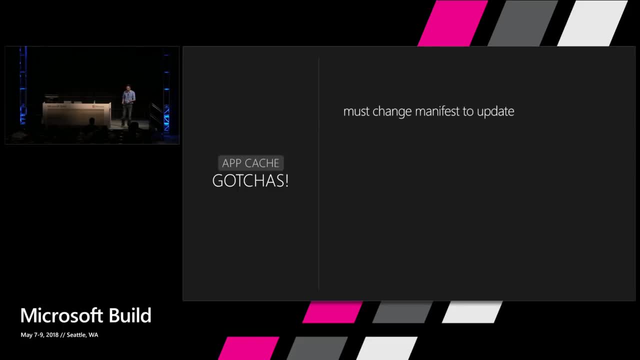 Just a little bit and then it would allow it to change. So you also had the different manifest files. If you had them become stale for some reason. if you set a far Future cache header, you're basically hosed, in the sense That you can't update your experience. 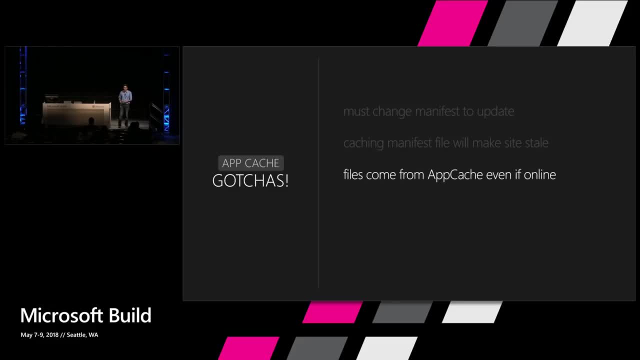 So you have to be careful of that as well. The files come from the app cache, even if you're online. Did you guys notice how, when i refreshed the page, even when i Was online, the files, the actual weather data, did not update? 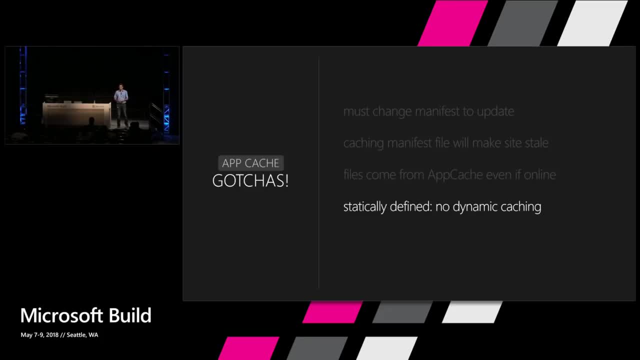 So that's a problem too. All of the rules inside the app Cache are statically defined. There's no form of dynamic Change And, quite frankly, it's very Magical and difficult to debug. The browser is doing a lot of Stuff on your behalf as the web developer and you really can't. 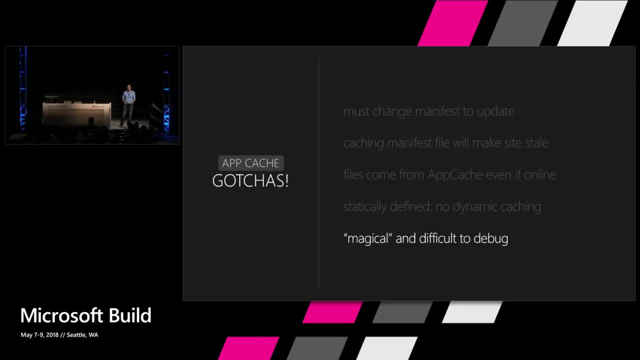 Tell what it's doing. It's not like javascript, where You can set a break point and see what's happening. In essence, you have no control. So app cache is useful. It had its time and place, But we can do better than that. 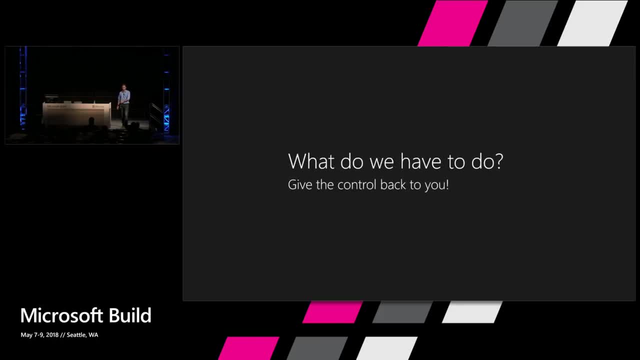 So to do that, to give you back control, you have to have a First look back at exactly what causes the problems in app cache, Which is from the very first point where we have the requests Happening in the app cache. we have to redefine that. 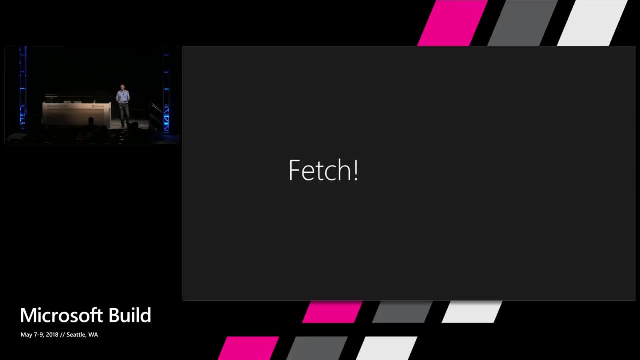 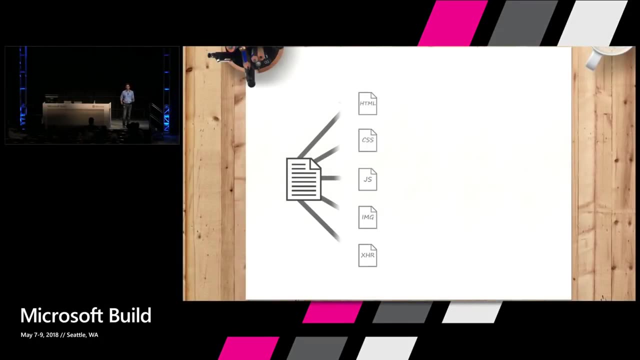 We have to unify that concept, And so we've introduced the Concept of fetch fetching. So on a normal web page, you Have a bunch of resources that are happening, that are being Downloaded. So you have your html, your Javascript, css, etc. You have a bunch of resources that. 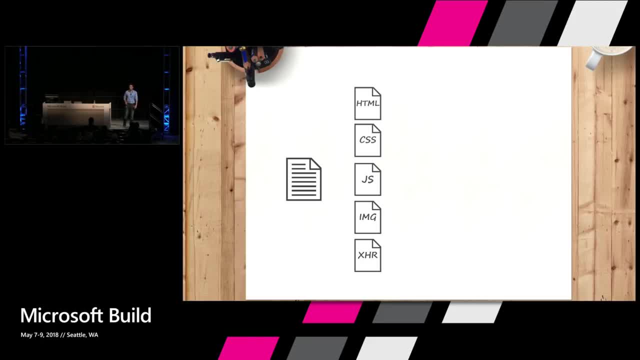 Have html requests, images, whatever, xhr html request, And then they normally go to the network if there's no http Cache for that item. With this new concept of fetch Instead of going to the network directly, we've basically Abstracted that concept, so now they go through this fetch. 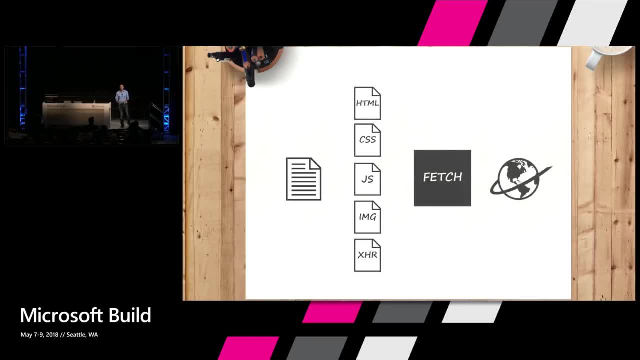 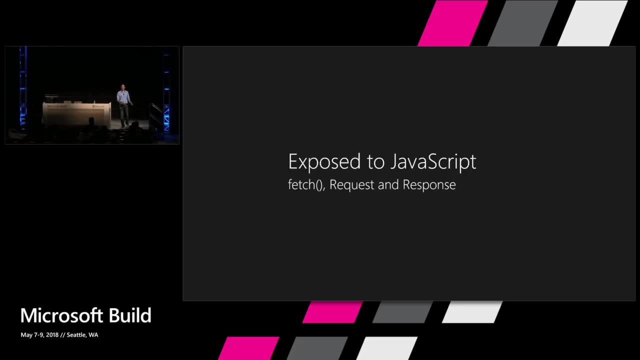 Layer this fetch abstraction that then can go to the network. So there's some interesting side effects because of this, One of which is we can expose these concepts to javascript, Such as the fetch method, so that you can invoke fetching Programmatically, and also the primitives for request and response. 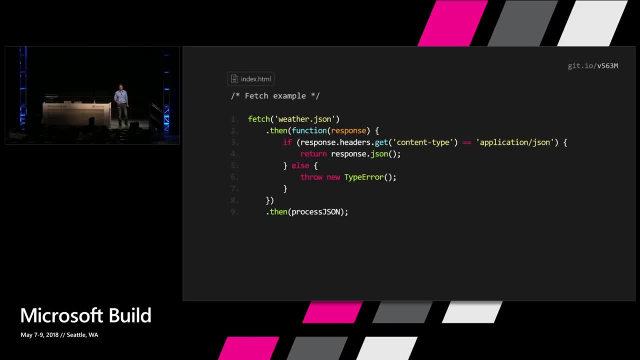 So this is what a fetch might look like if you were to write It programmatically. So first you would make the Fetch to weatherJson And then we're going to use, Because this is going to return a promise if you've never used. 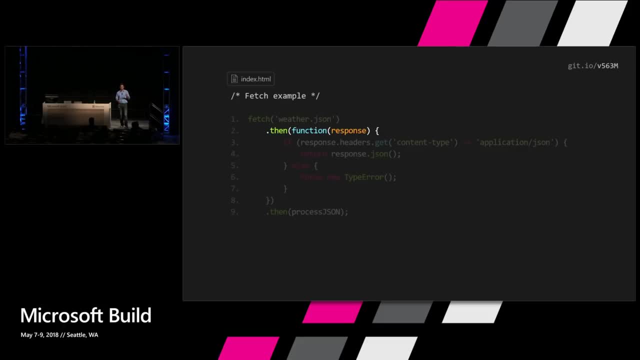 Promises before. just know that if you have a promise that you Have, if you have something that's returning a promise, you Can use dot then, which will then let you do something Asynchronously after the promise has finished. So it's a way of doing asynchronous programming in this. 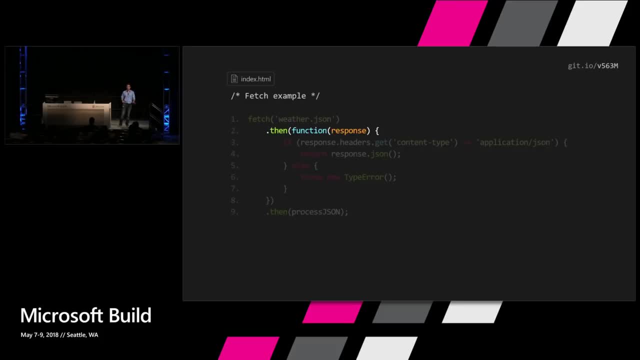 Sense, And most of these concepts are Going to be using promises. so if you're not familiar with them, I do encourage you to read up on them. So from that point we can check if what the we can actually get The headers object and then see. we can see what the content type. 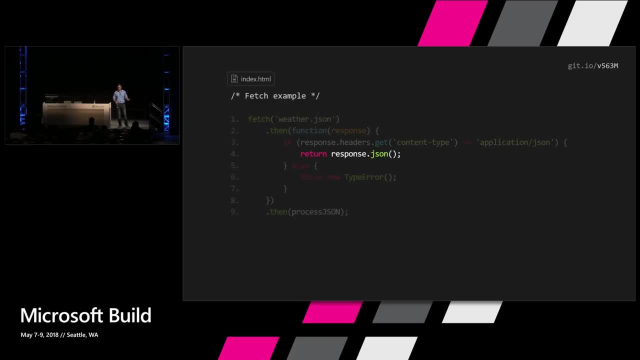 Is, And in this case it's application Slash json. We're going to get the json From that file, And the way that we do that is Use the dot json helper method, which will help get back the Json data For comparison. this is what it. 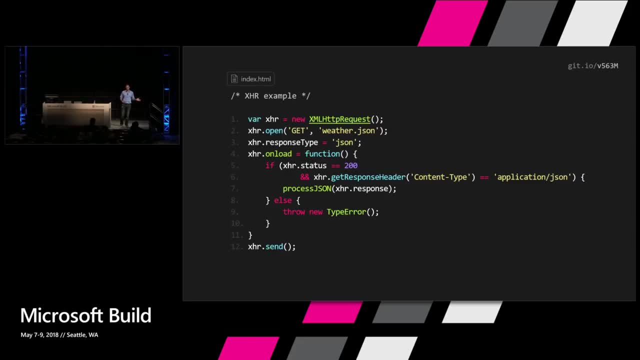 Would look like if you were to do the same thing in xml http Request, So it gets you the same results, Sort of, but what you're getting is a lot more code that you have To write, and it doesn't look as pretty as fetch. 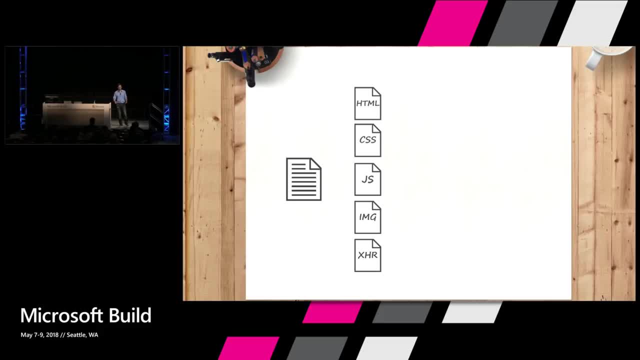 So back to where we were. You get your requests, your Subresource requests, for all the files. We're going to the fetch pipeline that we've now built And now, at this point, you're wondering: how do we give that Control back to web developers? how do we give it back to you? 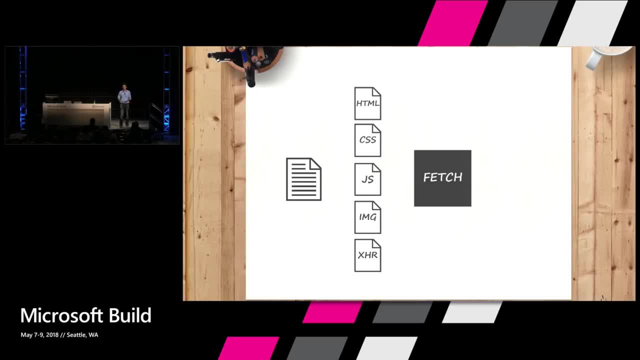 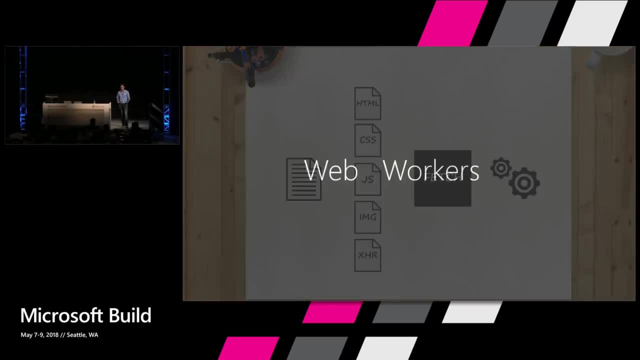 So you might be thinking of maybe a worker- javascript worker Type thing that maybe could take that request and do something With it, And in fact that's what it's Going to do. So you may have heard of web Workers, but you may not have heard of web workers. 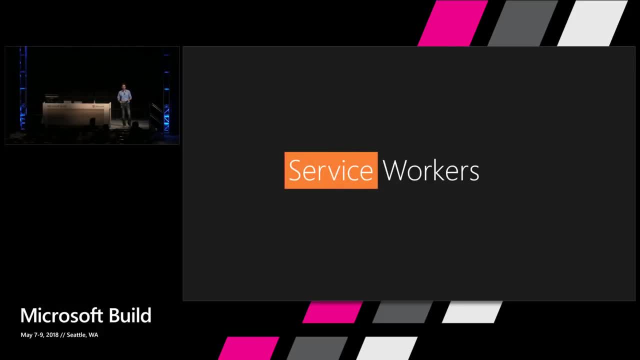 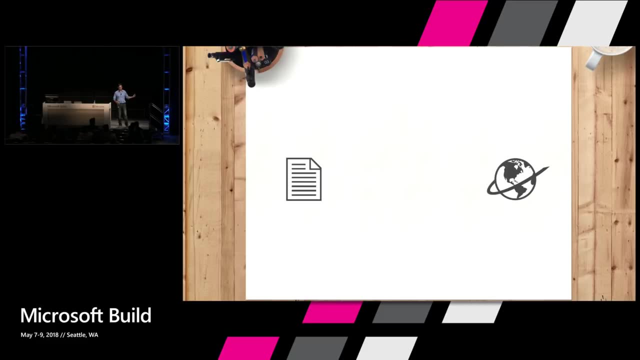 But this is even better. This is a service worker. So this is how a service worker works. You have your page and it usually just goes to the Network. It's getting its- you know- Requests out there and then gets responses back. 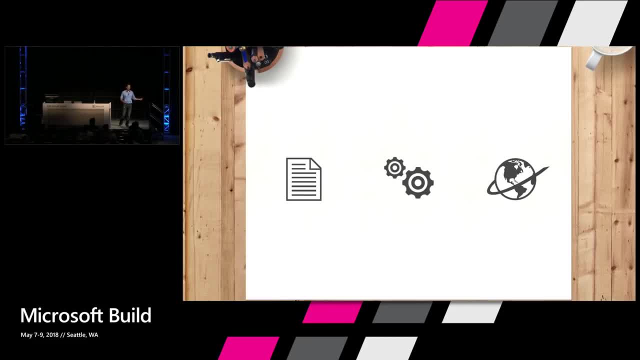 When a service worker is in play. instead, the service Worker gets to intercept that traffic and then return back to The page any of its responses that it wants. So you're probably wondering: this is all well and good, but How is this supported across the different browsers? 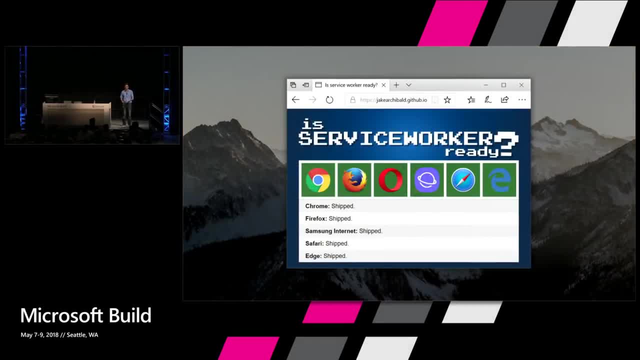 Do other browsers have service workers And i'm happy to report that we now will do have this support As of the april update that came out. for windows, service workers Are now on microsoft edge and for progressive web apps, for web Applications, if you're going to use them. 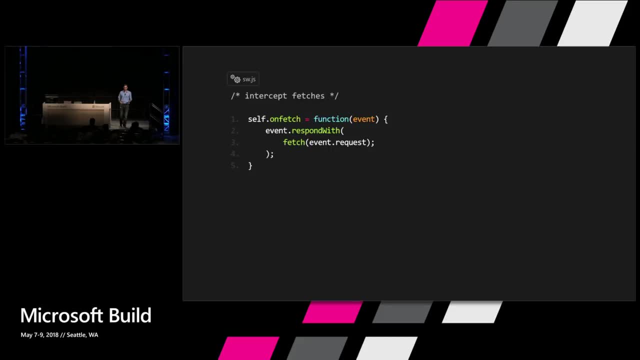 So to use the service worker to intercept fetch traffic, you Would basically have to write in the service worker what the Service worker- a fetch event- handler. So we're going to do self dot on fetch. You can also do self dot, add event listener- fetch, if you. 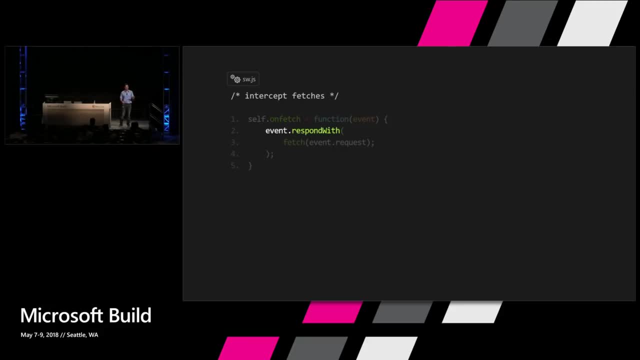 Want to do that as well, And then from there we're going To use event dot respond, with, which will give us a special Capability to respond back to the page by passing in a promise That either gives us a response object: remember when we were? 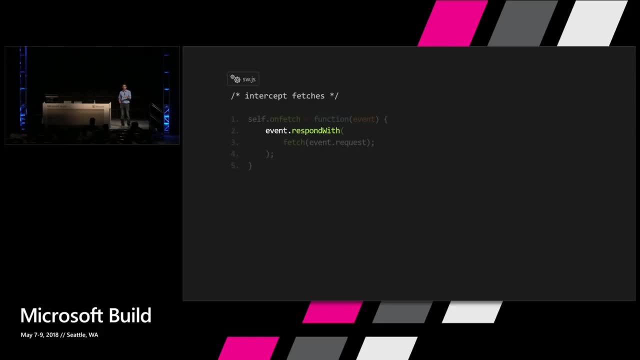 Talking about fetch, the response objects or we can Pass back a response itself. In this case, we're going to do What's called a pass-through. So we're going to do a pass Through. We're just going to do a Fetch with that request that we got and we're going to let that. 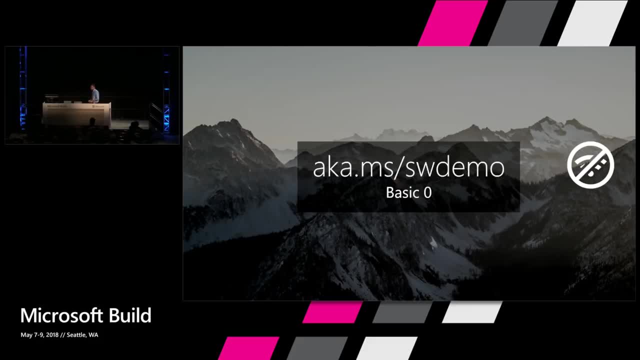 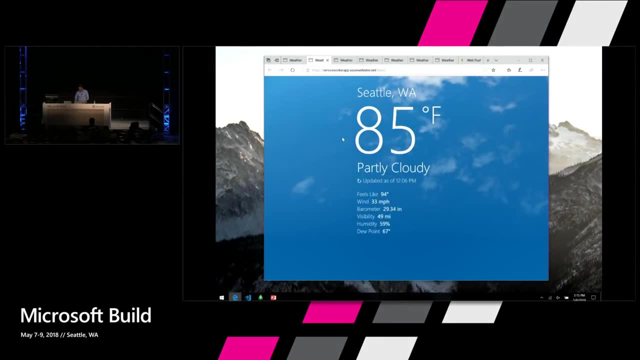 Go through. So we're going to see another Demo here of what that looks like once we've just set it up To do just that. So here we have that page again. This time it's using a service Worker, It's not using app cache. 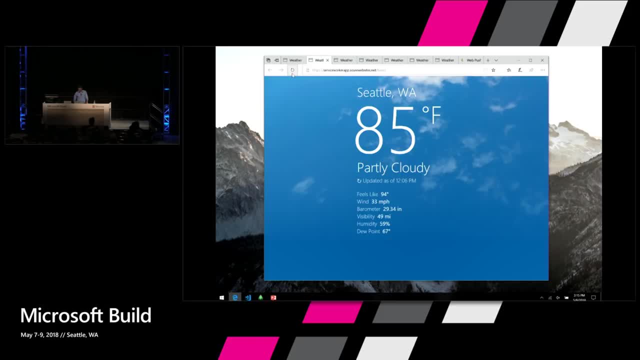 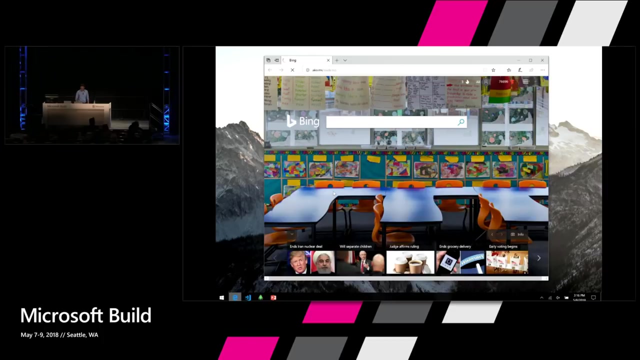 So you can tell that i'm going to refresh this page. Maybe i Let's see. It looks like it doesn't like me reconnecting, disconnecting From wi-fi. All right, There we go. So, by the way, you guys can go. 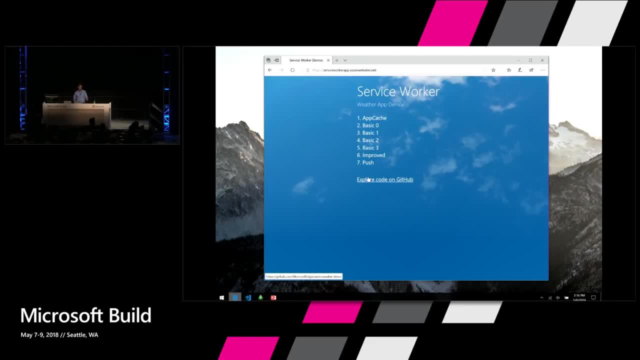 To this page, and then you can see all these demos as well And also explore the code on github, if you like. So i'm going to go to that sample page that i was just Talking about. So there we are. It's telling me that this is updated as of 316 pM. 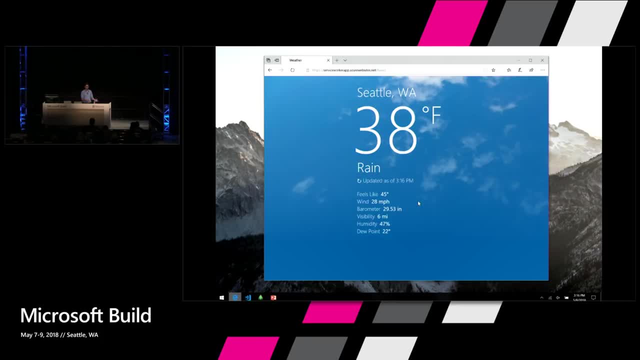 By the way, this is giving me nonsensical data on purpose, so You can see that something is happening. Obviously, 38 degrees again is not the temperature we're Inside. So what i'm going to do now is I'm going to disconnect it and i'm going to try this again. 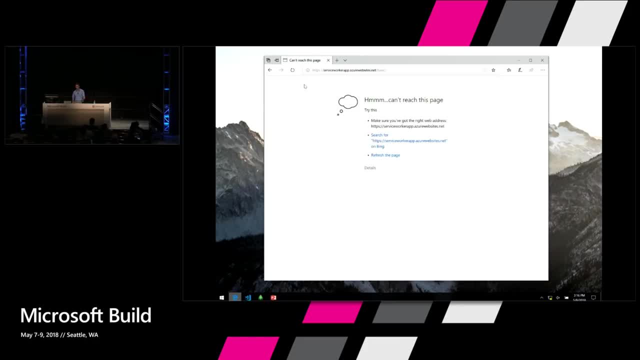 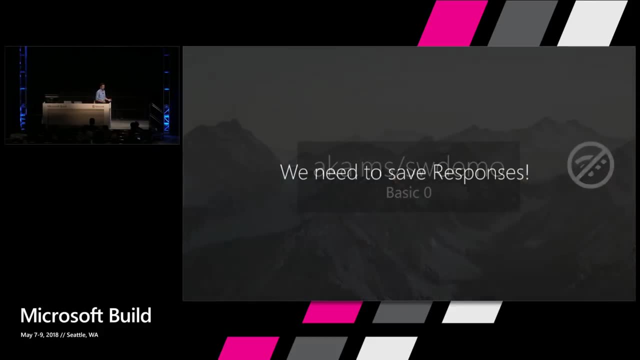 And what happened here. well, if you noticed, we Actually didn't really do anything but pass it through to The network. In fact, what we really need to Be doing is we need to save those responses so that we can Do something with those saved responses and then give it a. 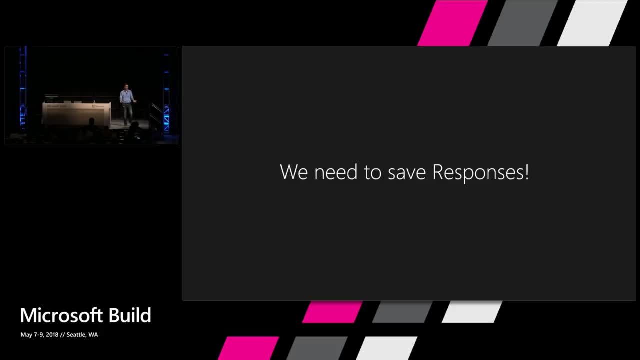 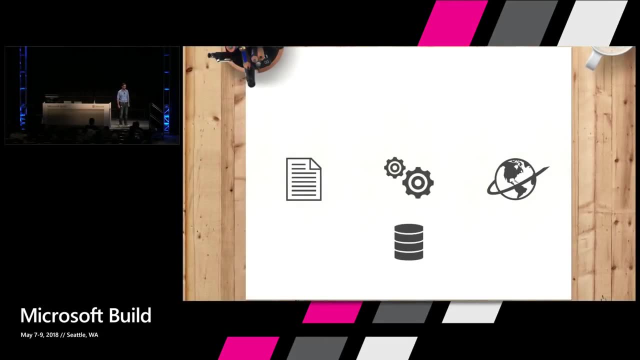 Back to the page, Because when i go offline They're not there. I need to put them somewhere. That's where we introduce the cache apis. So again back to that diagram of making the request to the Service worker. except this time we'll be going to the 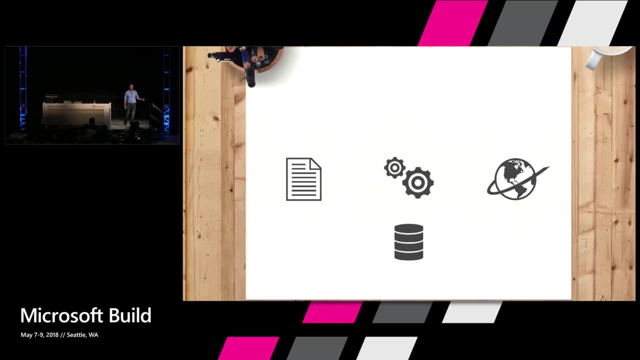 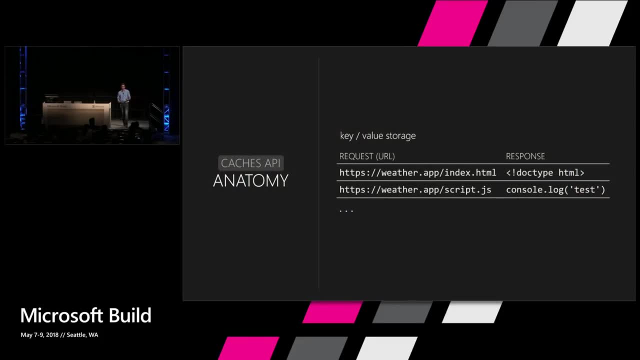 Caches, using these new cache apis to go back to the page With something that we've saved, So to give you a bit of a sense Of what those caches look like. they're basically a key value Storage mechanism Where the key is the request. 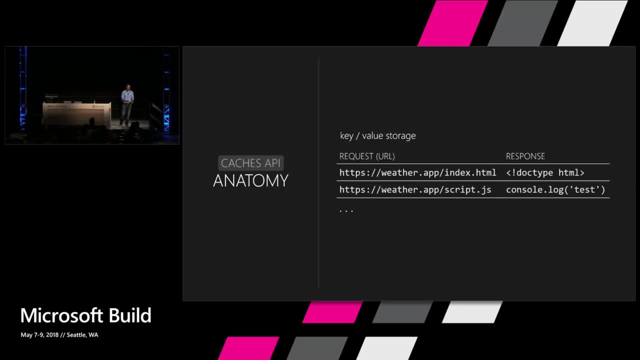 And the value is the response, The request object and the Response object back from when we were talking about fetch. For simplification, you can think of the request as being Just the url and then the actual content of the response. for the Response. So you're probably wondering now. 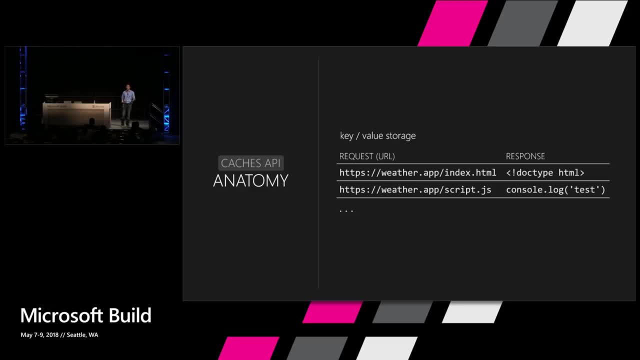 We've introduced a new concept, a new storage mechanism to the Web cache: apis. What about index db? You may have heard of index db. You may have heard of index db. A good way to think about this is if you have url addressable. 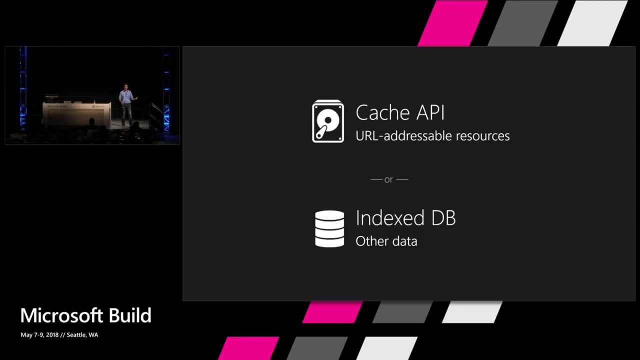 Content like a request and response pair. put it in the Cache api. Anything else? continue to use Index database. Put it there. I just want to make a quick side note about quotas in microsoft Edge. So, as you know, depending on the 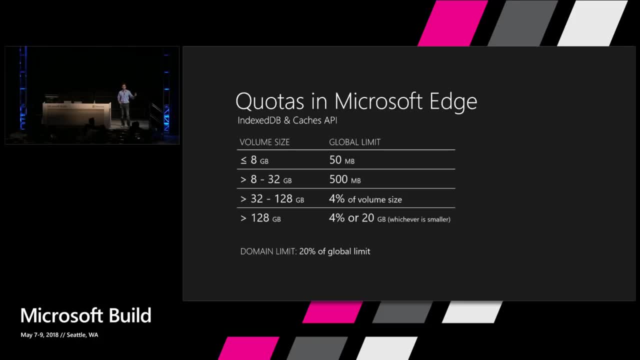 Size of your volume on the device that you're on, you're Going to have a different set of quotas for both index db and The caches- the new caches, api- And depending on that, you're Going to have a different total limit And on that total limit you'll also have, per domain, 20% of. 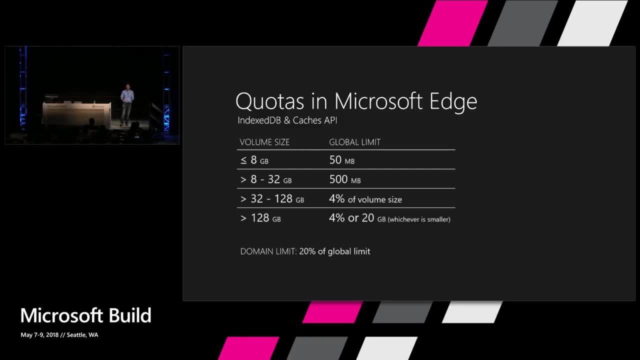 That total limit. So something to keep in mind as You build your web applications. It is also worth noting that if You have a pwa, something that gets installed to the user's System, to the device, then they won't be subjected to these limits. 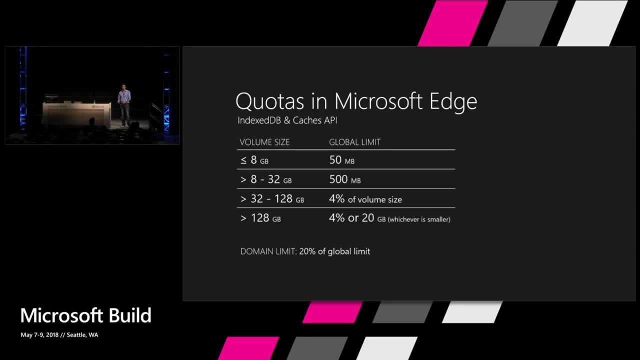 They'll be just like any other application on your system, where They can take up the space that they need to. Okay, So now we're in business, We can actually save those responses so that we can use Them later. All right, So we're going to register that service worker, which is the. 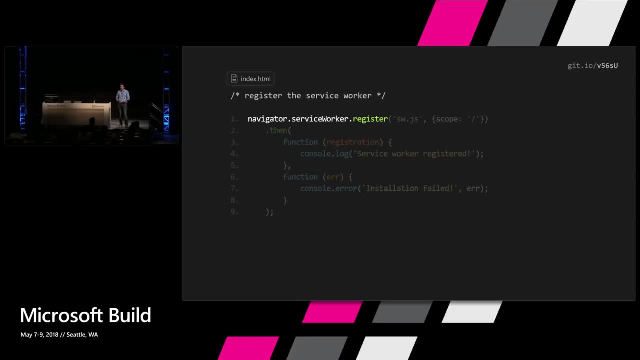 First step before we even use it. So first we're going to do NavigatorServiceworkerRegister. I've had a nickel for every time. i wrote that. Just memorize it: NavigatorServiceworkerRegister. Okay, Then we're going to pass in the 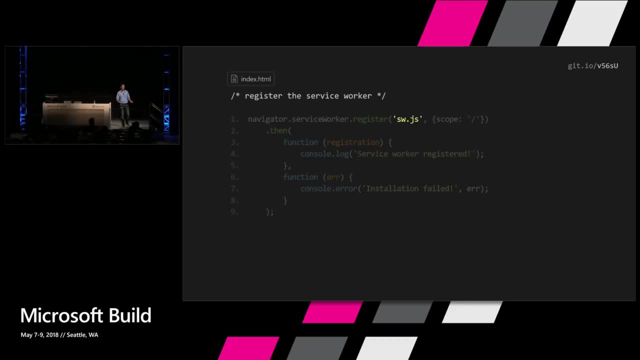 File that we want to register. It's just a javascript file. Here we're calling it swJs, And then we're going to pass in The file And then we're going to specify Scope. In this case, we're just going. 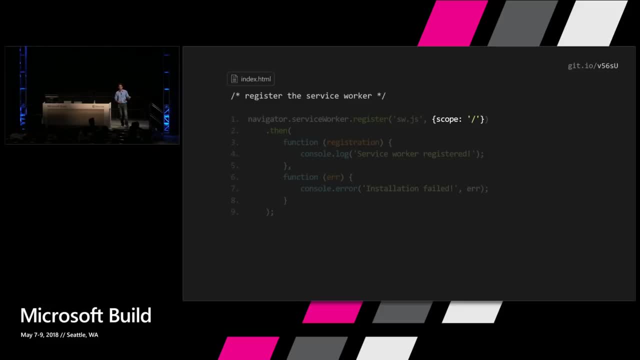 To use the default as the root. It's worth noting that the Service worker, where it is in the directory structure, will Basically need to be in the same scope that you're going to define. And again, we're using promises here. 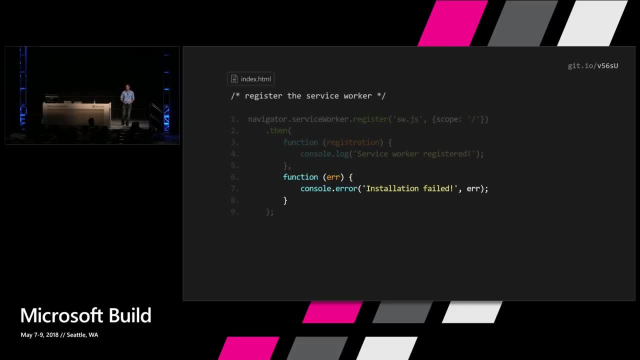 So if that succeeds, we can do something with that, And if it fails, we can catch that response and say that Installation fails. So some quick notes before we Move on and talk a little bit about this, Talking about what service workers, how to use them and 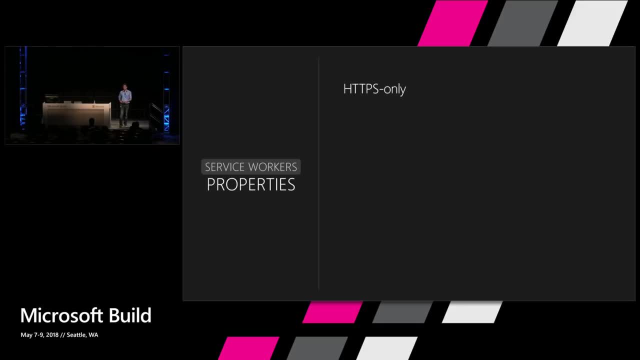 How they work. Some things to keep in mind. They're https only, So that means your site needs To be hosted on https for security reasons. You can do it on localhost as well. Browsers will work if you use localhost. You don't get any dom access inside of a service worker. 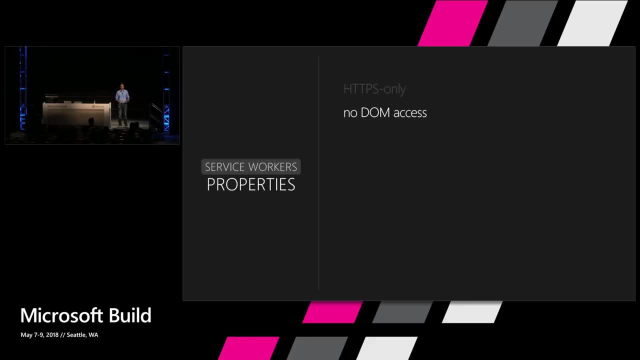 The same way that you don't have dom access in a web worker. So if you wanted to do something on your page, you're going to Have to do something like post message from your service Worker back to the page so that it can then do something like. 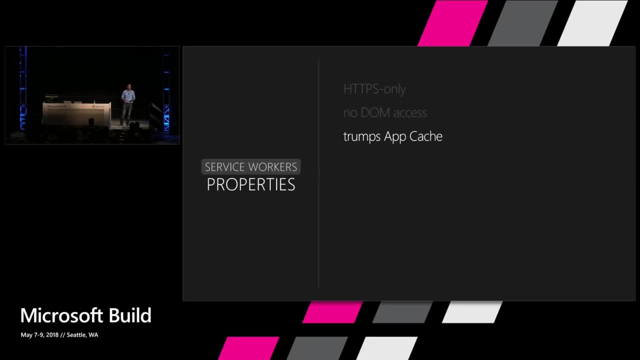 Update the page. If you have app cache specified For a page that also specifies a service worker, the service Worker takes precedence. In fact, if you have the service Worker, app cache just doesn't work. This might be a way that you would provide that progressive. 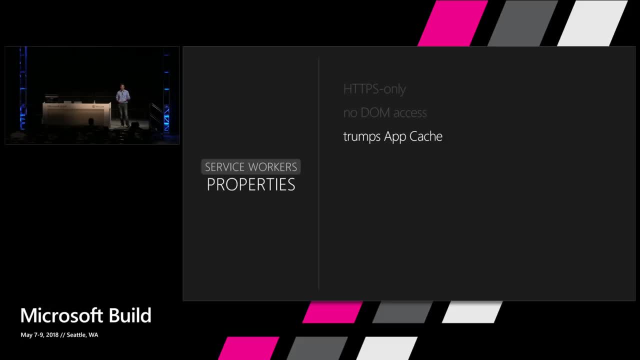 Enhancement that you may have been hearing. So if you have a user that doesn't have a service worker Browser, they could still take advantage of app cache, which Has been there for a while now. The original script at swJs Can't be on a content distribution network. 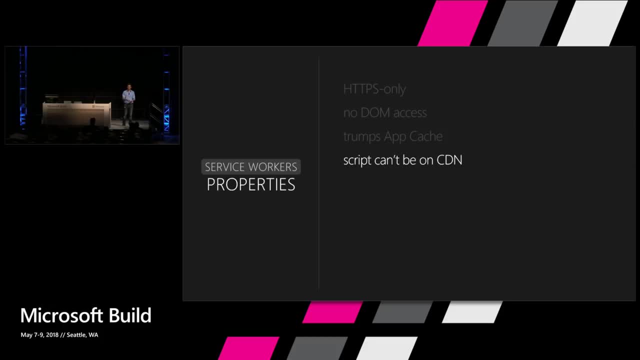 You can import scripts from a cdn, but that original script Can't be on a cdn itself. It has to be on the same domain. It has to be served from the same domain as your page. It's also important to note that they can be terminated at any. 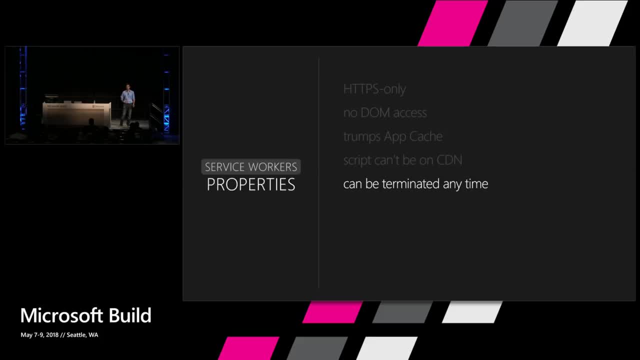 Time A service worker is at the mercy Of the web browser. If you have a service worker that Has a web browser or the operating system- for instance, If you have battery or storage pressure and it's trying to do Stuff- then they can be terminated the same way that. 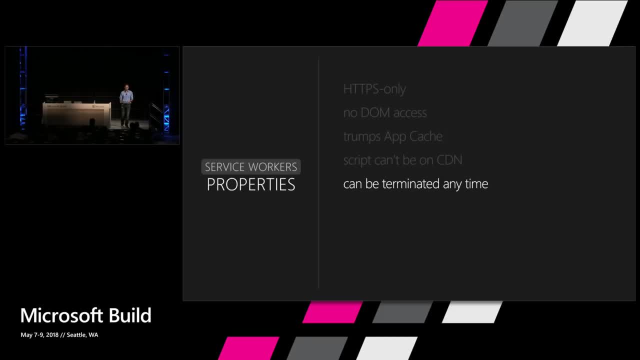 Any other process can be terminated Now. normally this won't affect you, but it's important to keep In mind so that you know that your service worker only has so Long to do what it needs to do inside of the events that it's Going to handle. And i'll talk a little more. 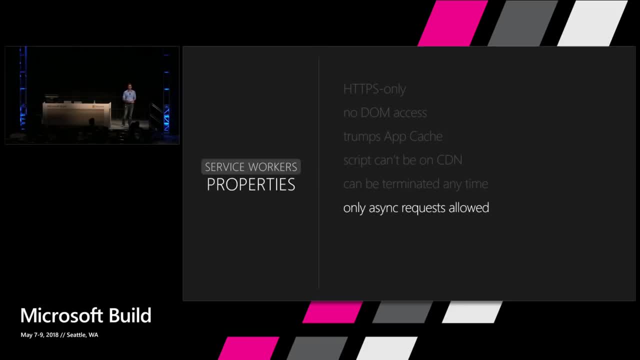 About that in a bit. Only async requests are allowed In a service worker, So there's nothing like a Synchronous xhr going on over here. okay, Only fetches which are asynchronous by nature, And you can't use local storage either. 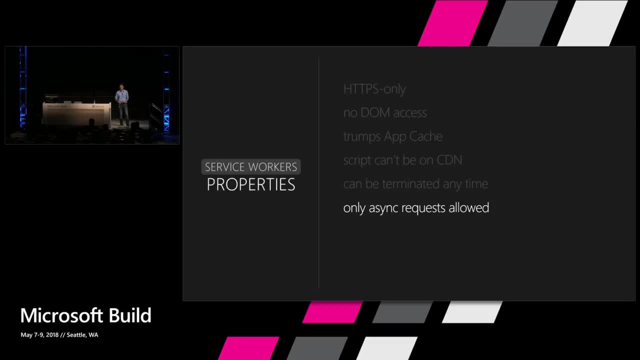 You have to use index db, which is also asynchronous, And the cache is api. They execute separately from the Page. So if you have a page that Normally executes javascript, you also have a service worker That's executing separately, And this is important to note. 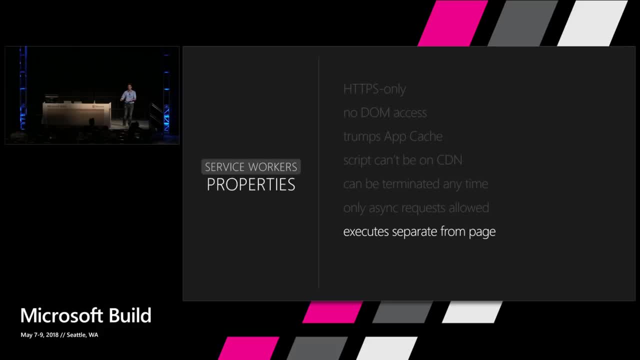 Because their execution contexts are not tied. You don't get the same globals, for instance, from your page as You do on your service worker, The same way that you don't get That for a web worker, And we saw a little bit about. 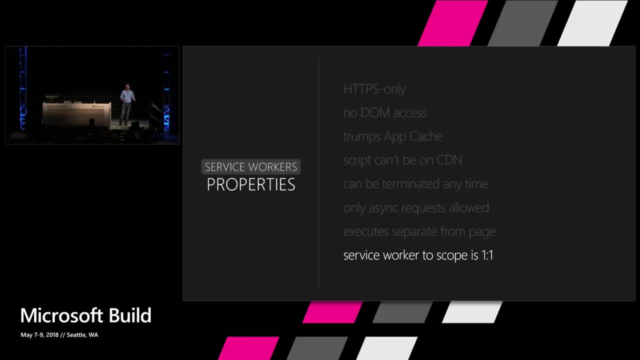 That scope earlier. It's important to note that the Scope to service worker mapping is one-to-one, Meaning that if you have a service worker that is going to Be registered on the same scope again, it will update that Service worker so that you can get the new version for that. 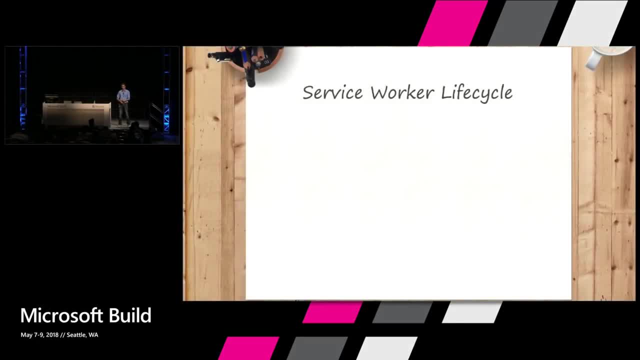 Service worker. All right, So now that we kind of got through some of the basics, We're going to go through the life cycle of a service worker, Which is important to know Because you may be wondering: Okay, you have this service worker, How do i maintain it? 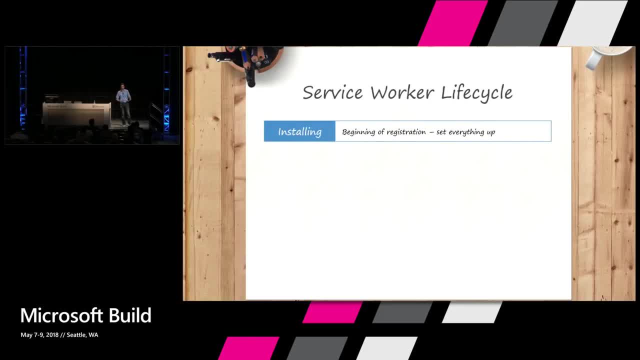 How do i update it? well, we've got to start with How exactly it goes through its life cycle. So the first step of its life cycle is that it goes through The installing phase. This is the beginning of Everything. This is when the registration. 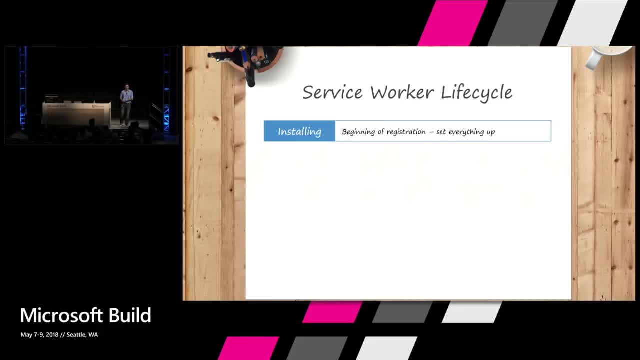 Happens and where we set everything up for the service Worker, And i'm going to show you what You do there in a bit. Then we go to the installed Phase, So it goes from installing to Installed. At this point the setup is. 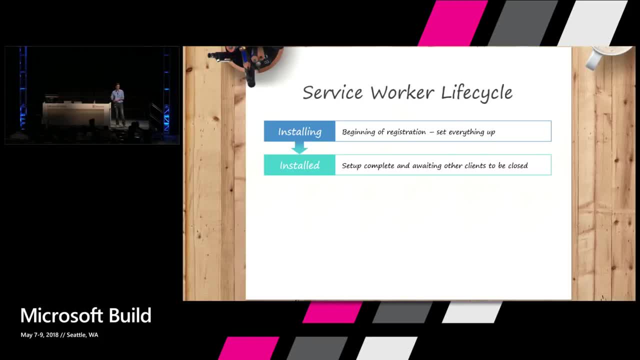 Complete and we're waiting for anything that is using the Service worker, where using means that if a page is trying To use a service worker to get responses from it's going to Wait for all of those pages to be closed, for instance. 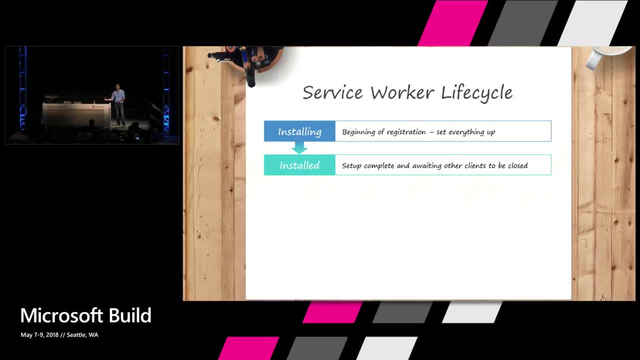 All those tabs. So if you had like three tabs That were using one service worker, those three tabs would Be closed before you can actually be installed. From that point you go to the activating phase. So at this point no clients are controlled. 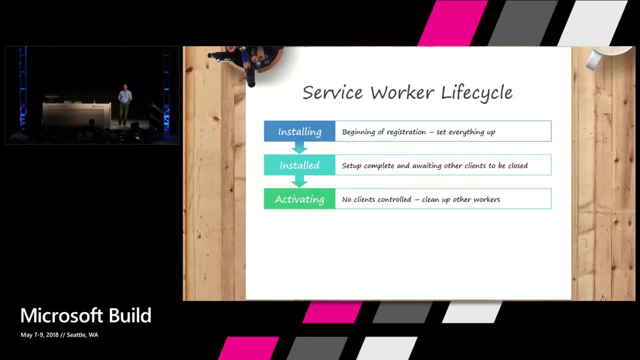 So you've killed off all those browser tabs, for instance, or The app, if it's an app, And what we might want to do Here is clean up any older versions of that service worker, For instance, our caches- I'm going to show you how to do. 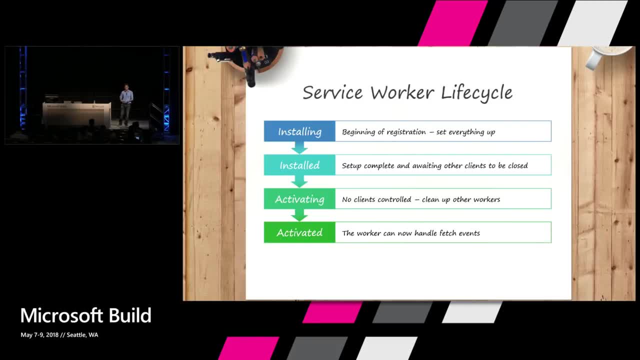 That as well, And then we go to the activated Phase. At this point the service Worker can fulfill its destiny and handle those fetch events That we've been talking about, so that it can respond back to the Page when a request is made. And then, finally, it becomes. 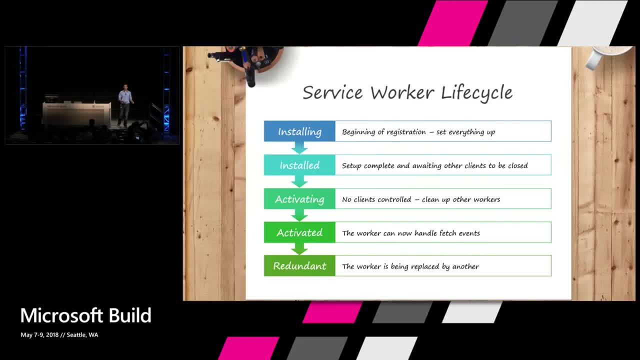 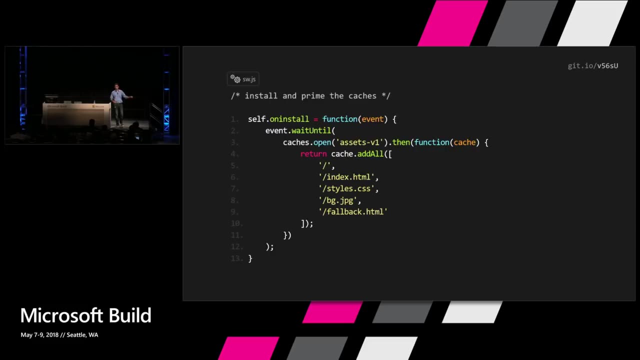 Redundant. This is when the service worker May be replaced by another because it's being updated. So, starting with the first step To install, The first thing that's going to happen is an event will be Fired in the service worker And we're going to handle that. 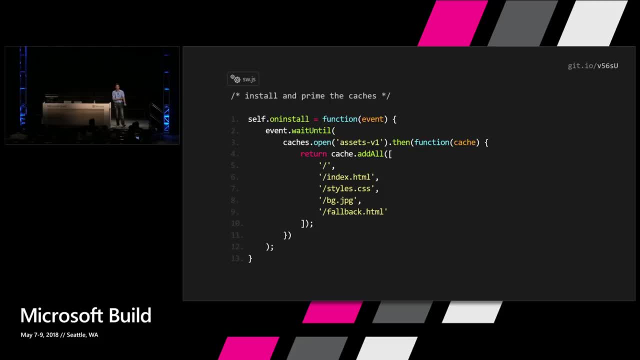 Event. It is the uninstall event And again you can use add event listener as well. So in this uninstall event we are going to use eventWait Until. EventWait until says we're Going to pass a promise into you and when this promise? 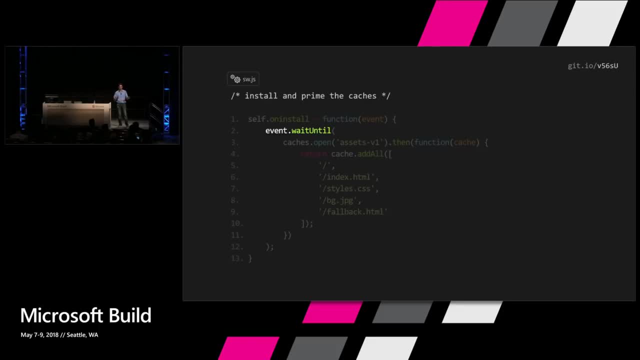 Finishes resolves. we're okay with letting the service worker Go away. So we're going to use the Caches api by using cachesOpen, And caches are a global variable in both the window Objects, so on your main page, and also the service worker as. 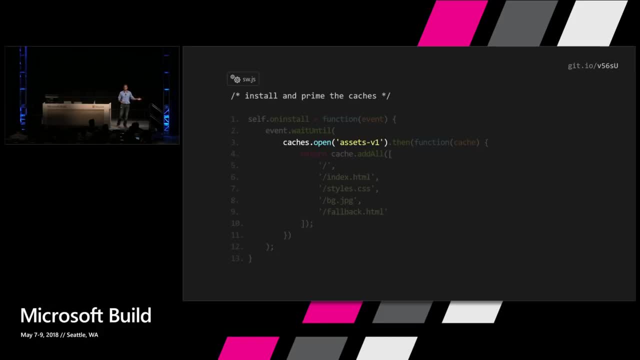 Well, We're going to specify a name for That cache that we're going to open Here. we're calling it assets v1. And then, when that cache is Opened, we will then use a helper method, cacheAt all- And we're going to have a list of things we want to be able to. 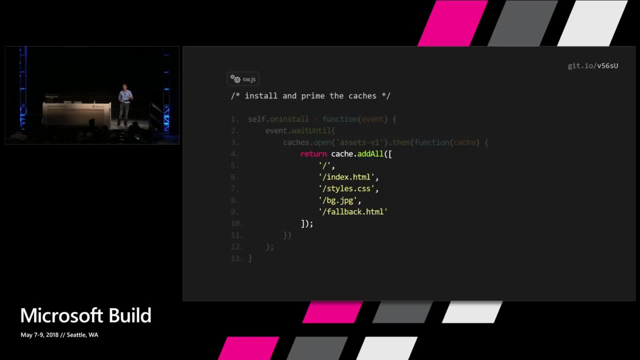 Prime the cache with. These are all the things that we Think we're going to need as part of the shell of our Application, for instance. So these are resources that, if They don't get installed, we're not going to register the Service worker. It's important that these files 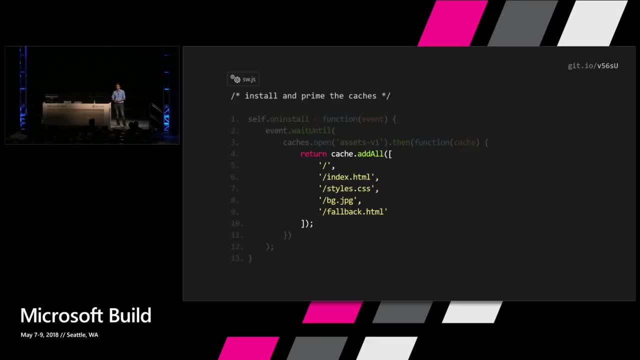 Get installed so we can at least have some base experience for Our application. So that at all is basically Implicitly doing those fetches for those items and then Putting them into the application. It will help us do that. It's a simple way of doing that. 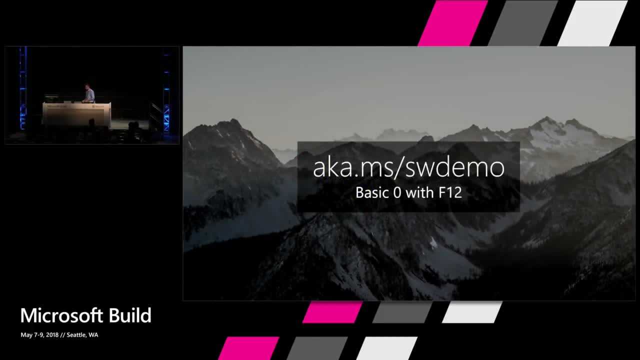 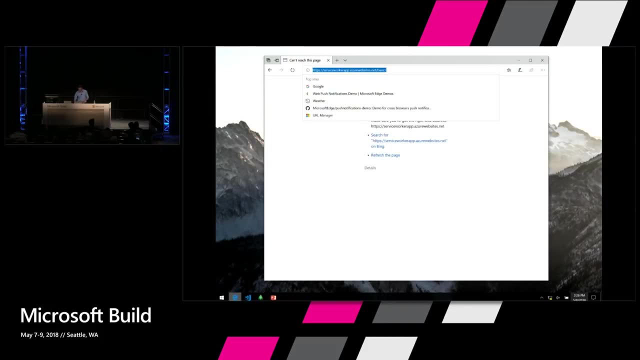 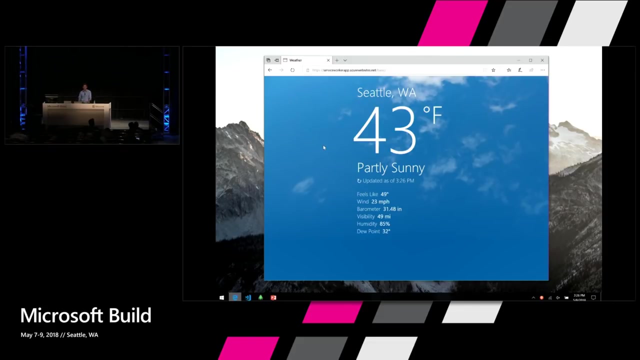 So now that we've done that, let's take a look back at our Demo here. So what we're going to do here is we're going to check out f12.. We're going to see how this service worker looks, Because obviously this, you can't really see it. 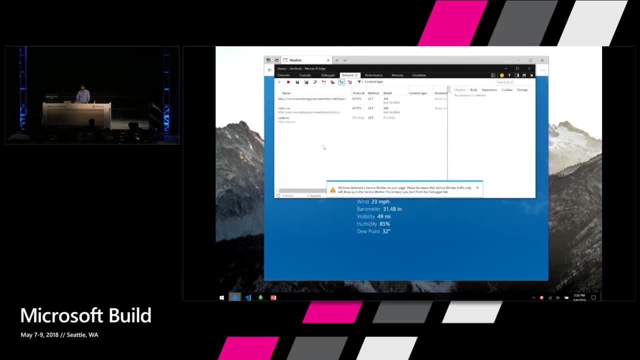 But if you open up f12, there's a way for us to see that Something's going on. The first thing you're going to See is that the page, or f12, is detected, that we have a service Worker for this page And this is important to note. 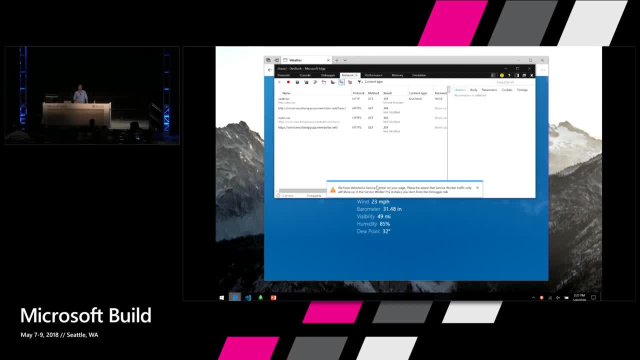 Because if you have any network traffic happening on this page, The network traffic that's being serviced by the service worker Will actually happen in the service worker itself. So what i mean by that is if we go to the debugger, we're going To see our domain. there. We have a bunch of service. 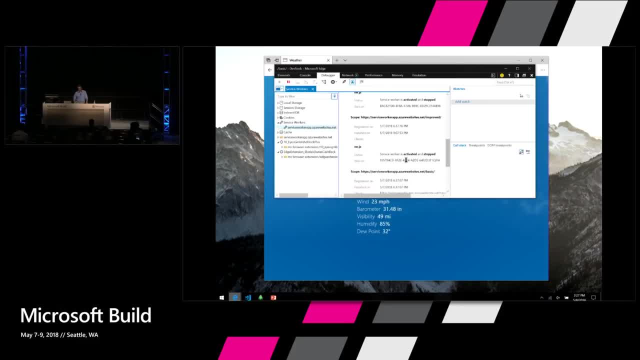 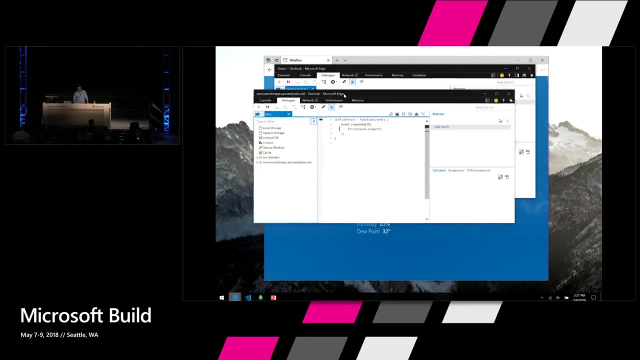 Workers here installed for each of the demos i have, but we're Going to scoot on over to the slash basic, which is what this Demo is. I'm going to click on the inspect Link, which will then open up a separate instance of f12. 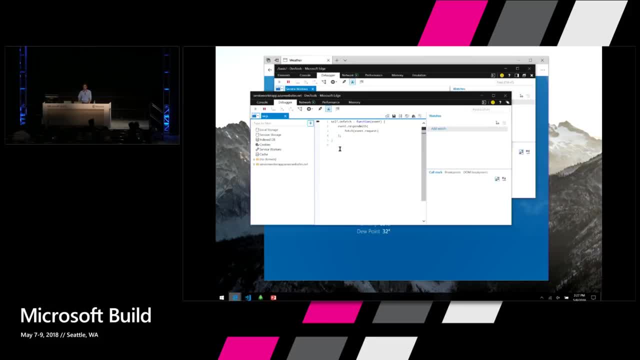 And in this instance of f12, i'm able to see the javascript that I had written before. So i'm going to click on the Javascript, And what i can also do is i Can go to the caches and inspect the caches as well. 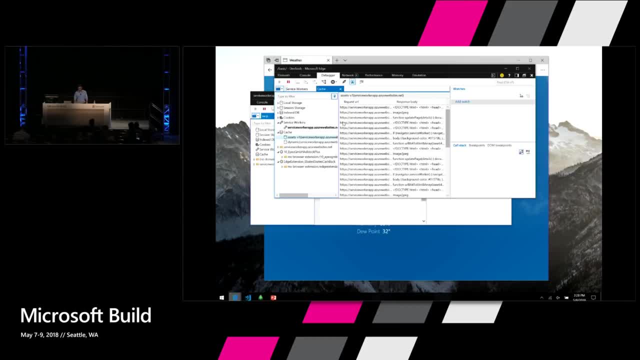 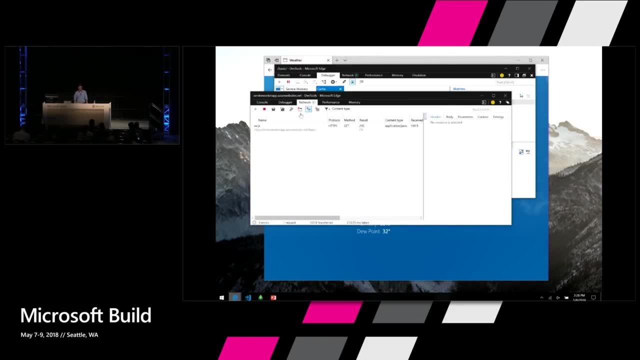 So under assets v1, i can see a bunch of resources here that are cached- And what i was trying to say before about the network Traffic. if any network traffic happens in the service worker, It's going to show up in the network tab of the f12 instance. 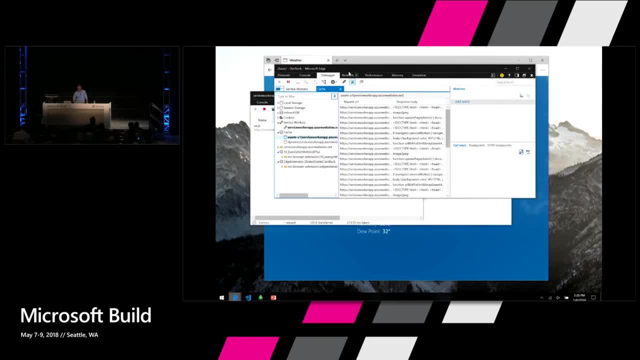 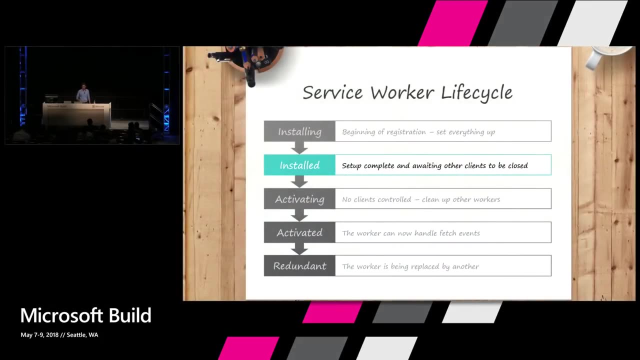 Debugging that service worker. So if you have any network traffic Happens in the service worker, it's going to show up in the Service worker, So you won't see it here, And that's what that warning is about. fyi. 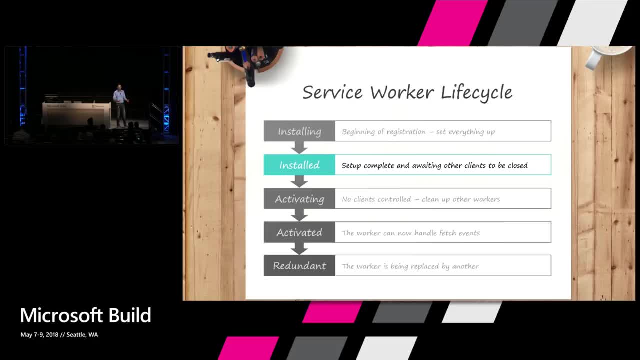 Okay, So now we've gone over to the Installed phase And once those clients have Been closed off, we've closed off all those tabs. we're going to Move to the activating phase. This is going to now signal the Service worker with another event. 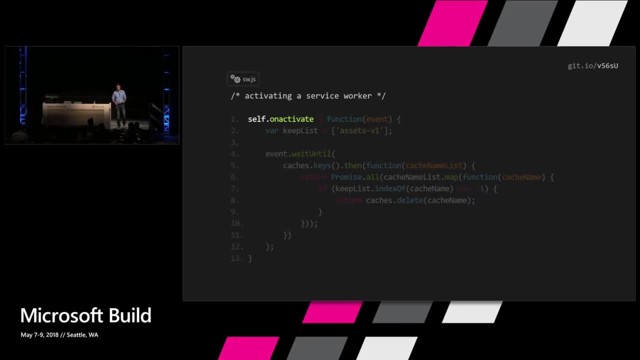 The on activate event Again selfAnactivate. It's a different event here And in the service worker we're Going to have a list of caches that we want to keep, So we're going to define a keep list Here. we want to keep our v1 caches. 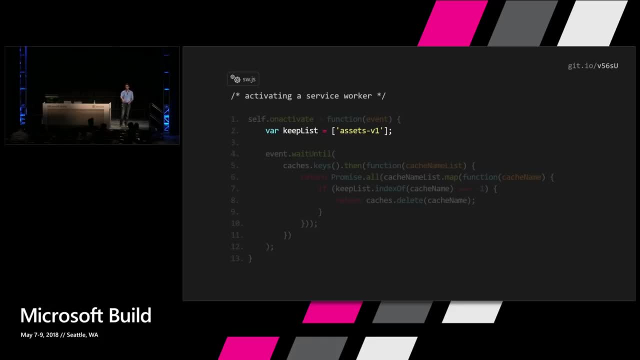 So, even though we're upgrading, for instance, our service Worker, this would be the opportunity for us to clean up Those older caches, if we needed to. Again, eventWait until So. we're going to wait until That happens, And what? we're going to wait. 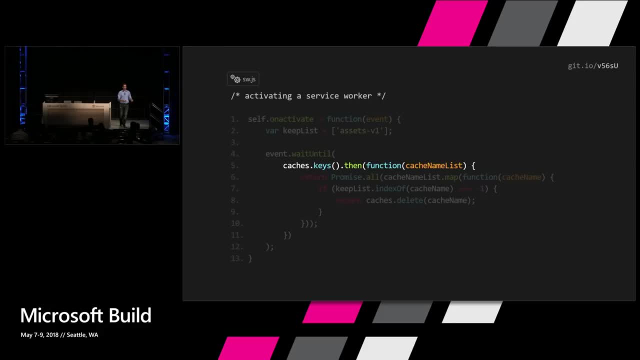 Until is we're going to use cachesKeys to get all of the Things, all of the different caches we have, And then we're going to permute through them. And when we permute through them, we're going to check if Any of those things are inside of the keep list. 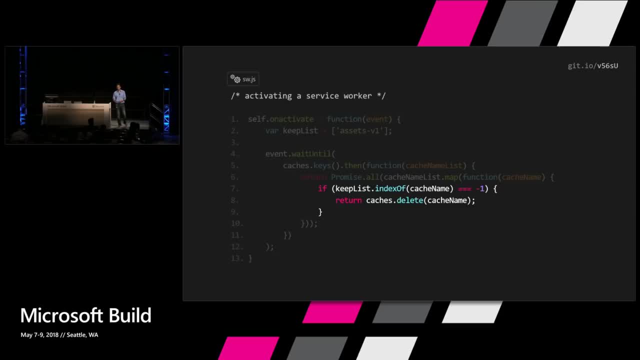 And if they are, we don't delete them, And if they aren't, we delete them. By the way, on the top right corner i have gitIo links if You want to get, if you want to see these samples, so you can. 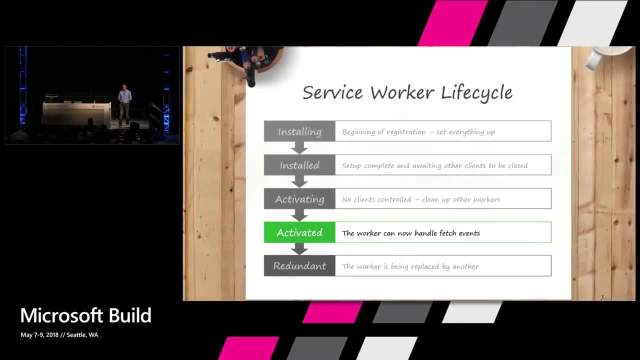 Consume them later. So we're going to wait until that Happens. So now we've gone to the Activated step. So again, the service worker Can now, now that it's activated, fulfill its destiny to Handle those fetch requests. So back to that example where we 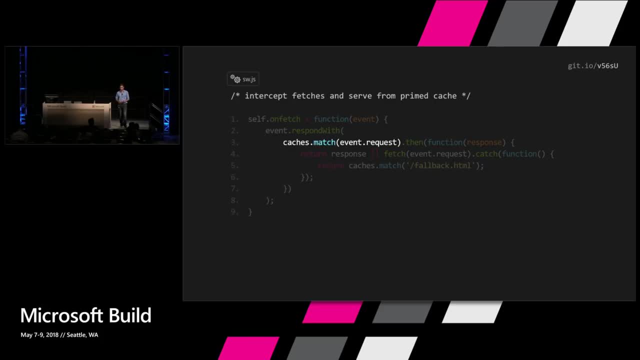 Have selfOnfetch. we are going to. instead of just going to The network and doing a pass-through, we are going to Do cachesMatch, where we're going to ask for a specific Request that we just got from the caches And if it's there, we'll return that back to the page. 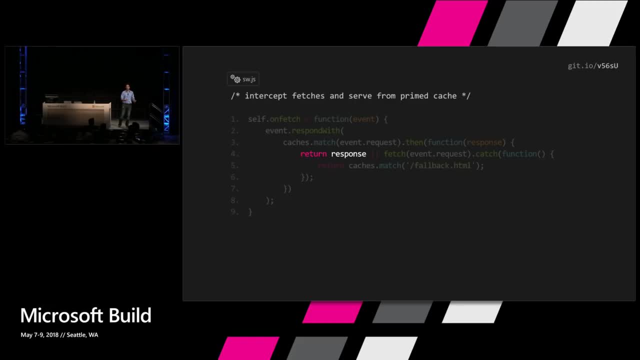 And so the page now has, or it's loading, what we just put into The cache during our install step. If we don't have something in the cache for that specific Resource, we're going to instead just fetch it from the network As sort of a fallback. And if we don't even have the 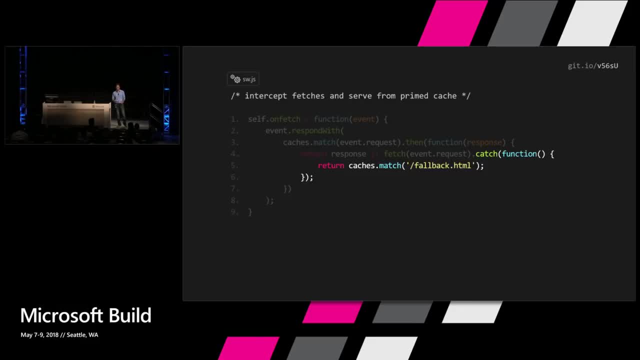 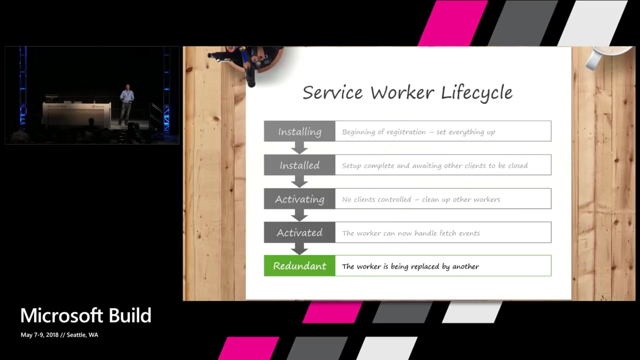 Network. if that fetch fails, using the fullback, we're going To return. something we do know is in the cache, that file that We've cached as part of the install step, the fallbackHtml. So again at the final step. now you are at the redundant state. 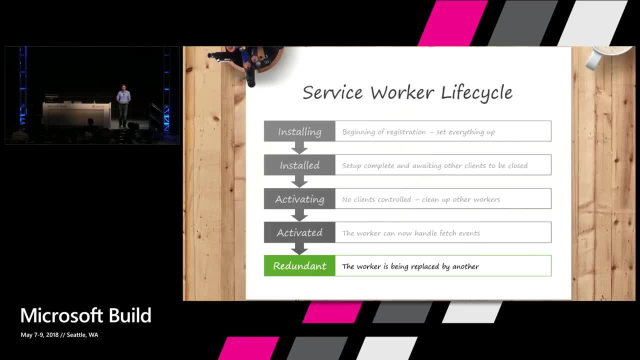 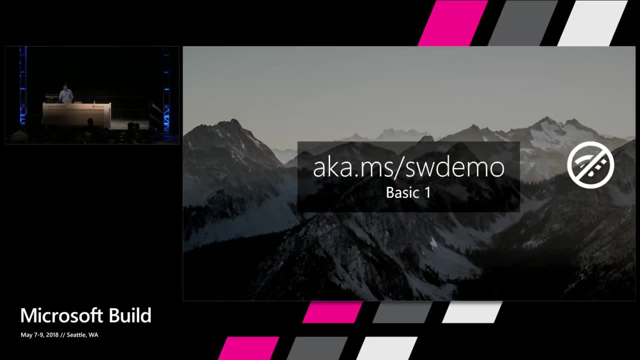 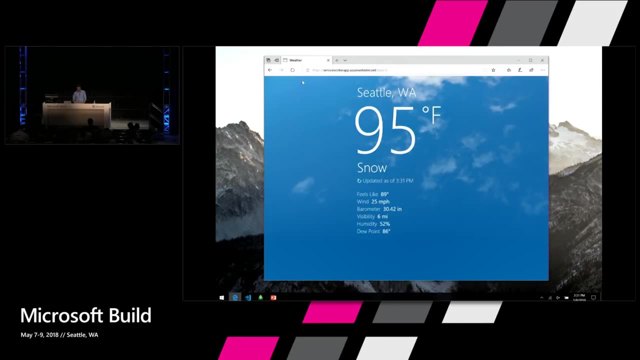 If a new service worker is being registered to take its place. So we're going to switch back to another demo Now that we've done all that fancy stuff, and see what that Looks like. So here we are, We're online, We're loading it up. 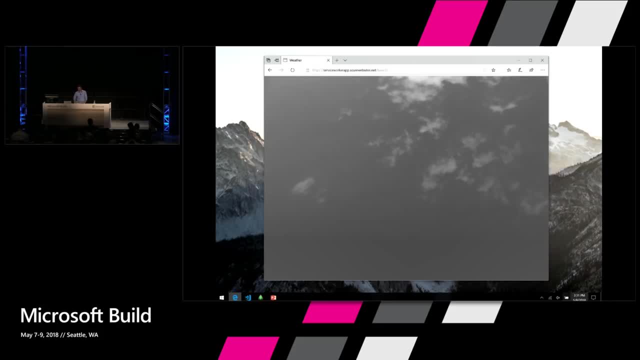 Looks all fine and dandy. All right, Let's disconnect from the network. see what happens. Please connect to the internet and retry. So we can do better than this then- And in fact we will, So something we're going to do. 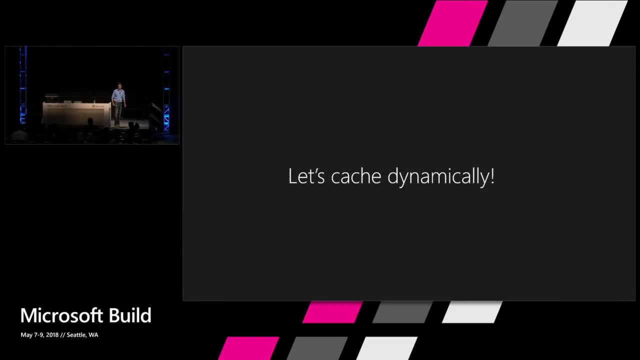 Something we weren't able to do before with the caches- with App cache- was being able to cache dynamically. This time we're going to cache dynamically. So what we're going to do is, instead of doing that fallback, Step inside of our on fetch handler. we're going to instead. 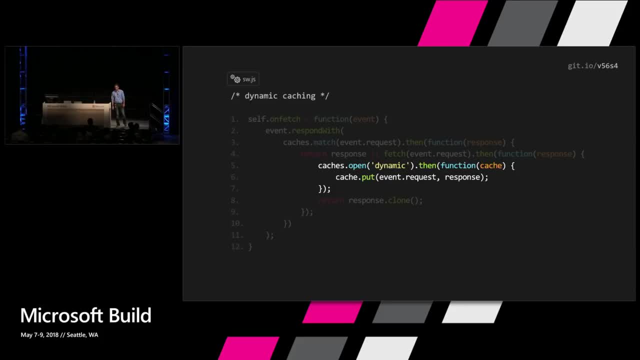 Open up a new cache and call it dynamic and then put that item That we just got from the fetch into the cache, into that New dynamic cache. So we're dynamically caching if It's not already in the cache. And then we also want to still. 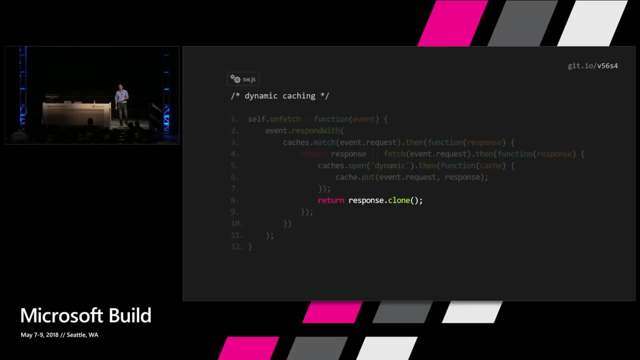 Respond back to the page with what we just got from the fetch. So we're going to use, we're going to return the response, But we're also going to have to clone it because that response Just got consumed by the put operation for the caches. 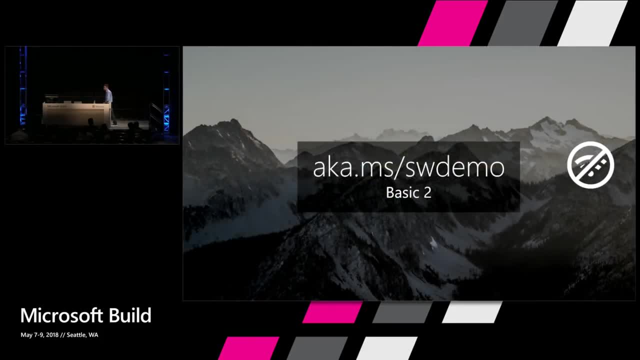 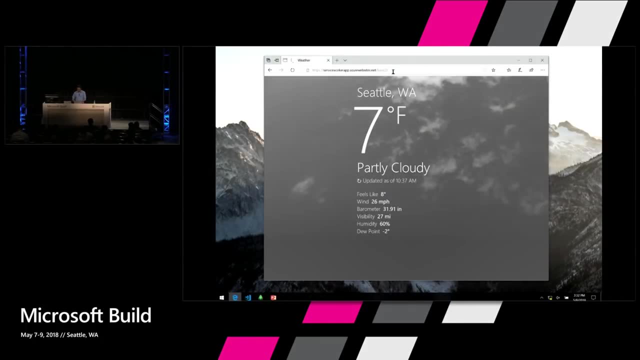 So it's important to note that you have to do that. So now, if we switch back to the demo with this new improvements, We're able to get an offline experience where it shows me The last known state. So that's better And, of course, if i'm going to go online again, 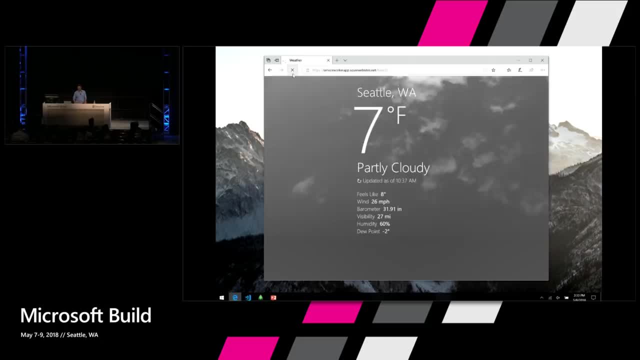 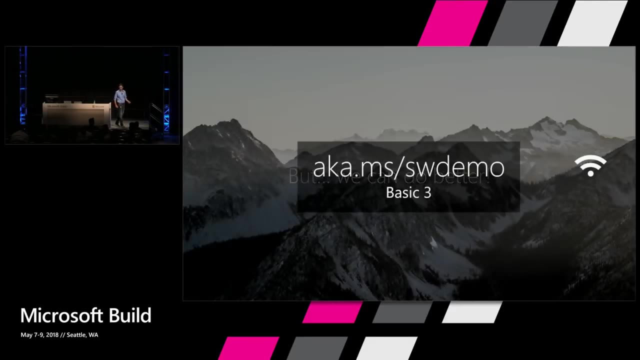 So i'm caching dynamically, but i haven't accounted for the Facts, So we're able to get an offline Experience, with the fact that if i'm online, i want to get new Data. So back to the drawing board. All right, So we can do better than this. 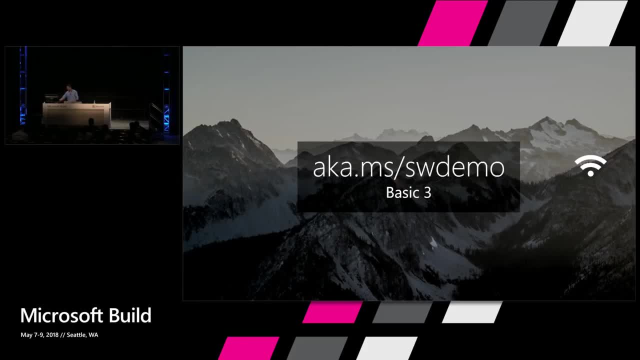 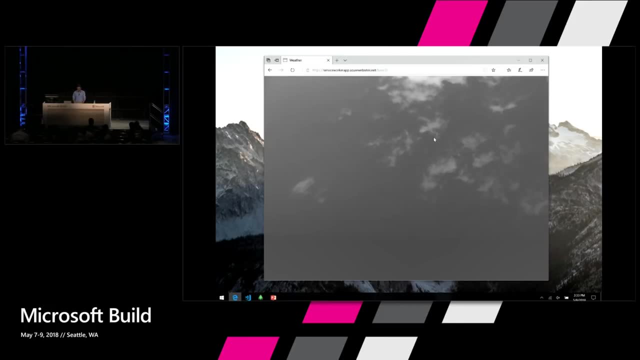 And i'm going to show you what that looks like. So what we're basically going to do. as you would expect, if You're online, show something And if you're offline, don't. I'm going to spare you from that demo. 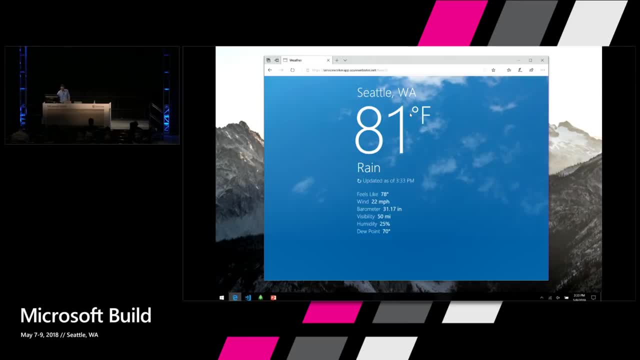 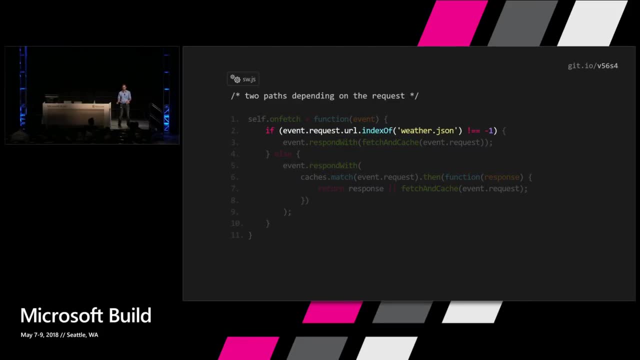 I'm sure you guys know what that looks like. So how do we do that? going back to our on fetch Handler, we're going to have two different paths. The first path is going to check if we're making the request for The weatherJson. If so, we're going to respond. 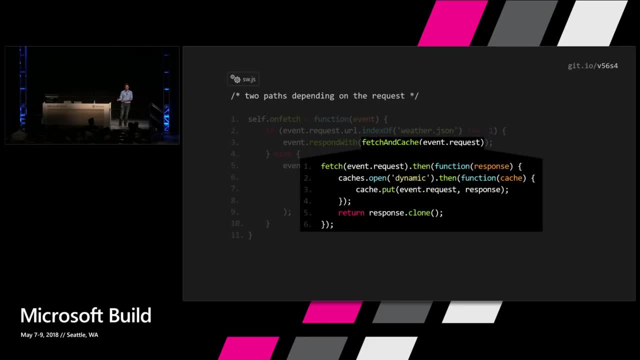 With a fetch and cache And the fetch and cache is just Doing what we did before. I just encapsulated it as a Method here, So just opening up that dynamic Cache and then putting it into and then doing the fetch and Then putting it into that cache and then responding back from. 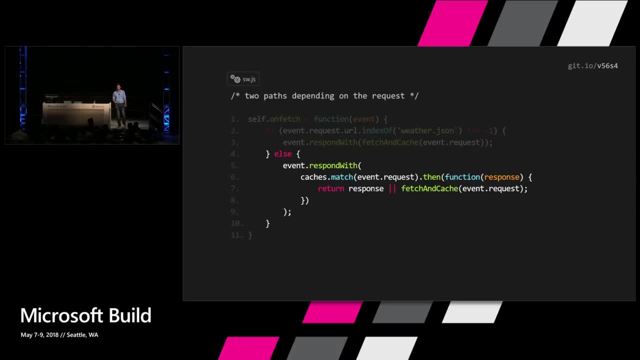 That request. Otherwise we're going to do What we were doing before. So on the weatherJson file, We're going to just do a fetch and cache. We're not going to do a from cache first And then, of course, on the page itself, on indexHtml. 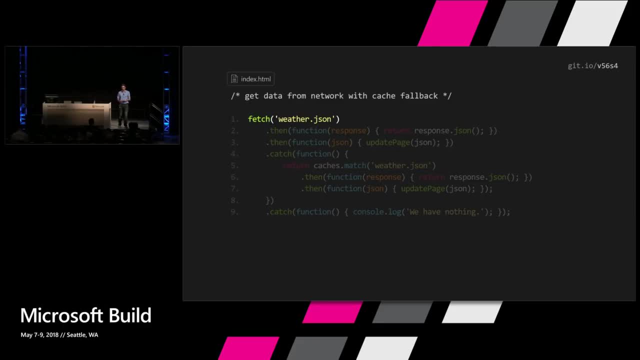 We're going to request that weatherJson and do something Special here too. So what we're going to do is we're Going to do a fetch and cache. So when that request comes in, We're going to get the json, like we were before. 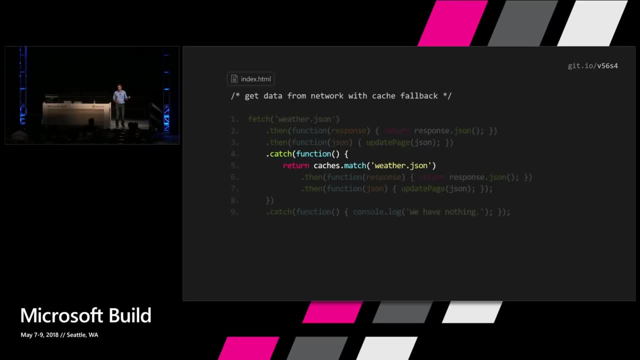 And then we're going to update that page with the json And then, if it fails, well then we can just get the thing From the cache, So that if you're not connected To the network, you're still loading it from the cache. 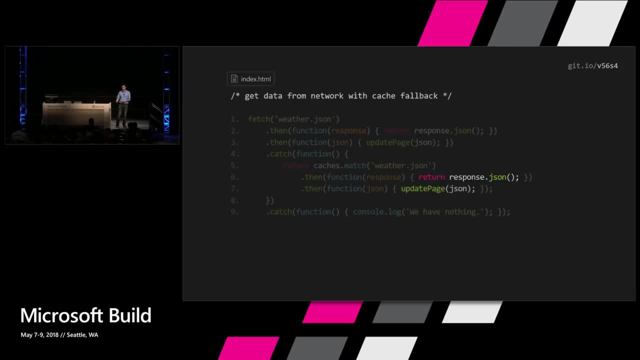 And we're going to do the same thing there. So once we get it from the cache, we want to get the json And then update the page with that json And then, if all else fails, if we don't have the cache and we 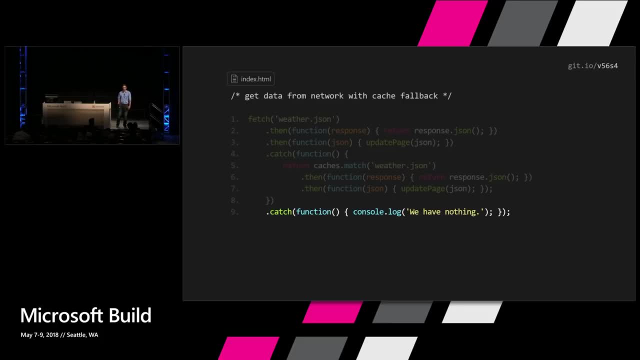 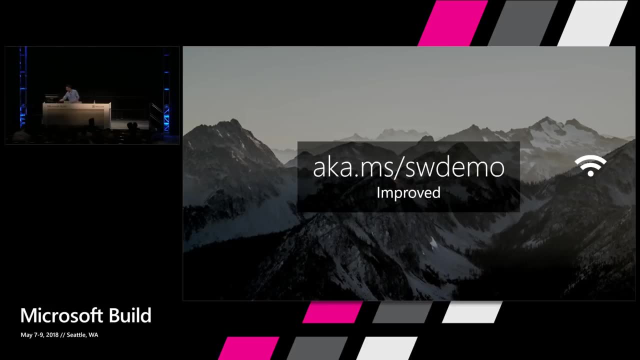 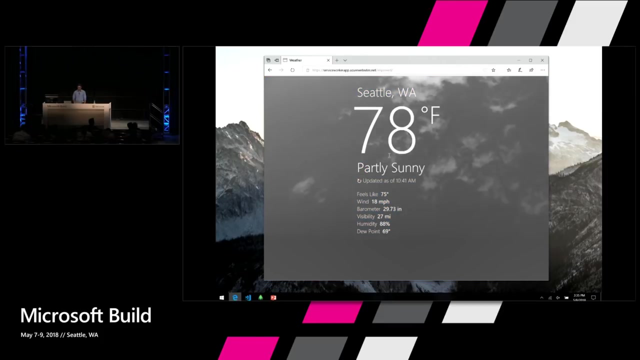 Don't have a network connection. well, we got nothing. You may want to show a different experience for that, But we can do even better than that. So what we'd really like to do is offer an experience where, When you're connected, it's going to show that very for a 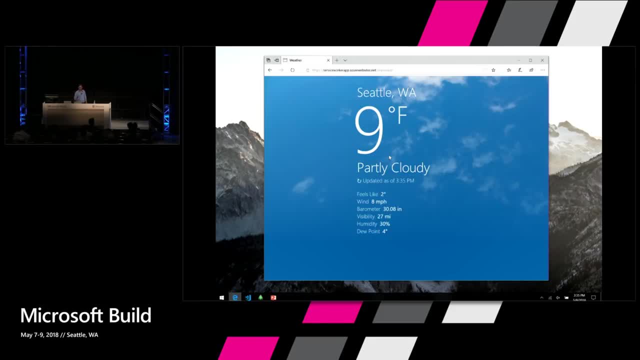 Brief. second, i'm going to show you that again It's going to show the offline experience where it's showing it From the cache. I'm going to show it again And then it's going to load immediately freshly from the Network. Again, this is sending me not. 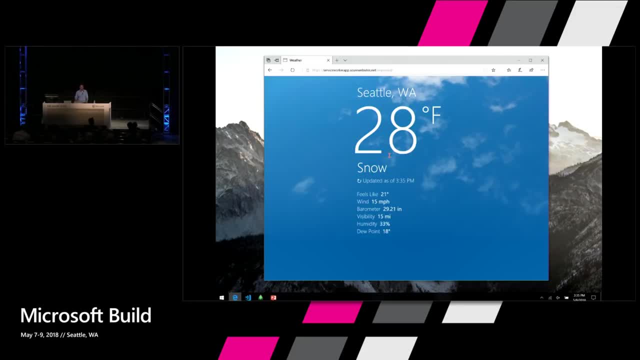 Nonsensical data to show you that it's updating from the Network. So this is what we'd like to do, And if i turn off the network here, it would just load that Offline experience and then that's it. So now we've gone to a state where we're behaving like that. 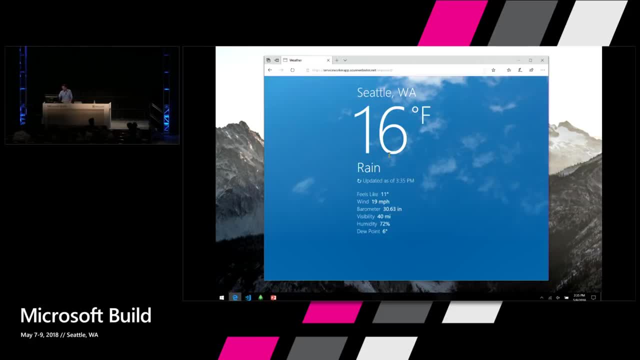 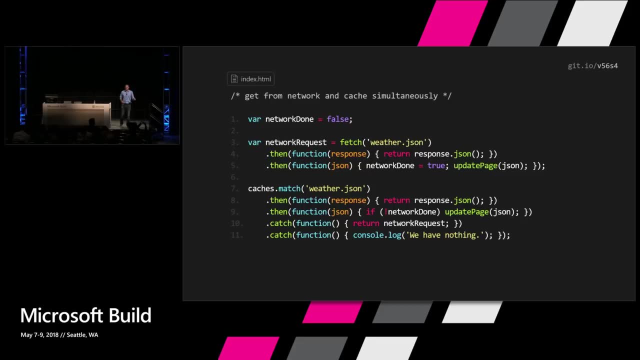 Weather app was at the beginning, And so you're wondering how we Do this, So let's take a look. So what we're going to do is we're going to race the network With the caches. So what we're going to do is we're. 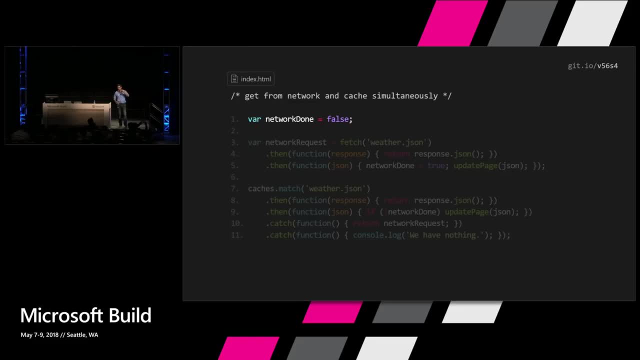 Going to set a global network done, set it to false because It's not done yet. We haven't done it yet. We're going to then assign that. assign the network request Variable to a fetch request for that weather dot json. and then 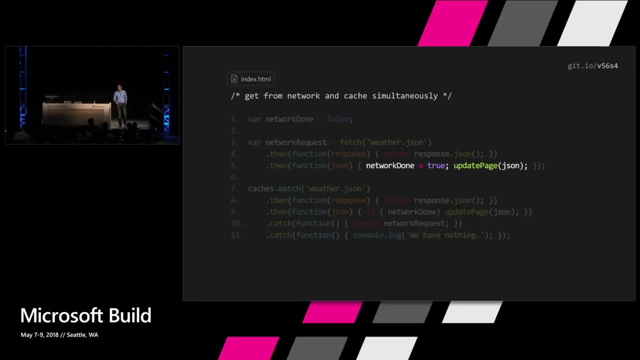 Again, we're going to get the json from it and we're going To set here the network done equals true, and then we're Going to update the page. At the same time, we're also Going to make a request for the cache for that same file. 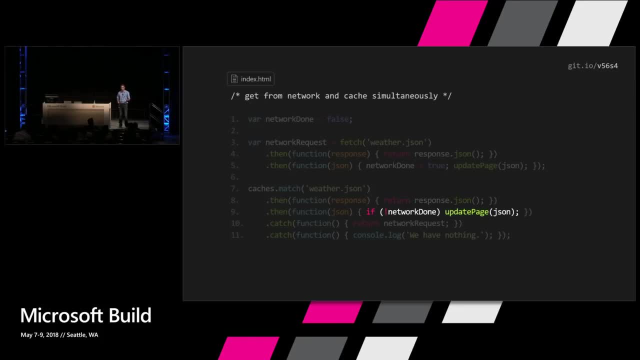 And if we get it again, we get the json from it, And then only if the network isn't already done will we Update the page with the cache, because it's possible in some Circumstances that the network may be faster than the cache in. 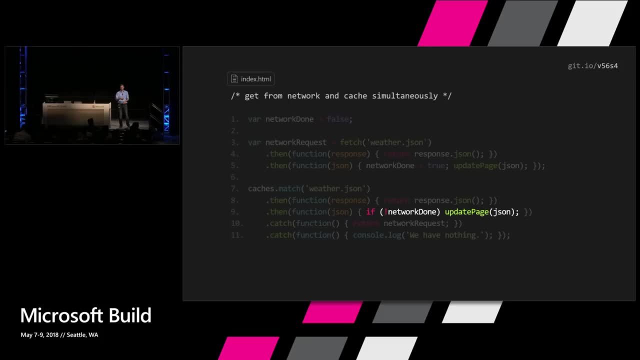 Which case you don't want the cache data to supplant the Network, the fresh network data, And if we don't have anything in The cache, we're going to do a dot cache and then we're just Going to return that network request, the variable that we 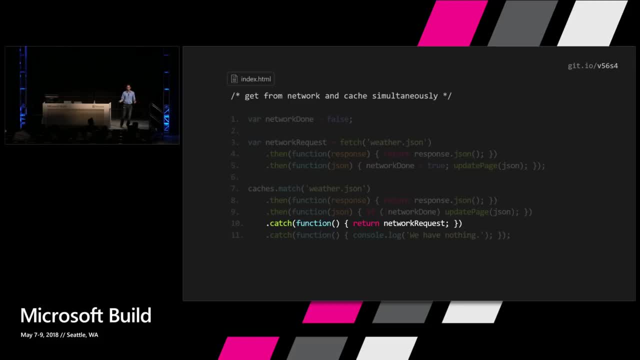 Said before for the fetch, in which case the network is Basically our last hope. It better have something in the Last hope, And if we still have nothing Because the network is not there and we haven't cached it Yet, then we would have a fallback experience because we 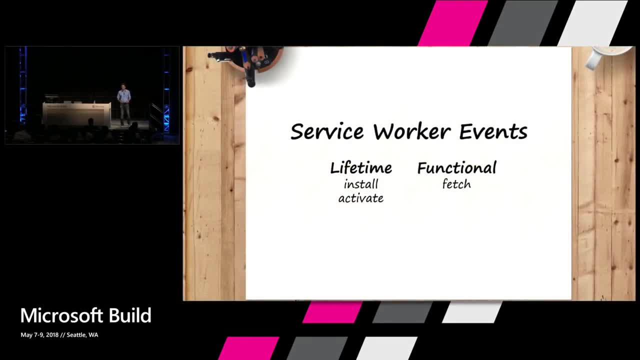 Have nothing. So so far, we've really been Talking about two different types of events: Lifetime, where we have the install and the activate and The functional, The fetch event- And we spent a lot of time talking about this fetch event. 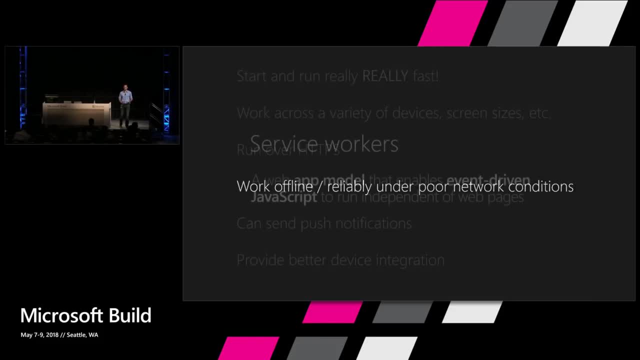 And talking about working offline and reliably under poor Network conditions. But service workers are a lot Better. And service workers are a web App model that enables event-driven javascript to run Independent of web pages. This is a very powerful Mechanism that could enable other experiences. 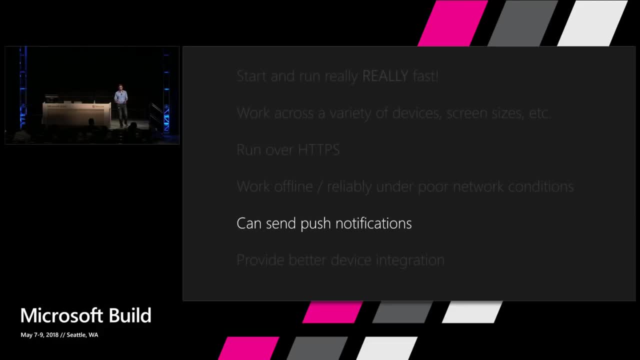 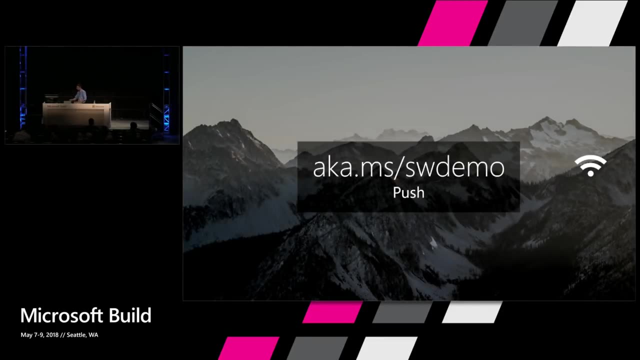 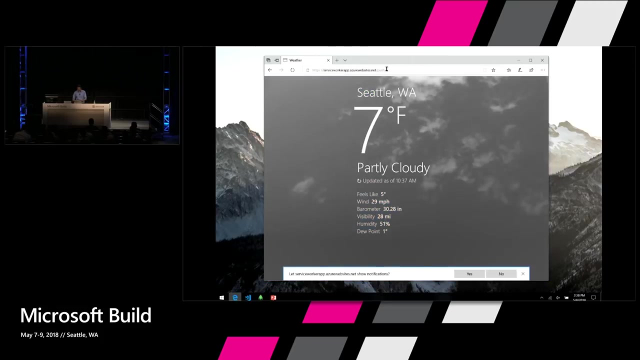 Namely, if you recall, that push notification scenario we were Talking about before, So i'm going to show you what This might look like. So, switching on over here, i'm Going to show you what this might look like, So i'm going to go to my push demo. 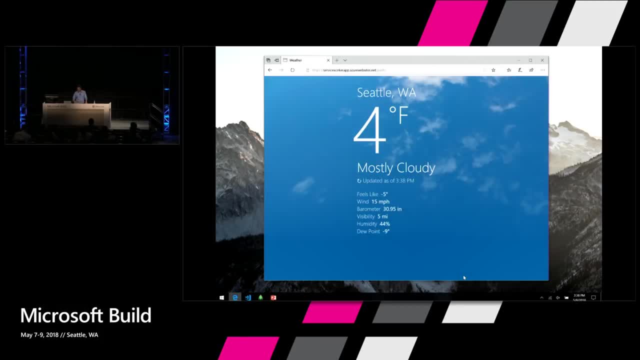 It's going to ask me if i want to show a push. I'm going to say yes, I'm going to give it a second And then i get a weather advisory notification on the Bottom right here. In this case, it's just. 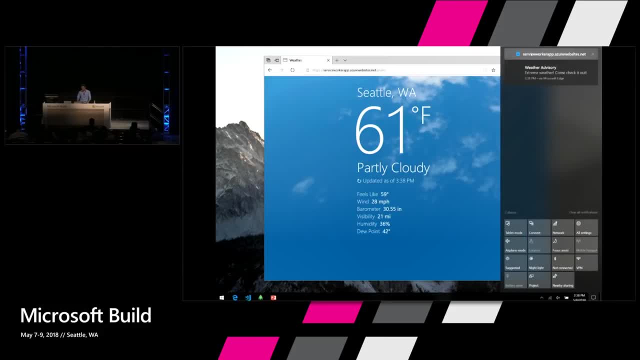 Basically loading it up and then showing it, And it gets integrated into the action center on windows. So you get to see it here And if i don't act on it, i can Act on it later and click it and it will show up. 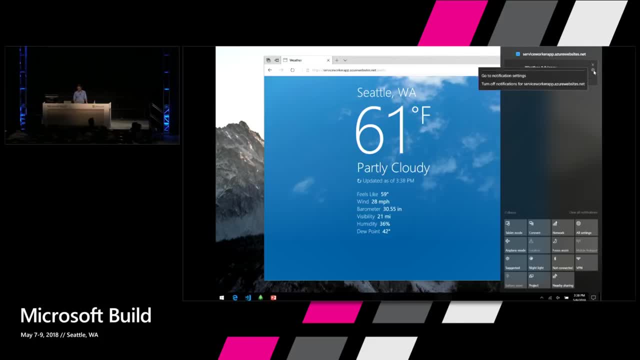 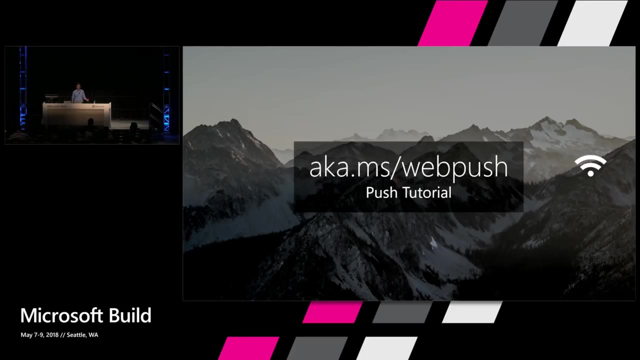 And it will do what it's supposed to do. I can dismiss it and do the other nifty things i can on Windows, like turning it off, for instance. So we've also built, as part of this talk, a demo, a push. 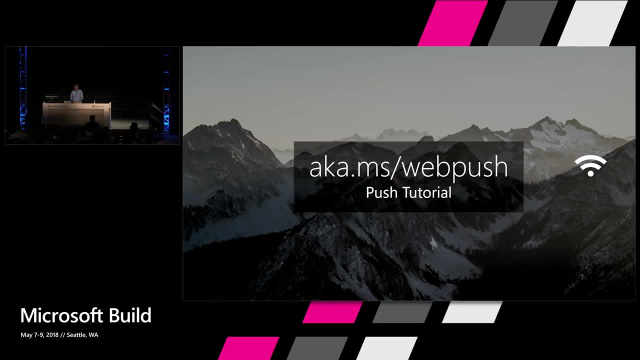 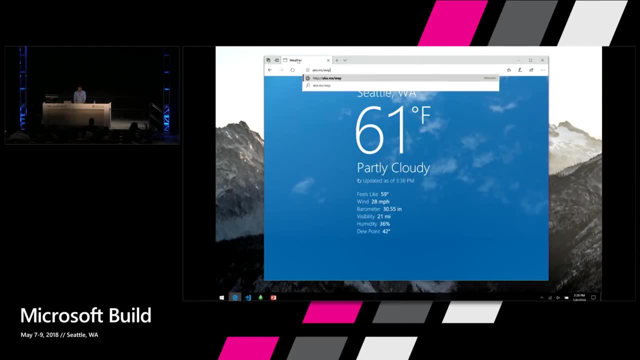 Tutorial that you can follow if you want to understand more About how web push works. I'm going to show you that Tutorial right now. So it's akaMs slash web push. I'm going to show you that demo, that tutorial, right now. 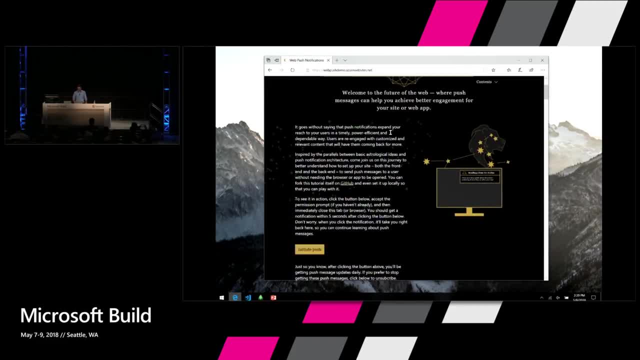 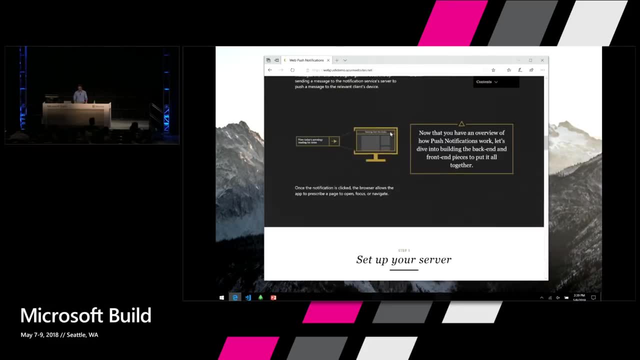 So basically it will walk you through the different steps on How to set up the server and the client side in a nifty little Way. here I'm going to scroll down, So this is just kind of giving you a sense of what this looks. 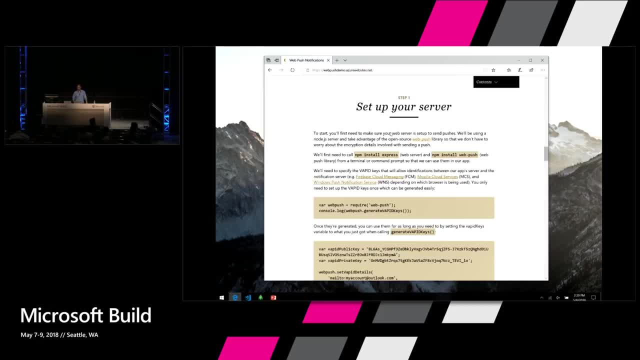 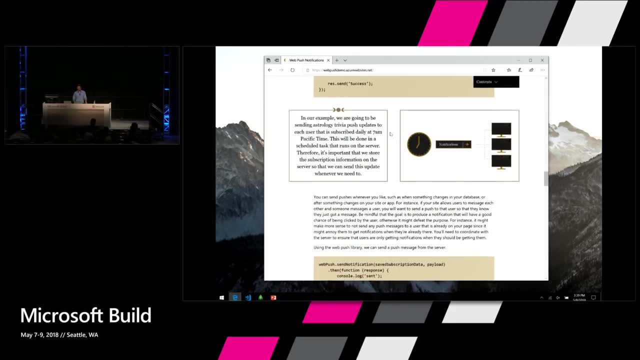 Like. I encourage you to go to this url And learn more if you want to learn more. We're going to walk through some of the basic concepts here, But this is a fully working demo that you can also fork on github To understand the concepts that we're going to talk about. a 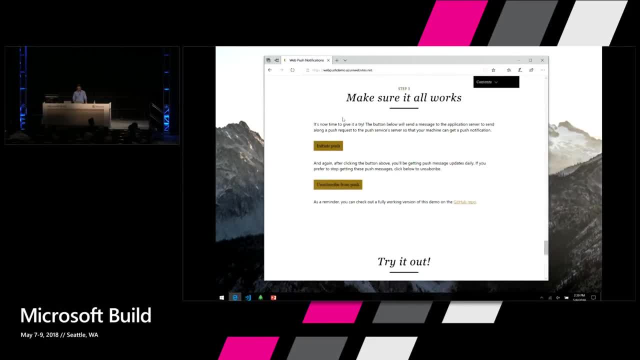 Little bit better, And so, to kind of give you a Sense of how this works, we're going to walk you through some Of the steps on how this works. If i click initiate push here, It's going to show me a push message that i can then click. 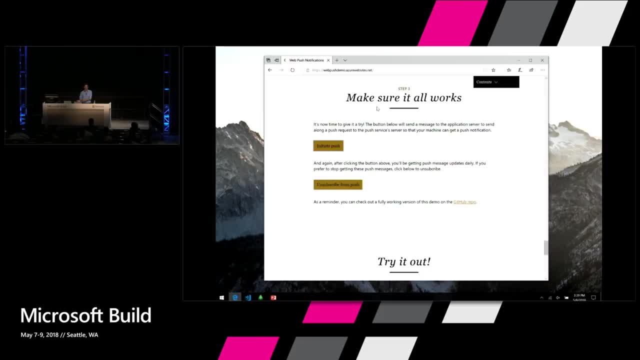 And then it would reopen the page. Of course, in this case i'm Already engaged with the page, so it's going to just focus the page. So let's talk a little bit about how push works. So you have your page and you have the service worker. 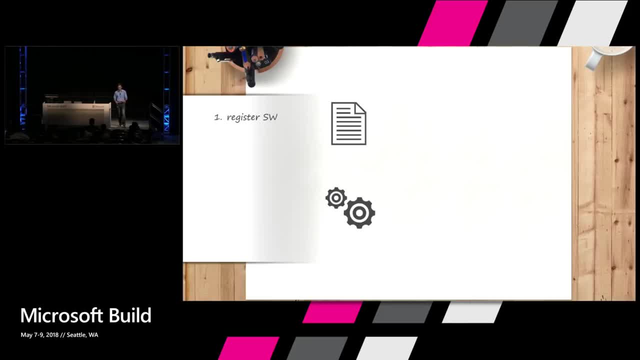 And of course the first step is to register that service Worker, like we've been doing. But so far we've only been Talking about the client side. Let's bring in the service worker Side as well. So the first thing we're going- 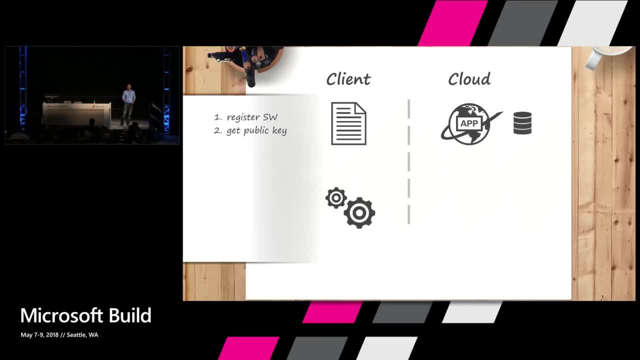 To need to do is talk to our application server and get What's called the public key. We're going to need this to Subscribe for our push message so that we can set up our push Message channel to get updates from our server. The next step is we're going to subscribe for the push. 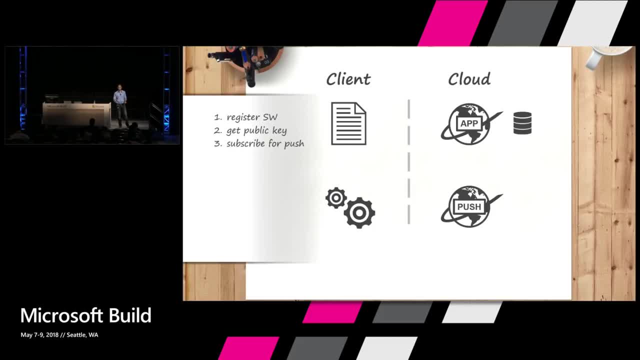 And that's going to talk to the push services server And in edge's case, microsoft, edge's case it's w3.. There's fcm for chrome and there's mcs for firefox, So they're all different, But we're going to do it in a 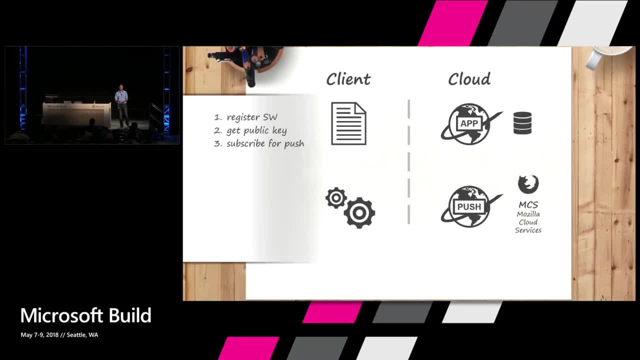 Standards-based way that will work across all the different platforms. So we're going to make that request to subscribe from the Push server. We're going to get that Subscription data and we're going to save it on the cloud. We're going to save it on our application server. 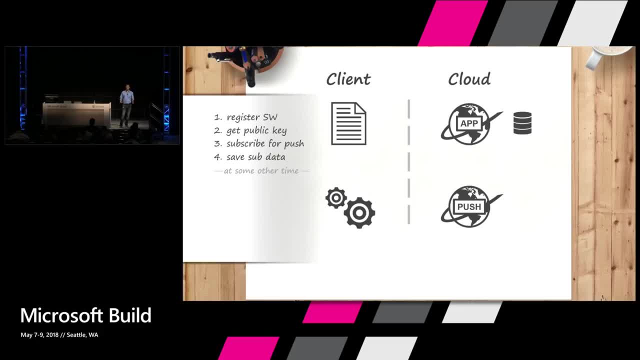 The reason for this is because, at some other point in the Time, we are then going to get that subscription information, Which is going to have, for instance, the end point url That will tell us exactly where to send a message to, which Will then notify the push service again using that end. 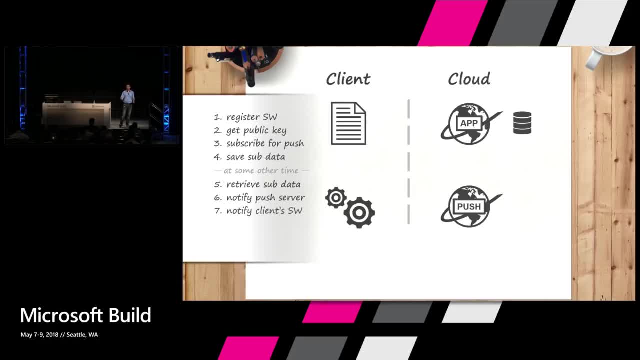 Point url and then that push service will know how to talk Back to our client, our client device, and notify that service Worker that we got a push message. And again, once that service worker gets that message, we're Going to be able to show a notification. and when that? 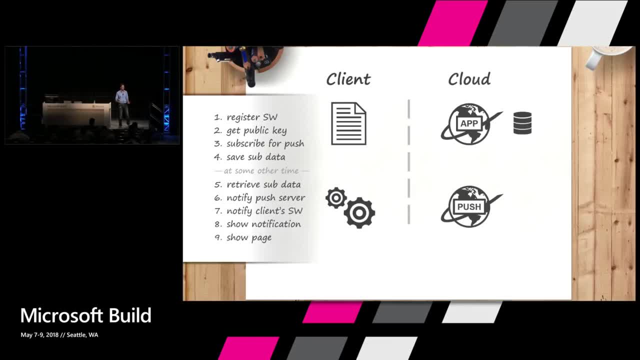 Notification is shown, we can click it and then it can do Something like show the page. So we're going to walk through The different files that would be involved in making this. We're going to be using a node js server to build this, but you 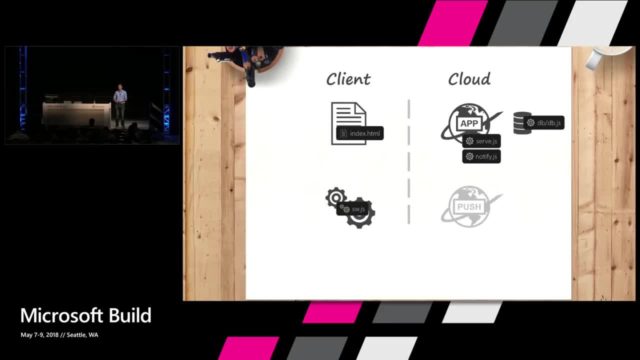 Can build it with other types of servers. I'm using it because i'm going to be using the web push library, Which will help us kind of abstract away all of the Encryption and cryptography that we're going to be using. So the first file, the indexHtml, which is our page. 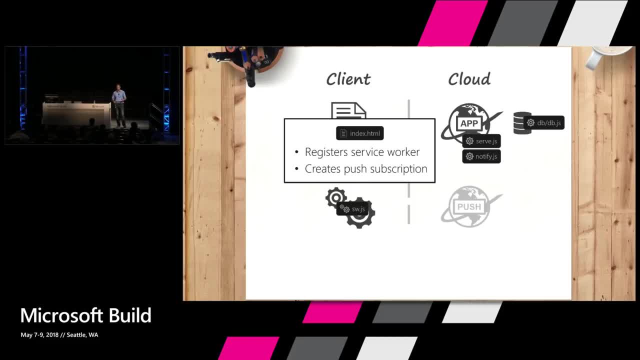 It's going to be handling the service worker and creating the Push subscription, And then the service worker is Going to handle the push event and the notification click event. So when the notification actually gets clicked, it's Going to be handling that as well. And then we're going to have 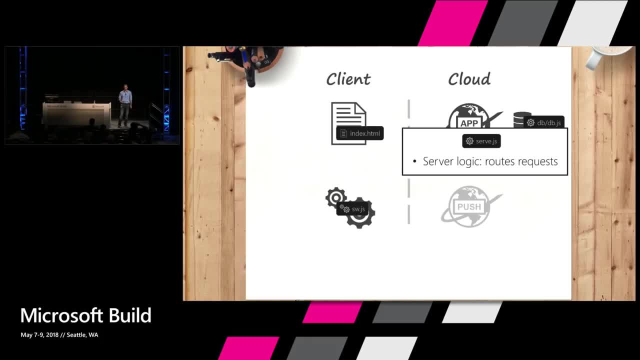 Our dot js, which will actually handle the server logic. It will be routing all the requests so that it's going to Be able to send requests. So the api end points that we're Going to be using will be routed through that And then we're going to have a database file. that's basically. 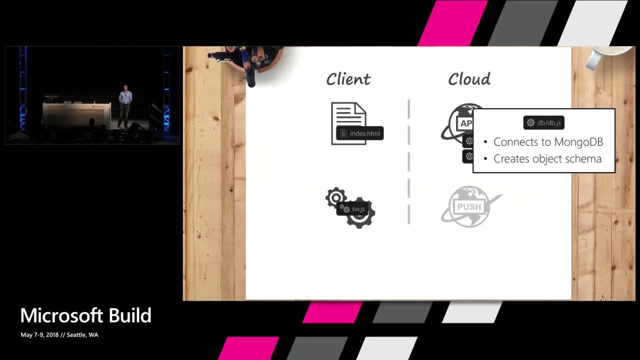 Going to connect to some back end database, for instance Mongo db, which is what we're going to be using here, And then it's also going to create the object schema for the Data we're going to store. I'm going to show you how that. 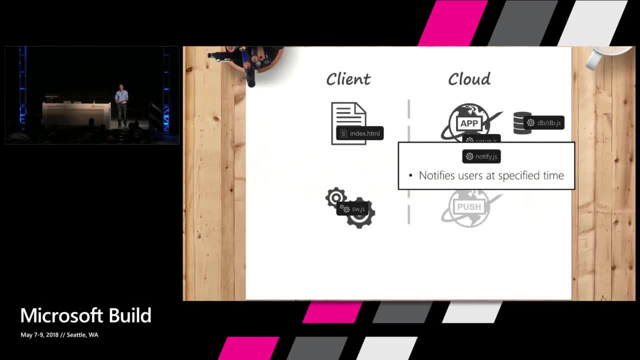 Looks as well And we're going to have a notify Dot js. Again, this is all server side. This is going to notify the users. It's going to send a push at some other specified point in Time. So from the client side, we're. 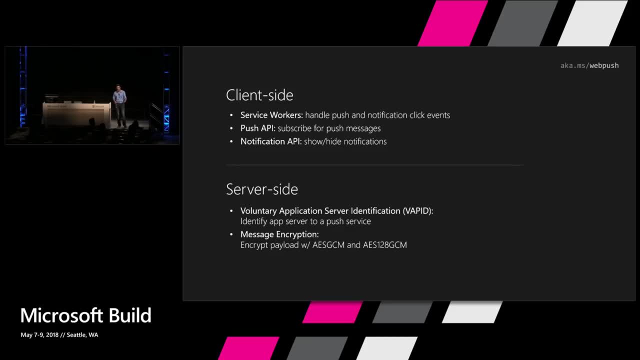 Going to be taking advantage of service workers, the push api And the notifications api. From the server side, we're Going to be using something called vapid, the voluntary Application server identification. It's kind of a mouthful. All you need to know is that. 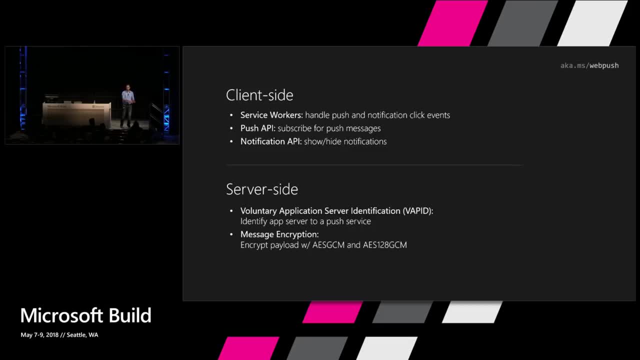 It's going to allow our client to interface with the push Services server so that it will know who it's talking to. So it's a great tool. And then we're going to have a Contract, sort of a handshake. You're going to see what that 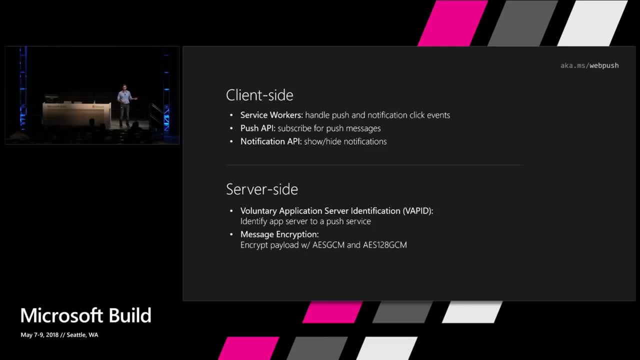 Looks like in a bit, And we're also going to be Dealing with message encryption And again, we're going to be Using the web push library that's available via node so that we Don't have to deal with the actual encryption logic. 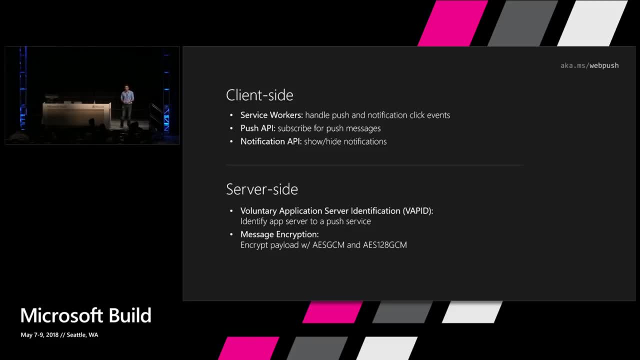 We're just going to be using helper methods that are going to Do that for us. But it's worth noting that there Are two types of content encoding types: aes gcm and aes 128 gcm. So to set up our server, we're going to be using the 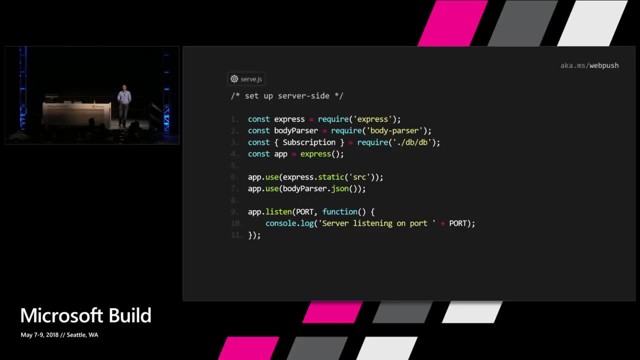 Express. If you've never used node, It's just a minimalist server that we can use, And so we're going to set that up. require express and we're Going to use the body parser so that we can get the json from Any of the responses we get. We're going to include that db. 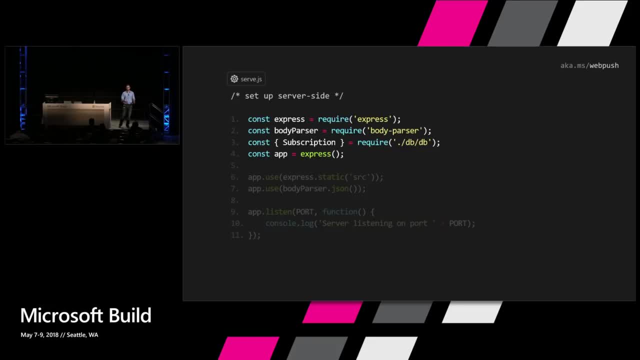 File that we were talking about before, and then we're going to Instantiate the express server as well, And then we're going to tell express to use some directory And serve them statically, and we're also going to tell body Parser to use json. Now, these details are not that. 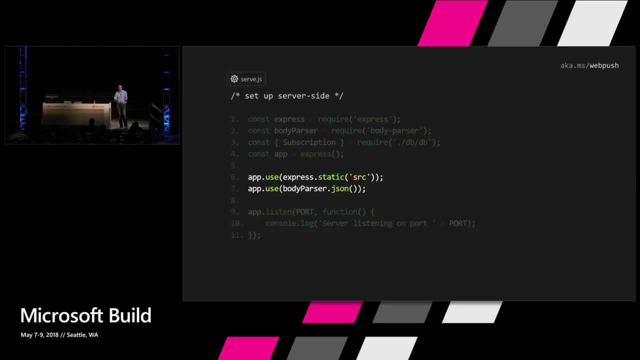 Important. It's just kind of getting us Set up for the server, but it's important to know how exactly We're going to do this, so that it's not magical, it's not Smoking mirrors. There's something happening here That is that i'm hoping to demystify. 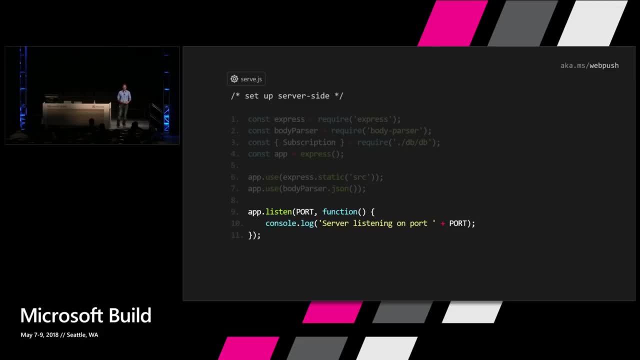 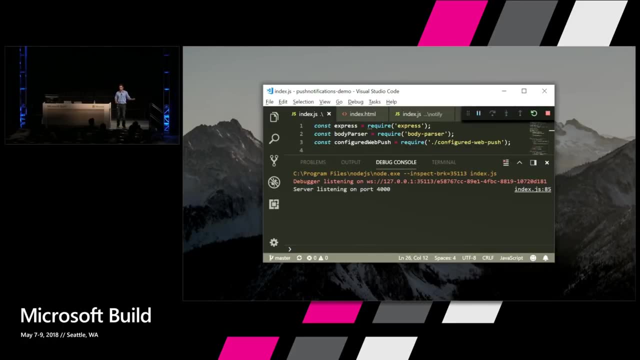 And then we're going to tell it to listen to the port of our Choosing. I'm going to be using 4,000.. And then if you run this in, for instance, visual studio code, You'll be able to see that our server runs. 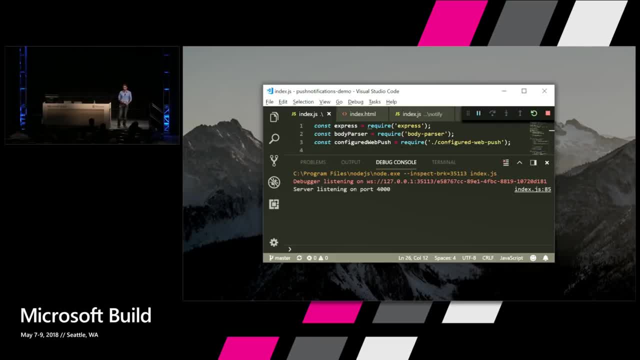 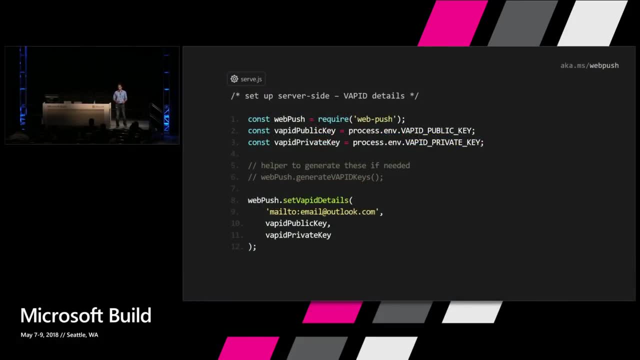 And it's listening on the port that we specify. And at this point you really haven't done much. You just kind of started up a server. So this is where it gets more interesting. We're going to include that web push library that i was talking. 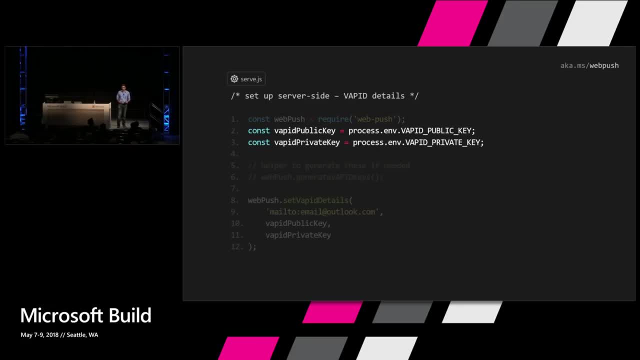 About as part of the first step. Then we're going to specify two Keys, a public and a private key. This is about that vapid thing i Was talking about before, so that we can interface with the push Services server to let it know what the client is doing. 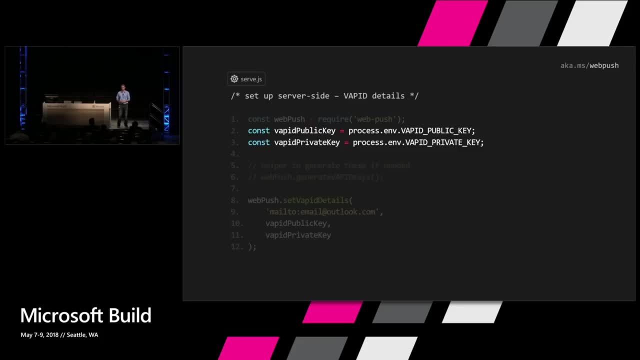 So that it can identify itself to the push services server. In this case, you can actually generate these using a helper Method, using the web push library. It's just web pushGenerate vapid keys And it will give you those keys that you can then put into. 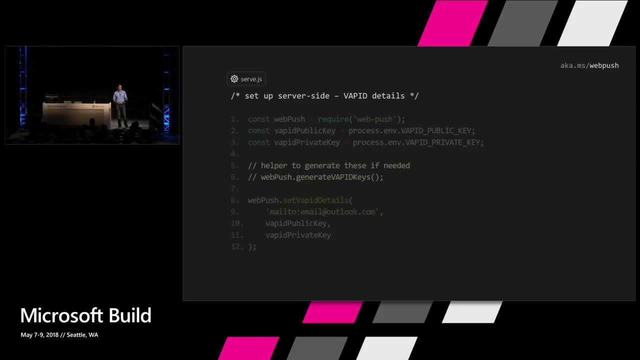 Global variables up at the top. You don't have to change them Once you've set them up. Then we're going to configure The web push, the web push library, by setting it up as a Vapid details. We're going to specify an e-mail. 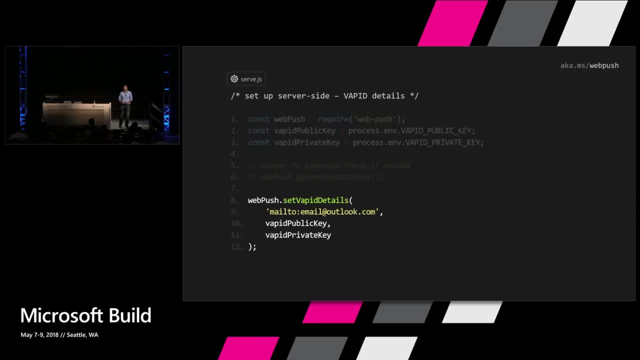 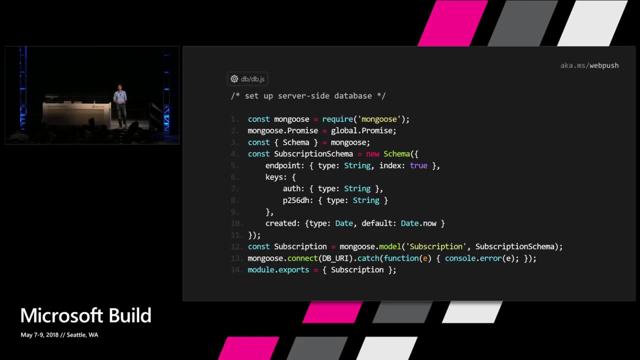 Address, and then we're going to specify the public and the Private key. So we're going to move on to the Database file to actually save those, to save the subscription data, And i'm not going to bore you with all the details of setting. 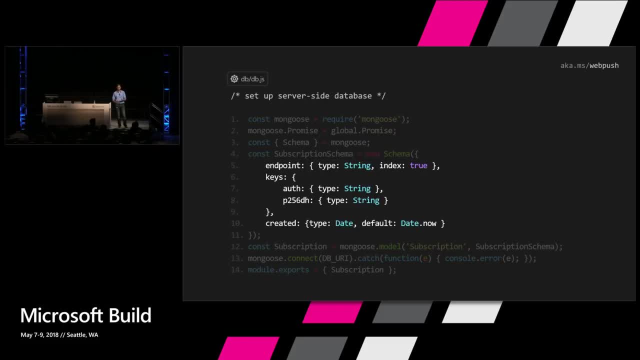 This up. We're just going to focus on the Schema, the data that we're actually interested in storing. What we're interested in storing is the end point url. So, again, the url that we're going to talk to from the push. 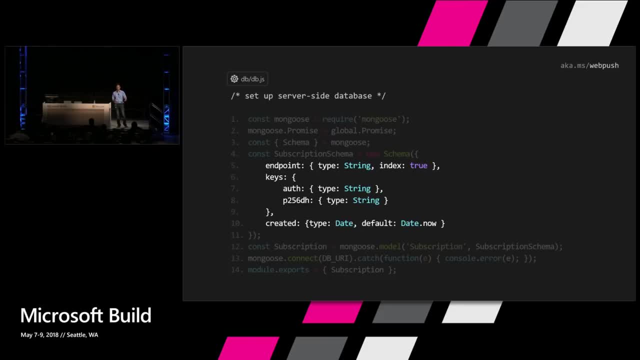 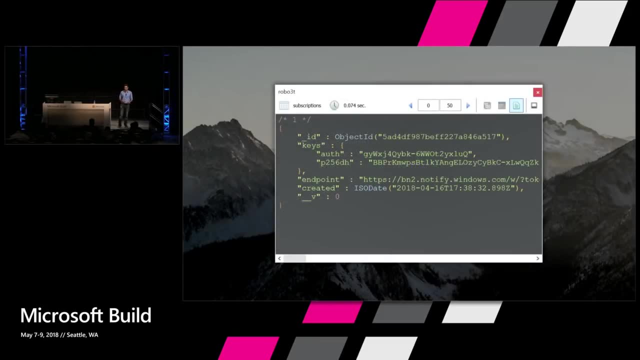 Services server so that we can get the data that we're Going to use, so that we can message the client And the keys, the encryption material that we're going to use. So this is what it would look like. I'm using here robo-mongo. 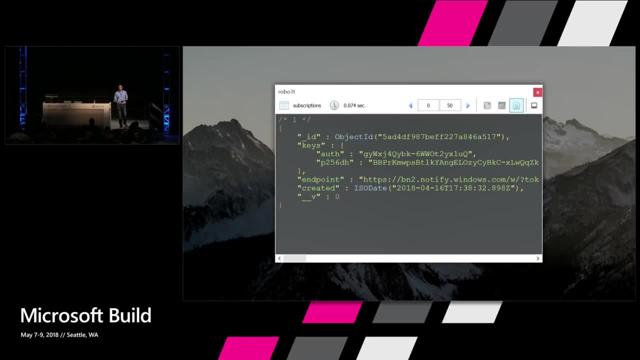 Which lets us introspect all the details of the database, And you can see it's json formatted exactly as the scheme I was showing. This is sort of how it would Look if you had an end point and the keys populated inside of a Database. So let's go through our. 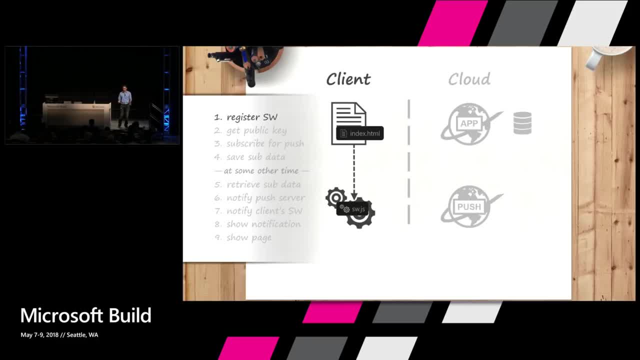 Workflow now that we've set up the database. So the first thing we're going to do is we're going to register The service worker. So that's from indexHtml. It's going to register service workerJs. First thing here. obviously we've done this before. 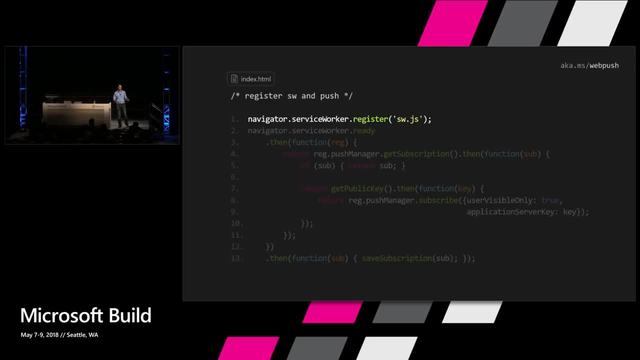 You guys remember what the key, magical thing is: NavigatorService workerRegister. And then we're going to use a special property on there, NavigatorService workerReady, which will tell us When the service worker has some of the data that we're going to. 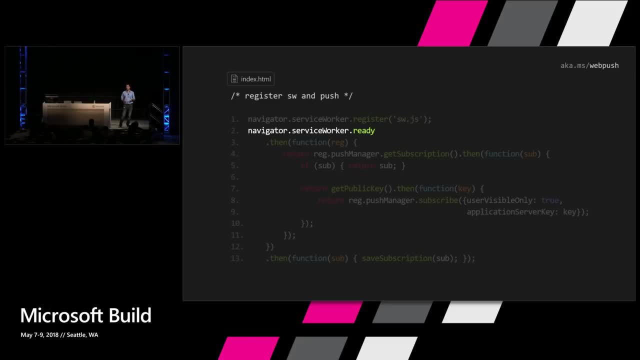 Use to set up the push. So when it's ready, we're going To, using the registration of the service worker, get its push Manager and then call get subscription to see if we Already have a subscription, Because if we do, we're just 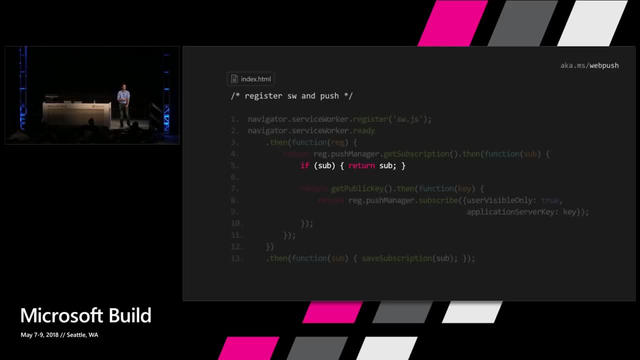 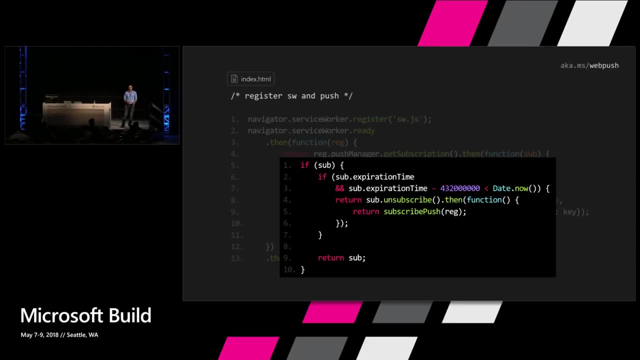 Going to give that subscription back and it's okay, We've already subscribed. In fact, you may want to have Something that's already in the database. You may want to have something a little more robust, because some Of these subscriptions can time out. They have, for instance, a 30-day time limit. In this example, what i'm doing is i'm saying in the last five Days of the subscription, i'm going to renew it by first Unsubscribing and then resubscribing. 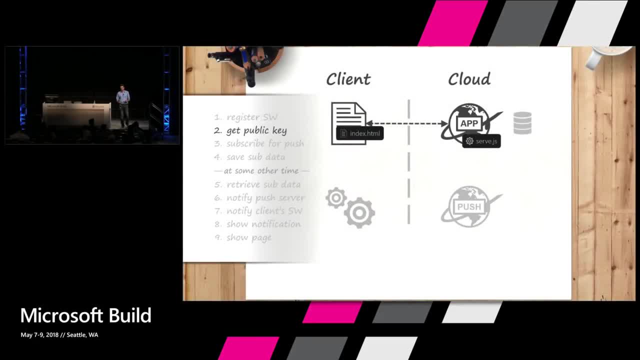 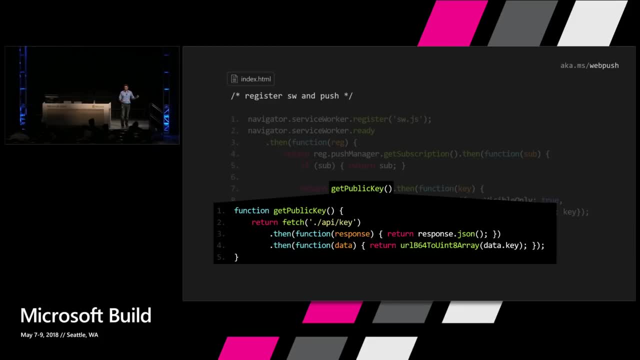 So we're going to get the public key as the second step To do that. we're going to go to the public key To do that. going back to our example here, we are going to Call get public key. So if we already have a 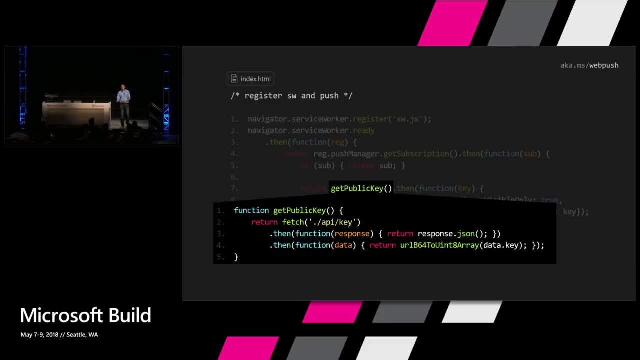 Subscription. we're going to return that, But if we don't, we're going to need to get the public key, And all get public key is doing is it's making a fetch to some Endpoint url. we specified Nothing magical there And then it will get the json from there. 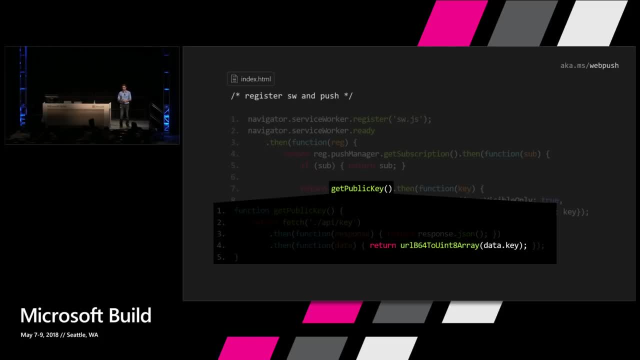 And then it will call this method: url: base 64 convert. For this you will need to do on chrome, you will need to do on Microsoft edge. The value you specify as part Of the application server key will need to be in this format: 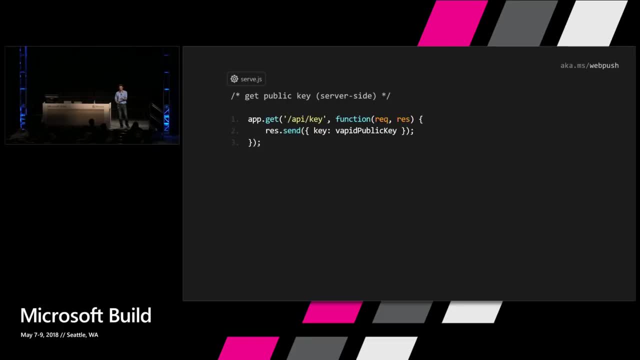 So from the server side, all you're doing is for specifying That api slash key. all you're doing is you're responding back With that vapid public key we set up as a global. That's it. So it's nothing complicated in That sense. So we're going to go back to the 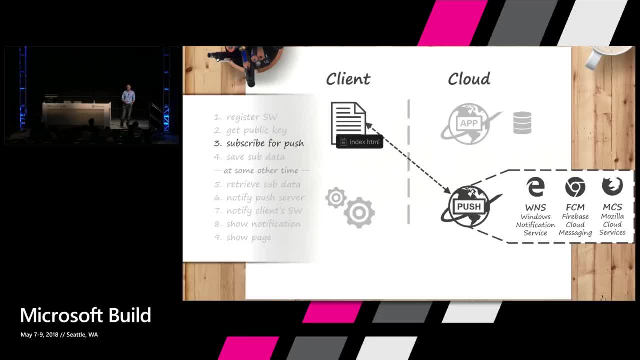 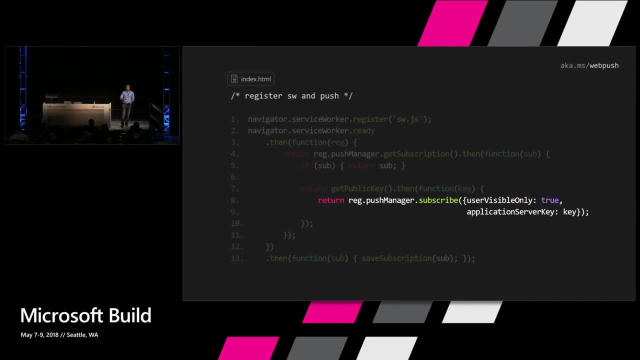 Website in that sense, And then we're going to Subscribe for push. So, again, this is going to Interface with different types of push subscription services, Depending on whether or not you know, depending if you're on Edge or firefox or chrome, And that will happen here. 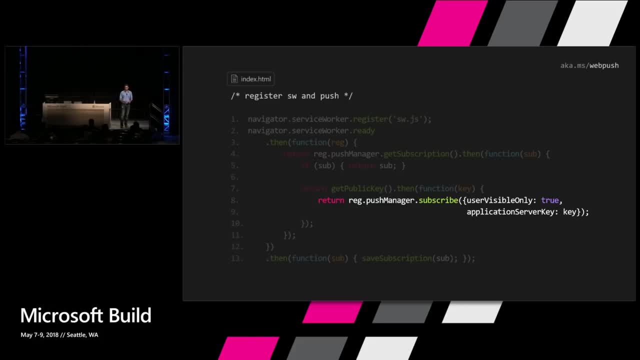 So we're going to do regPush managerSubscribe And we're going to specify user: visible only, true. And the application server key, the public key we just received, We're going to put that in there. So we're going to do that. 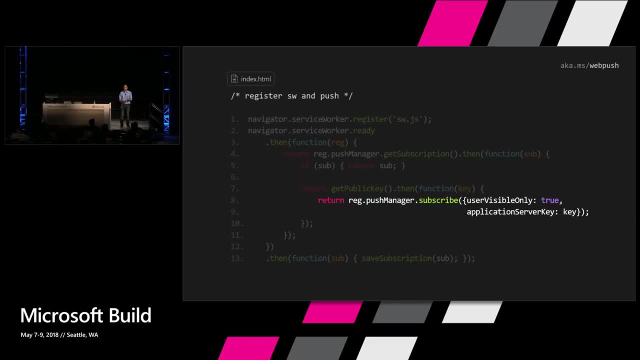 And it's important that we specify user visible only. true, Because it's creating a contract with the browser that we intend To show something when a push message arrives at the client. It could be the case that you may not want to show something. Like you know, you're getting push and then you want to do. 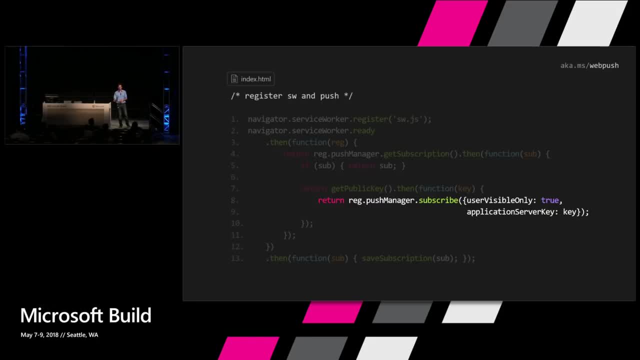 Something like bitcoin mining. Well, that wouldn't be possible If you specify this. In fact, we won't let you Register unless you specify true here. So you have to show: for every push that comes to the client, It has to show a notification. So we're going to do that. 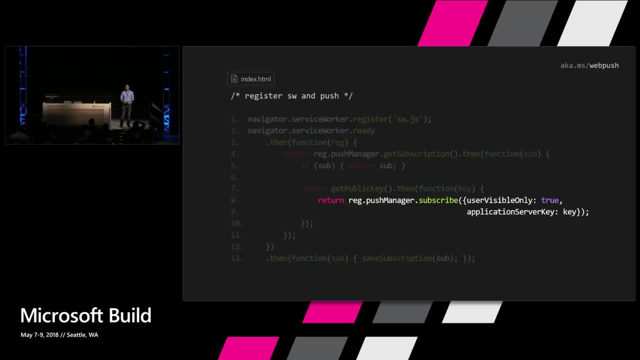 So that the user knows that something is potentially Happening in the background. I'm sorry if i killed any of Your hopes and dreams of bitcoin mining. Yeah, you have to set it to true On firefox. you can set it to false. 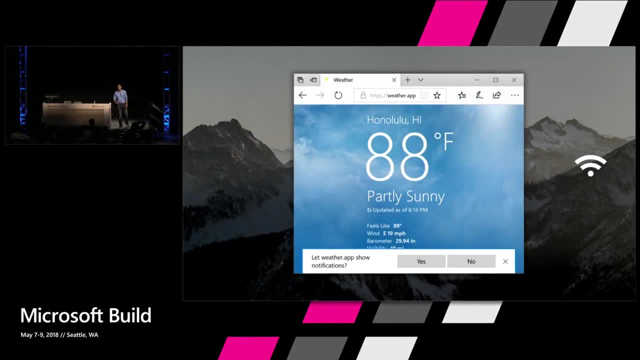 But that's another can of worms. So when you call subscribe, what Will happen? is you're going to get that prompt At this point? you're going to get that prompt for permission If it's not already granted. In this case, if the user says: 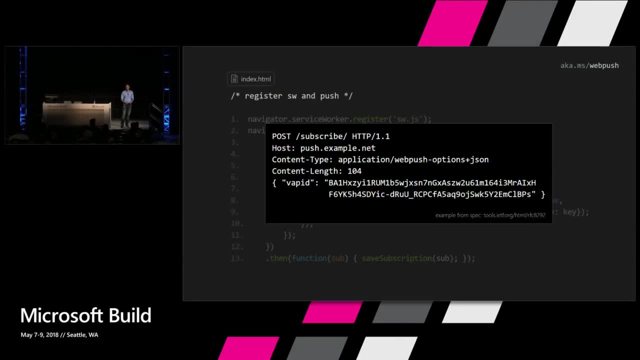 Yes, we will. then the browser or the engine, the platform That you're on, will issue a request. This is just a plain old http request, If you've ever seen one of these. it's very simple. It's just a post request to this end point. that will then give us. 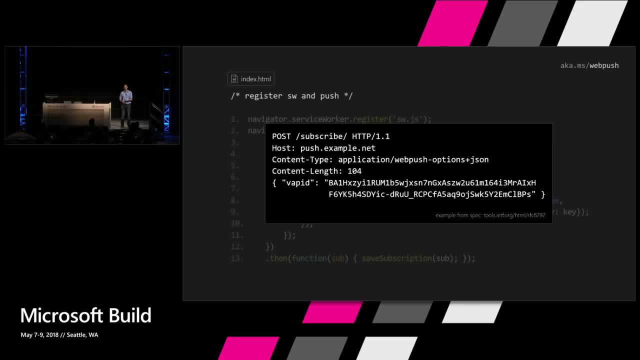 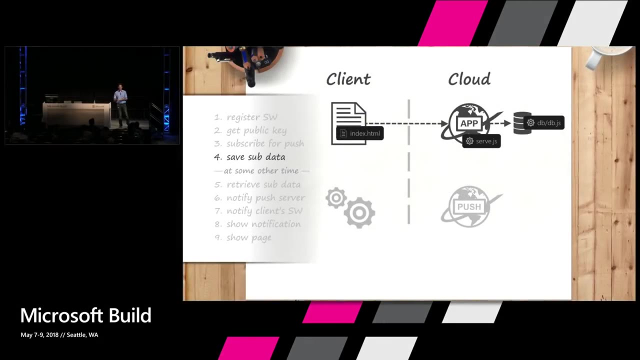 Back the information about the subscription that we can then use Again. trying to demystify this here for you, you're not going To see this happening in the browser, but this is what it's Basically doing. So at that point on our 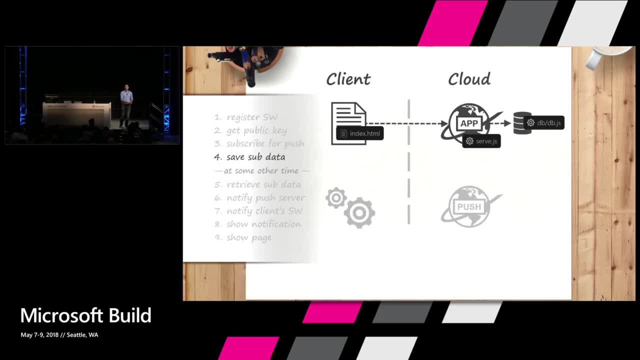 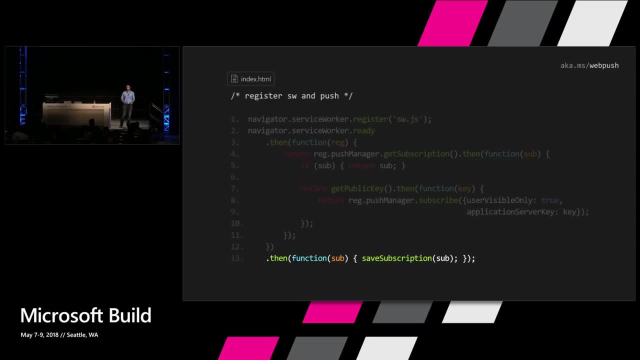 Application server. so the code we own, we're going to save the Subscription data. Okay, So again from that registration, the service Worker and the push, the last thing we're going to do is, once We have a subscription, we're going to go ahead and save that. 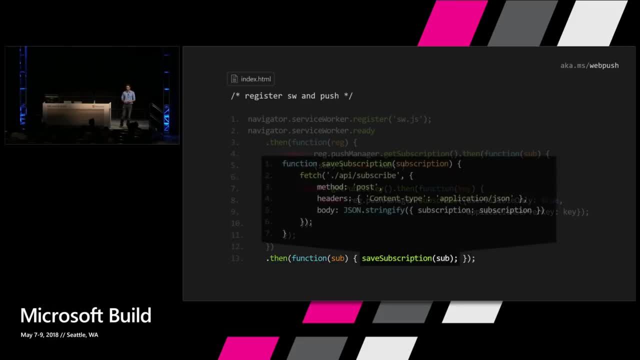 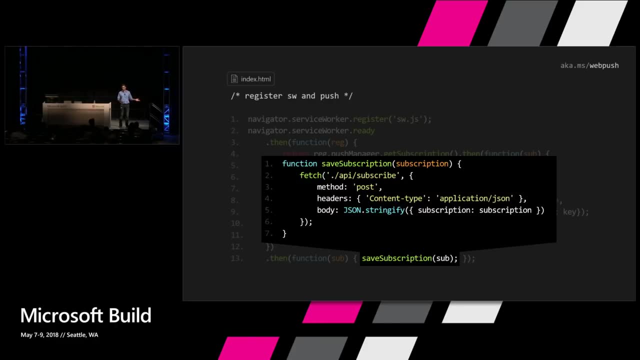 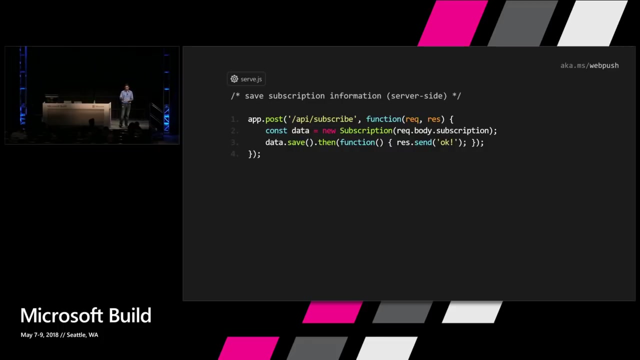 We're going to pass it up to the server And what save subscription is doing is just doing a fetch and Just telling the server: hey, here's the subscription data, Go ahead and save that inside the database And on the server side we're going to handle that. 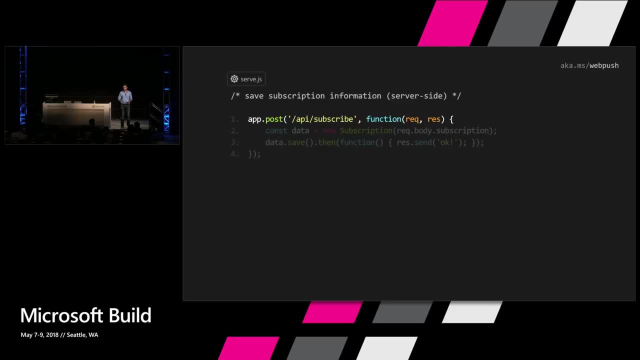 So what we're going to do is appPost and specify the api for Subscribe, which is going to save this data. We're just going to create a new subscription object that we're Going to project. Again, i don't want you to get. 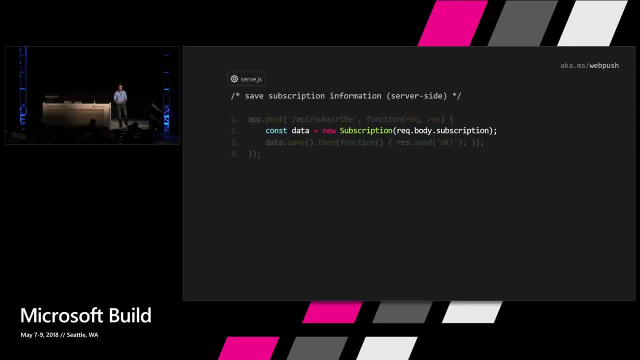 Bogged down with the details here. All it's really doing is just Saving it into our database So you can interpret this for any Different type of database you're using here, And then we're going to save that to the database And then we're going to tell the page that it succeeded. 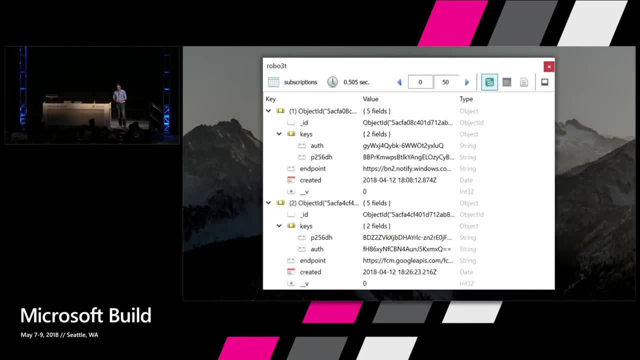 We're all good. So, using again robomongo to Introspect the database, we can see now that things are showing Up inside of our database And again we have the end point Url. here We have the keys, the. 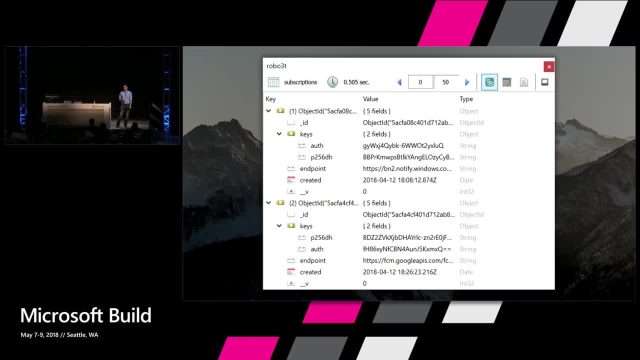 Encryption material. This is needed for sending Push updates for later, But really you don't really need To worry about exactly what these are doing. You just have to save them so that the web push library, when You pass it to it, can do the right thing when it needs to. 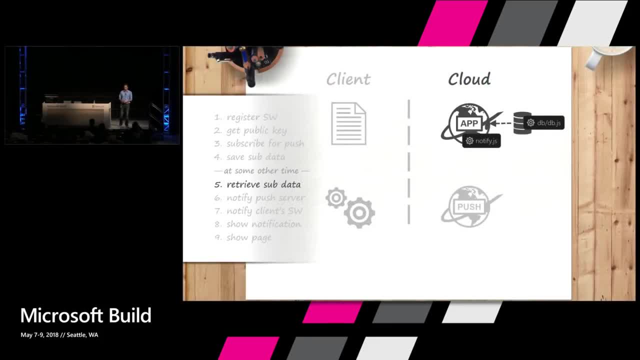 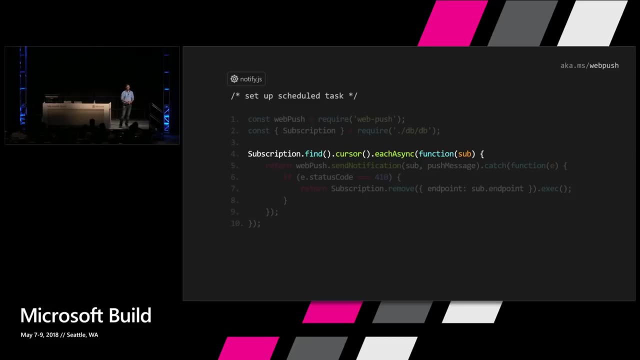 Send the push message. So here comes that other point In time where we're going to retrieve that data from the Database And to do that we're simply Going to just use a method that will enumerate all of the items In our database And, of course, at that point, 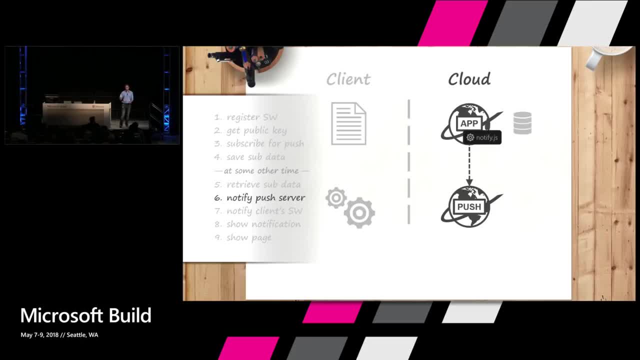 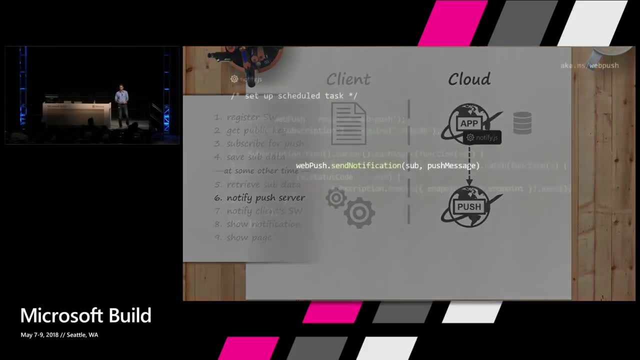 Once we've enumerated them, we've gotten it out of the Database. we want to notify the push services server that we Want to send a push message to the client. So to do that, we're going to call web push dot send Notification Again. this is a helpful way to 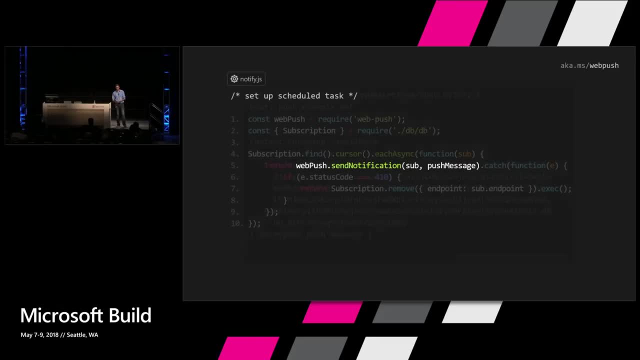 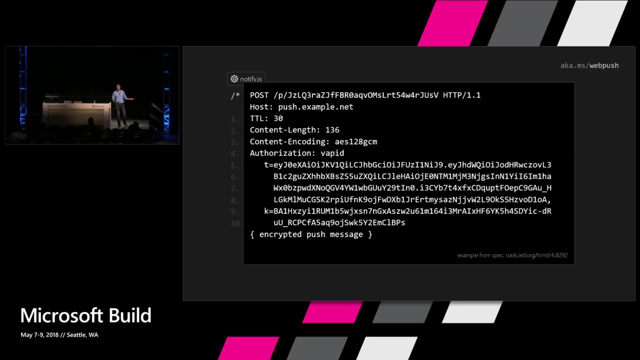 Use the helper method And i'm going to demystify this For you. It's kind of ugly, but this is What it does. It basically sends a request to The web push or to the push services server- again a Simple hdb request asking it to give us back details about. 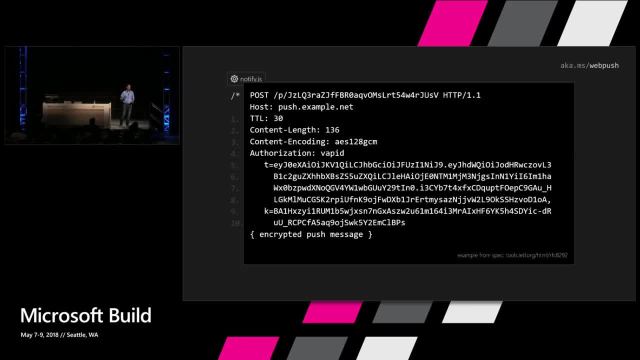 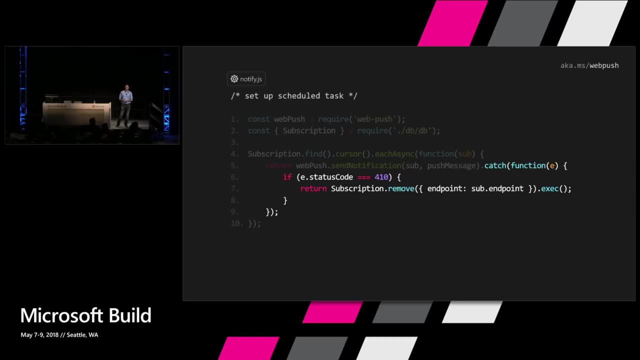 Whether or not the push was sent. But here it's just issuing a Request: Please send this data. And at the bottom it's the encrypted push message there that We want to send to the client. So if it fails, so if the server comes back to us with a 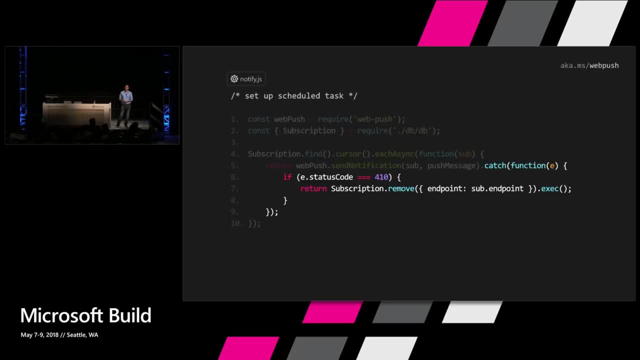 410,. what that means is the subscription is no longer valid. So maybe the person- the client, for instance- decided they no Longer want to receive pushes from you. In this case, you want to see that it got a 410, and you may. 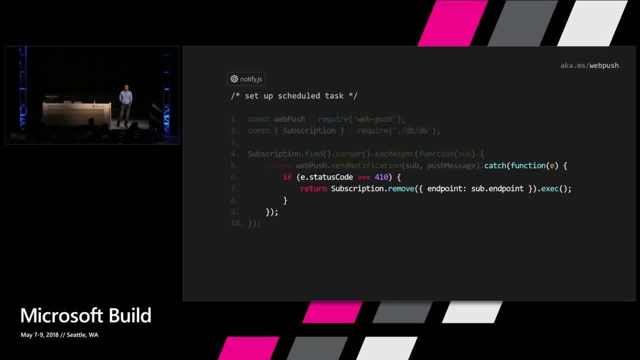 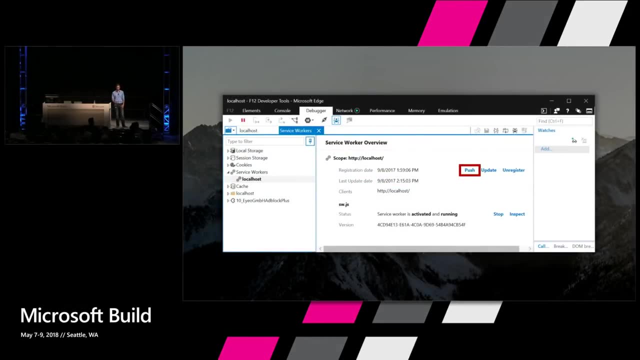 Want to actually remove it from your database so you don't keep Trying to push to it, because then it becomes wasteful. So here we're going to remove it from our database. In case you're interested, you can emulate the push event in a. 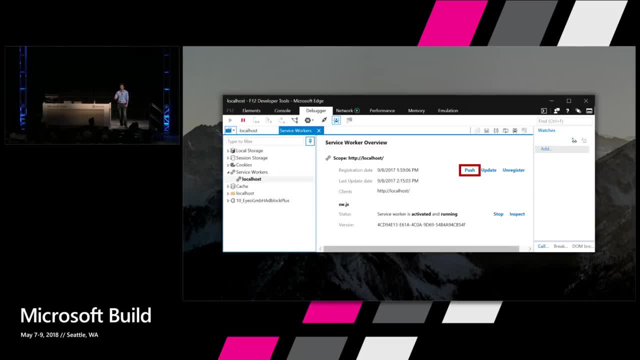 Service worker using f12.. So in that same panel that i Showed you before, where the service worker overview page Was, you can click push and it will send a push. It's just a faked out push message to your service worker So you can test out the push event handler in your service. 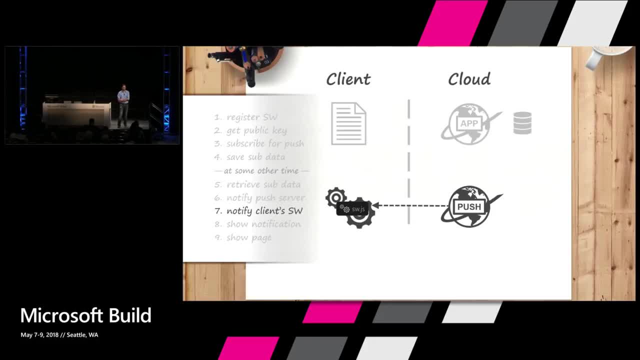 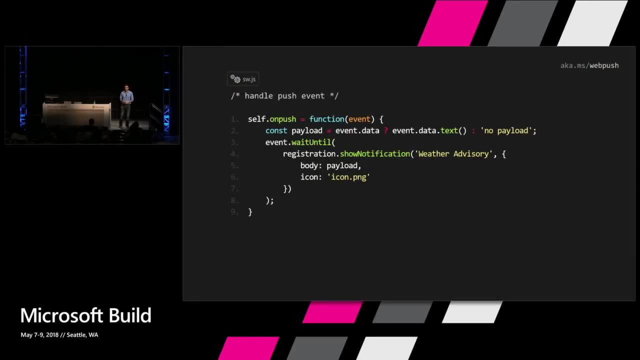 Worker, which is what we're going to be talking about now. So now we notify the client service worker, So here's another event that we're going to be talking about. Here's another event for the service worker on push. All right, We're going to get the payload. 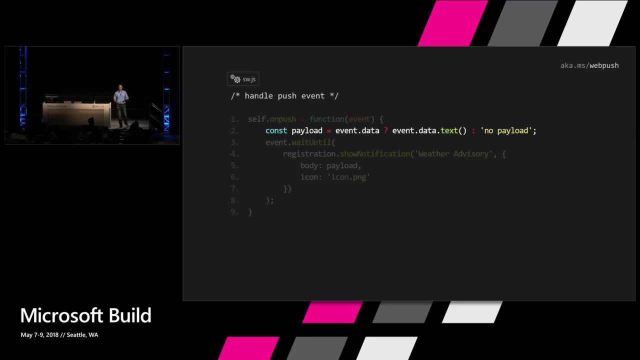 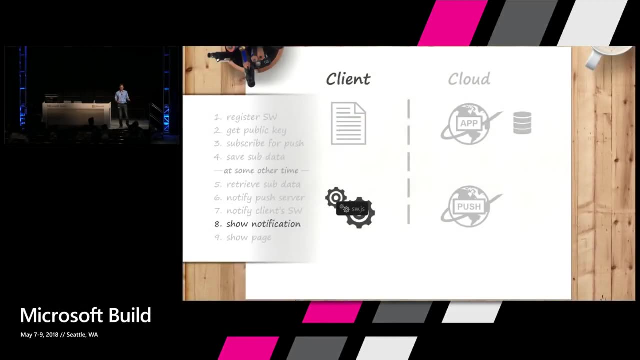 And we're going to grab out the text, the data, from that payload. So this is that encrypted message we got From here. we're going to wait until we show a notification. So how do we do that? we basically call RegistrationShow notification. 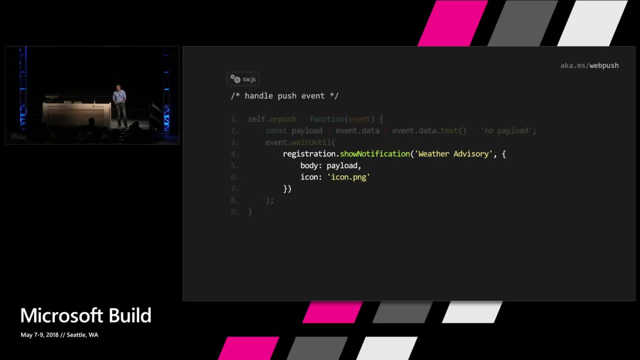 We're going to pass in a title and we're going to pass in a Payload, which is the message we got from the payload. So we're going to wait until we show a notification And we're going to give it an icon as well so it can show. 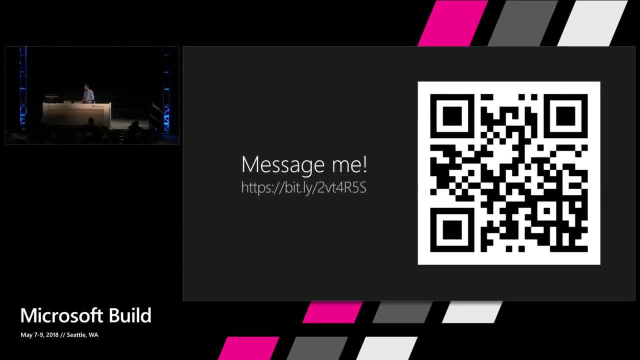 Something. So we're going to do a little Bit of an interactive demo here where you guys are going to send Me a push to my device If you guys want to either open That up or One second. I'm going to switch over to the 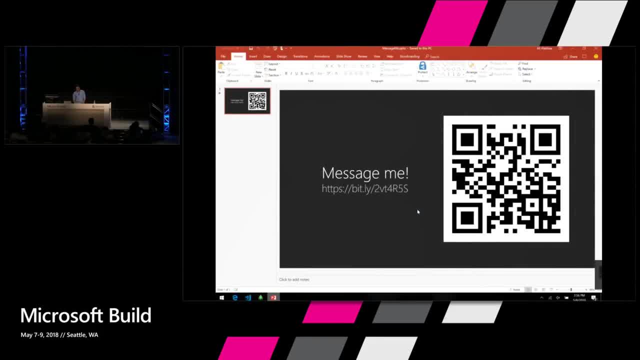 Other one. I'm going to keep it. So you guys are sending messages. Look at that, It's still piling up. All right, guys, keep it coming. So all this is really doing, by the way, is you're loading a. 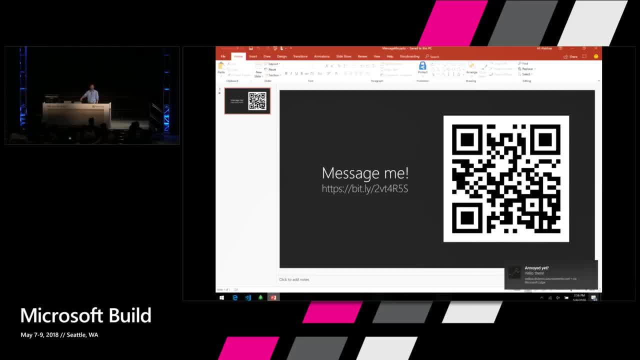 Page that is making a call to the server and it's telling it To send a push to the push services server. All right, so it completes that loop And then it comes back to my client here. Wow, holy cow guys 21.. 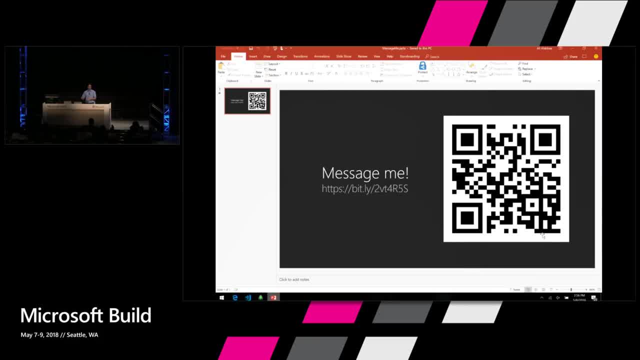 Okay, So that means that we're Now able to on the client device we're getting. Yes, i'm annoyed, Thank you. So that's what i'm about to show you Very, very nice. So what i can do here is because 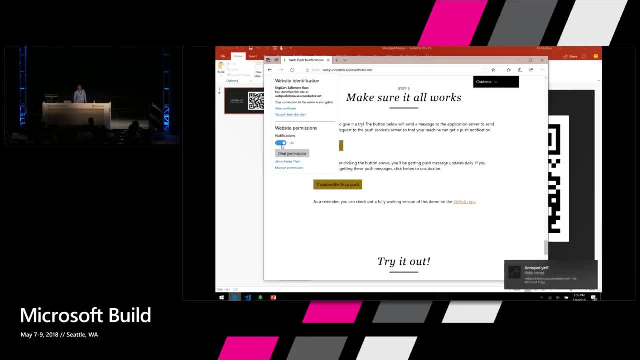 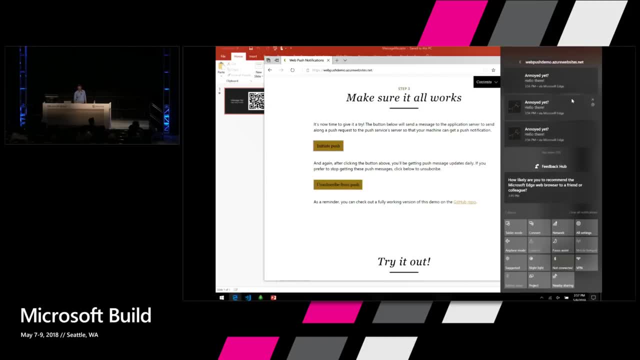 You guys come on, I can turn it off or i can Clear the permission and then i effectively disable you guys From sending me more pushes. But you can see here, these are All the pushes. They all got stacked here into My device, All right. 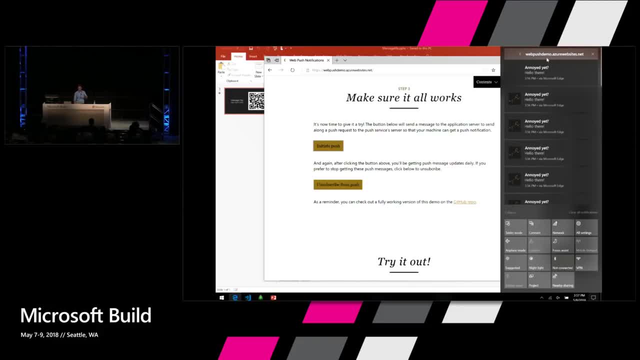 This is my action center And they all get grouped under That same domain. So we've tried really hard here To integrate with the action center. so it feels more like a Native application. So i'm going to close this and Show you what it looks like when you actually click it, because 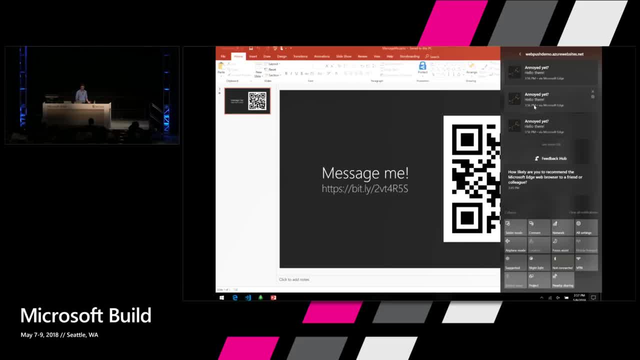 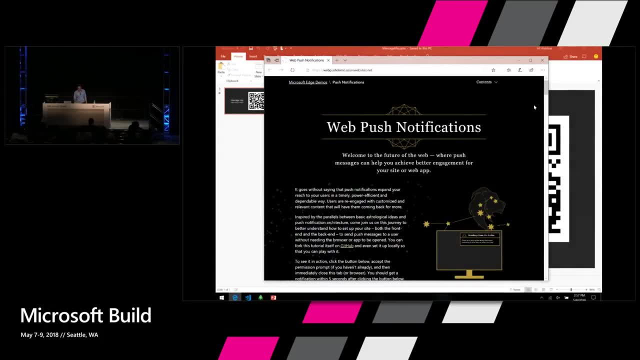 That's what we're going to talk about next. So i'm going to click on this and what it's going to do, Because you can tell that edge is not open down there. it's Going to open edge and it's going to navigate me back to. 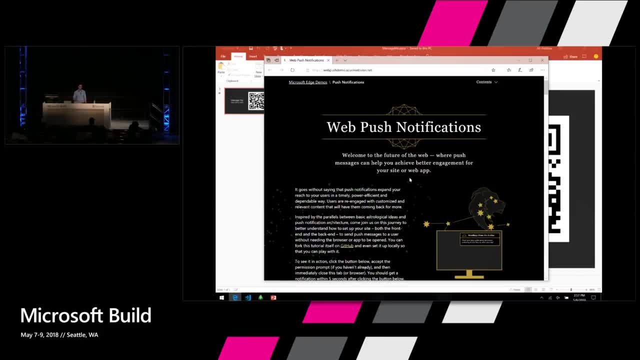 The demo. So this is a good way You can specify where you want it to go, but this is a good way To repatriate your users back to the page that you intended them To go to. So Thanks, guys. So now we're going to show the 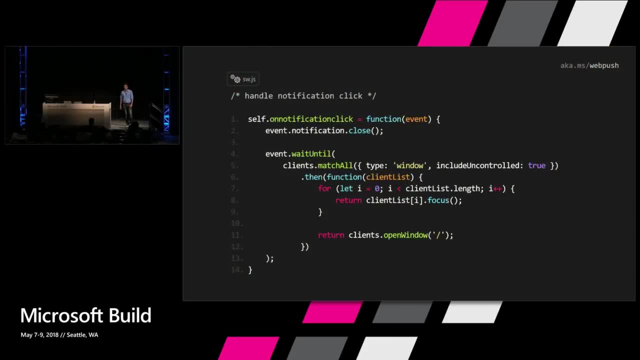 Page and you just saw how that worked. I'm going to show you how to do it. So we're going to handle the notification click event. What we're doing here is we're saying So on notification click and then we're going to first close. 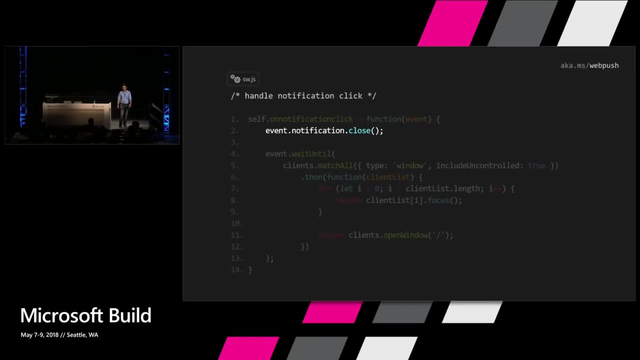 The notification. So we're going to tell it to Tell the notification to go away, And then we're going to use ClientsMatch all and we're only interested in the clients That are windows, because you can have other clients, like Iframes for instance, and we don't care if they're controlled. 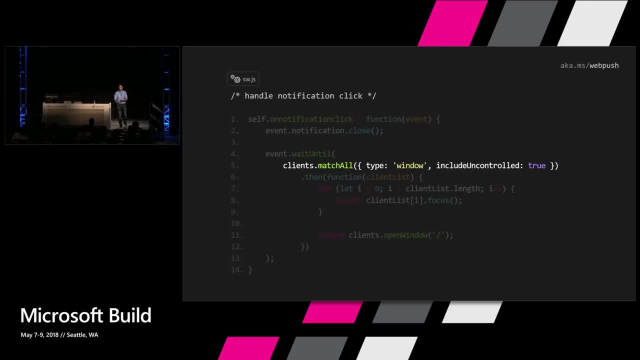 By the service worker. Remember, controlled means that It's servicing its requests. We want all of the service Workersers, or, sorry, all the clients that are under the same Domain as the service worker. In this way, we're going to tell. 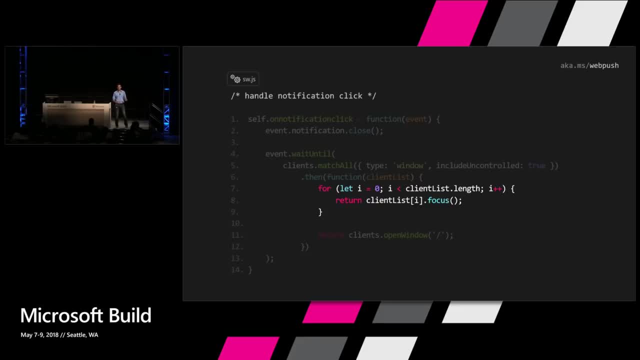 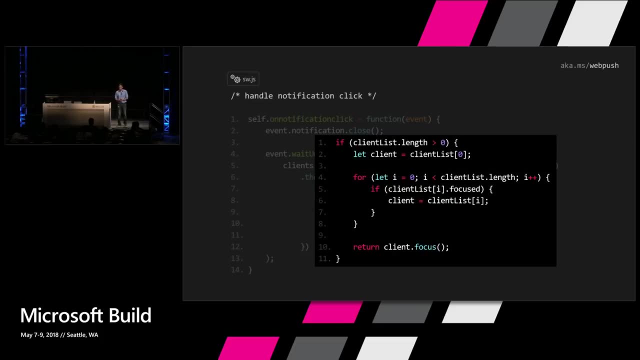 It to go away. In this way, we can then Enumerate through them and choose a client, if one exists. To focus on A more robust implementation, Might actually check for those clients and see if there's not Just the first one, but see which one would be a better. 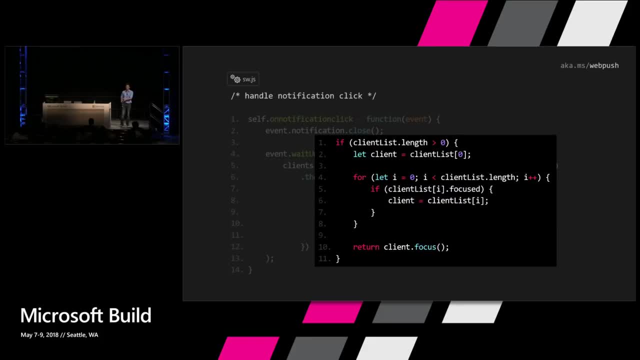 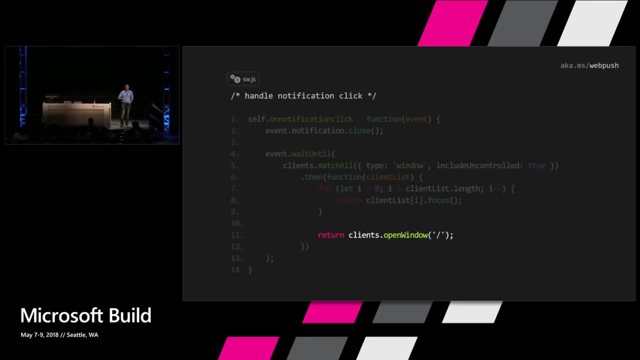 Match Again. these examples are part Of that web push tutorial demo, so if you wanted to get more Context on that, i advise you to go check it out. It's on the top right corner of that slide And then If we don't have any clients, so if none of those are open in 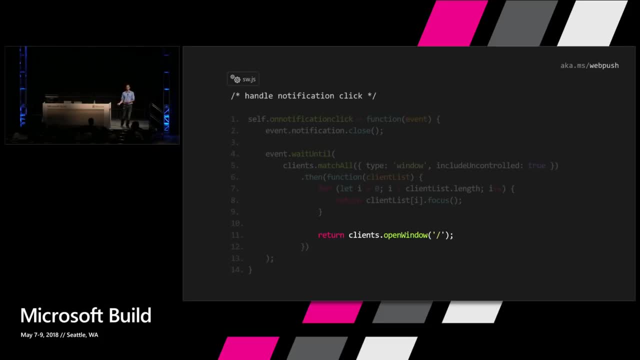 The case that i just showed you, we're going to open a window so That we have something that will actually be shown. So here we're just doing clientsOpen window and we're Specifying a place for it to go to, And so here we go back to our app or whatever it may be. 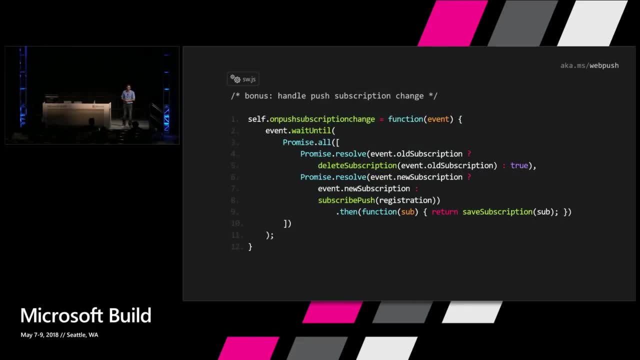 So, as a bonus, although on push subscription, change is not Implemented by the various browsers, we are looking to Implement this, especially considering the fact that we Have that 30-day period where it will get expired. So, if you like, you can implement this method to future. 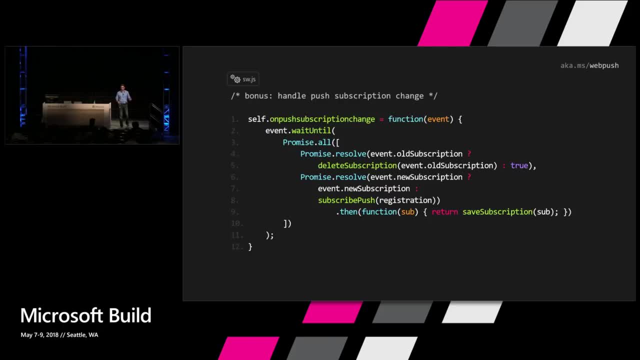 Proof you. Here's what you might want to do Here. So listen for the on push Subscription change event. This is when, for instance, You're at the end of that 30-day period and we attempt to Resubscribe you. We're going to wait until both. 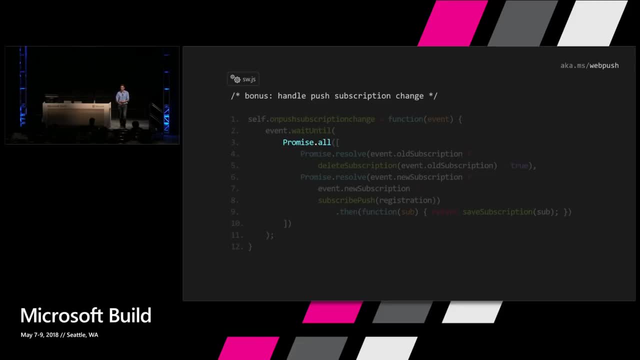 Of these promises are finished, I'm going to go through the First promise first. The first promise checks if the Old subscription is still available. So we're going to wait until both of these promises are Finished. I'm going to go through the First promise If the old subscription is. 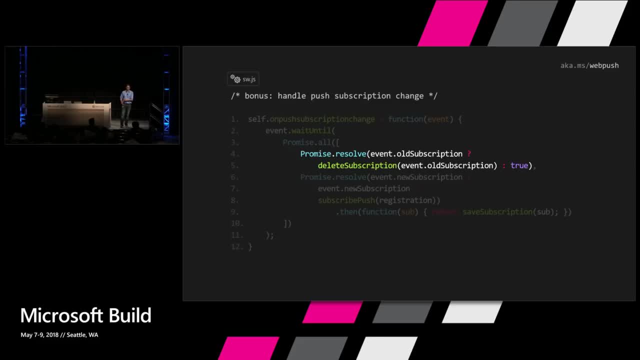 Specified and, if it is, let the server know to delete it. Otherwise, just resolve the promise and it's fine. The second promise: if a new subscription is specified, just Resolve it with that, Otherwise we're going to just. 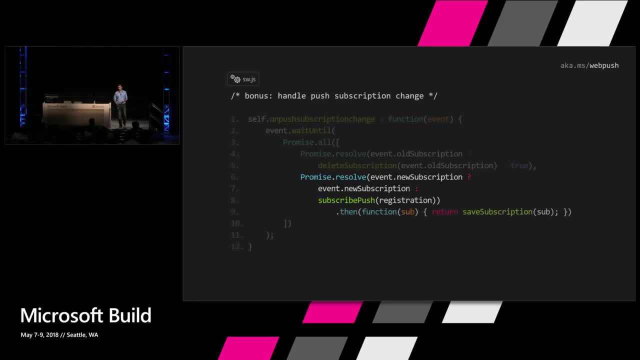 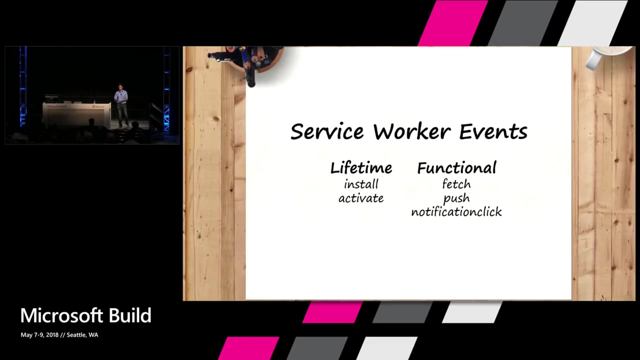 Subscribe for a new push, And that's that part, And we're then going to need to tell the server the new subscription Info so we can save it. So so far we've talked about The different lifetime events and these new functional events. 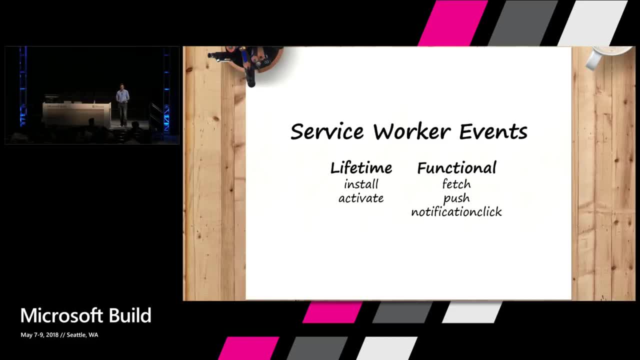 Like push and notification click. But again, a service worker Can do way more than this And we can expand on the Possibilities here. You may have heard of something Called background sync or periodic sync, for instance, Where, for instance, let's say, you had a news application or